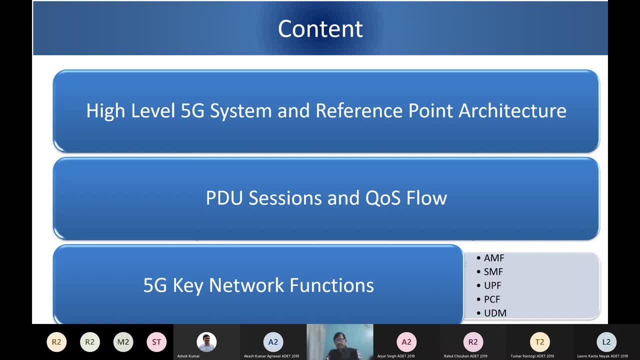 network functions of 5G, like a AMF. AMF is access and mobility function, Then we'll talk about SMF, which is session management function, and then we have UPF, user plane function, then PCF, policy control function, and then we have 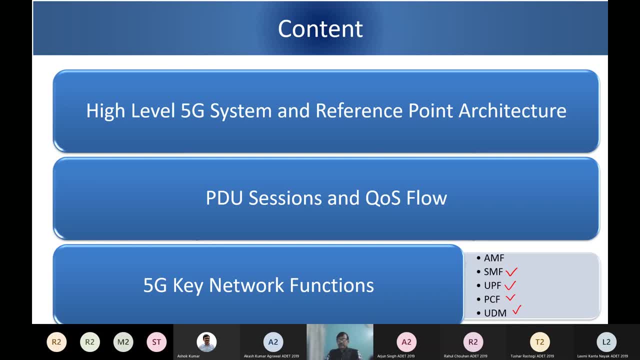 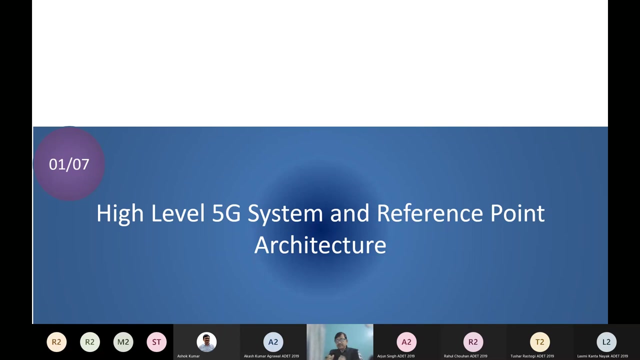 UDM- unified data management. We will also compare these with our 4G architecture so that you are able to correlate. You have gone through 4G architecture and other aspects you will be able to correlate, and also, as someone was telling that some part in 4G is left. so, wherever possible, I 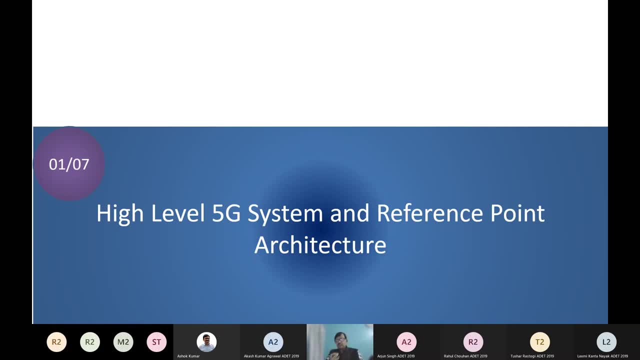 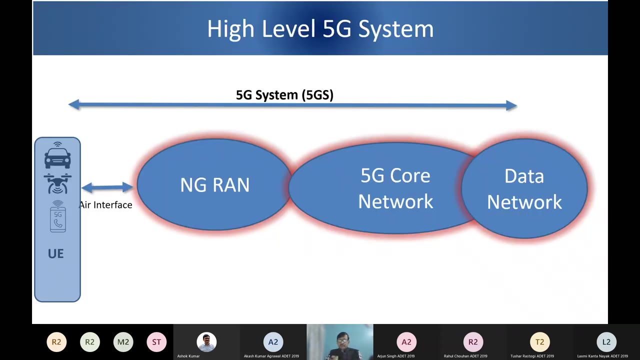 will try to compare with 4G and also cover the 4G part wherever you feel that was not covered. So let us start from a high level 5G system and then we will talk about SMF. We will look at reference point architecture. So this picture is a high level 5G system. 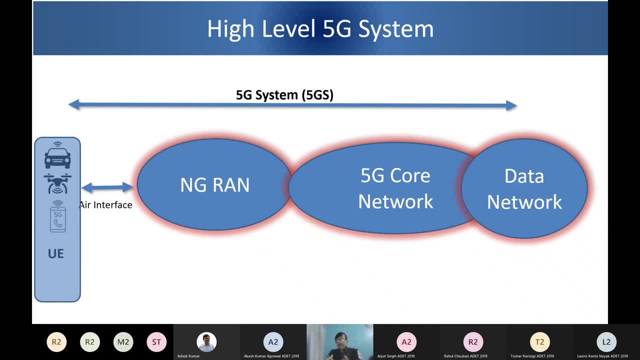 and this is similar to 4G, 3G or 2G that you have user equipment. In case of 5G, user equipment can be mobile, can be any object, can be machine, So it can be a drone, it can be a car or it. 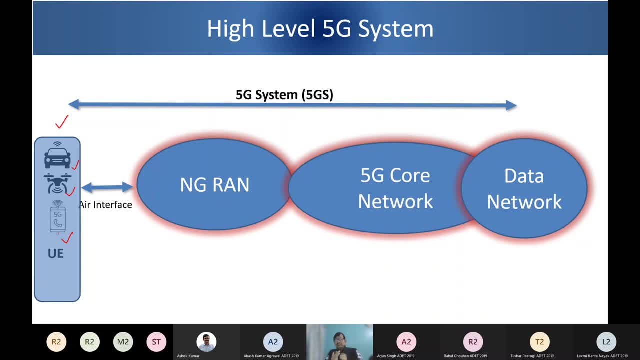 can be any object or device. So that is the difference from earlier generation of the network, wherein prime focus earlier was only with the mobile phone, whereas 5G will support not only phone, which we use, but also it will connect any kind of object and equipment. Then we have RAN part. 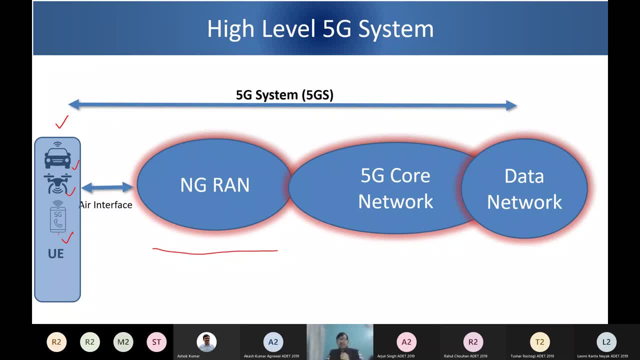 Radio access network. Here we call it ZNB. In 4G the name given was: can somebody tell me what was the name in 4G? ZNB, ZNB, ZNB, ZNB, ZNB, ZNB. 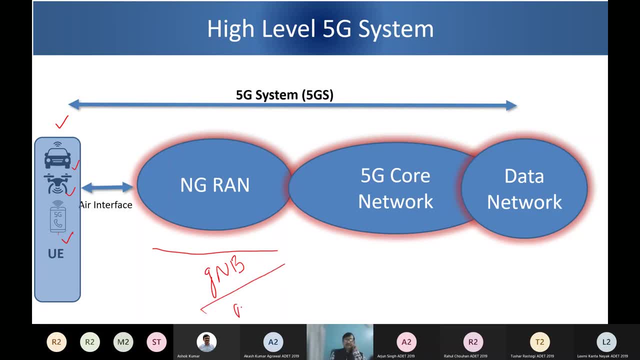 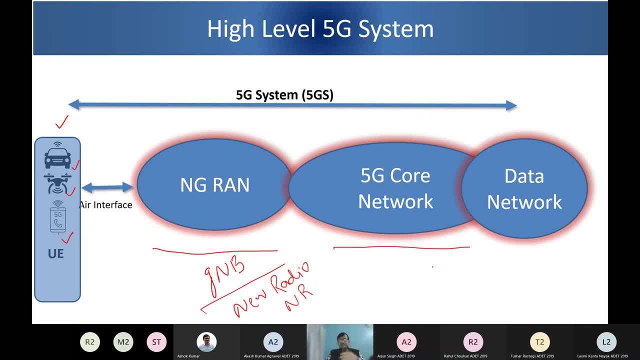 Which may consist of multiple network functions like AMF, SMF, PCF and so on. So we have a core network, Then we have a data network. Do you remember what we used to call this in 4G? What was the name? it is a data cluster. 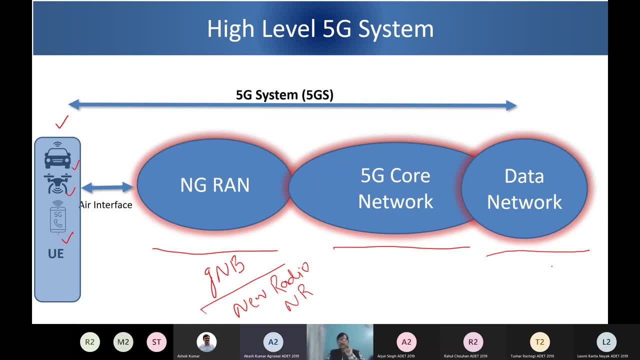 what was the name given in 4g epc? evolved packet core. evolved packet core, or we used to call it evolved packet core, was name of the entire core. i am just talking about the data network part. what was the name given? do you remember, do you recall, pdn? 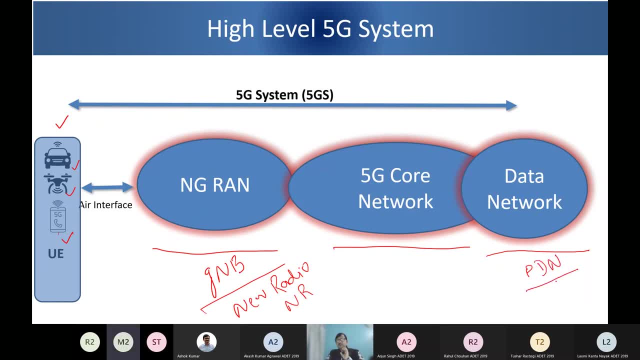 so it was a pdn right data network. it was a data network, but in 5g we are calling data network. can you guess what is the difference? can you guess why we are calling data network and not calling a packet data network? maybe it's one of the key difference from 4g. 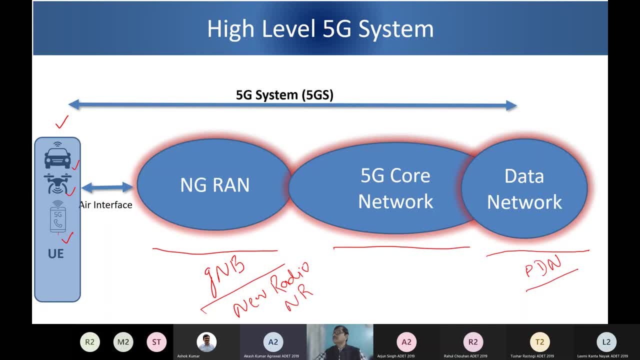 ims systems and those things are also there. maybe because of that, that was also there in 4g, that was also there in 4g. so difference is that 5g not only supports ip type of traffic. so when we say packet data network, we actually mean the ip type of a traffic right. but when 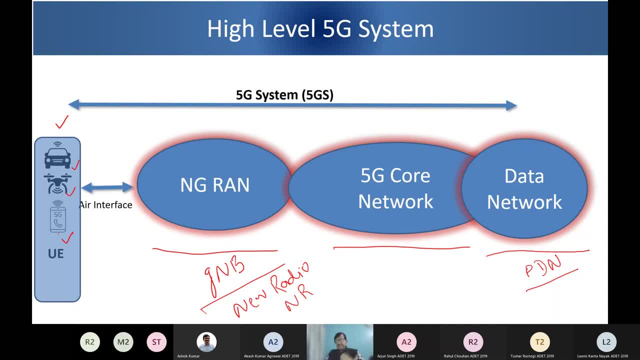 When we say the pure data network, it can be any other kind of data network which is not a IP data network, right? So that means IG also support some kind of structured data, right? In addition to the packet data? Like what, sir? 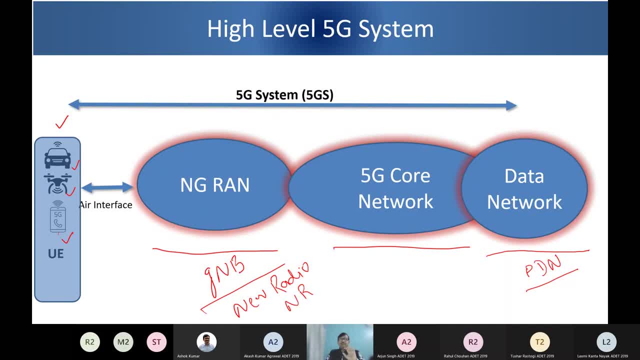 So, for example: so normally in IP data you have a lot of overhead header and all right. But suppose you want to serve IoT devices where you want to use very, very small bandwidth. So IP traffic is not suitable because a lot of overhead is there in the IP. 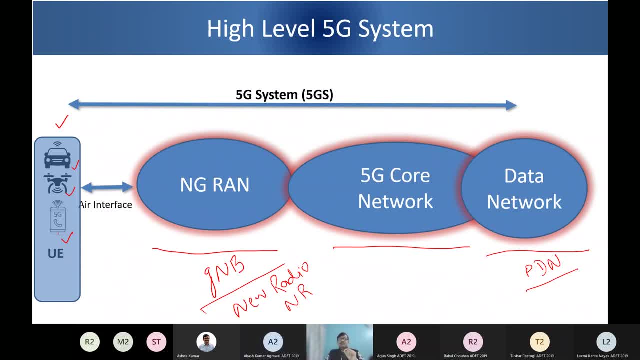 So there we use structured data just like our signaling messages, right? So that's why we call it a data network. So any kind of data network it supports it can be, of course, IMS or any service, any application function. 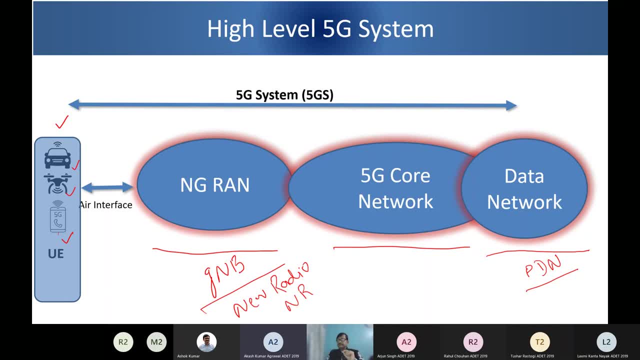 Right, And also, is there any standard related to that, sir? Yeah, yeah, yeah. So yes, that is there, for I mean, the 5G defines that what kind of structured data it will be supporting. Okay, so now, end-to-end system is called 5GS. 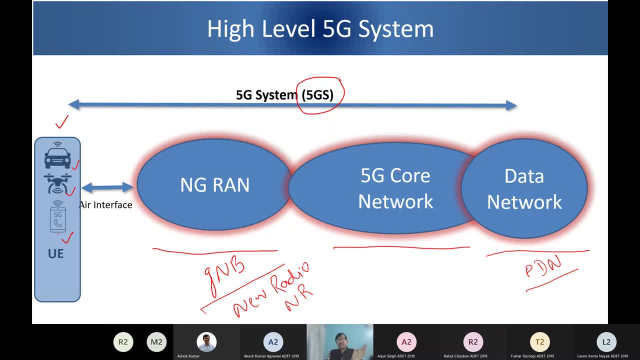 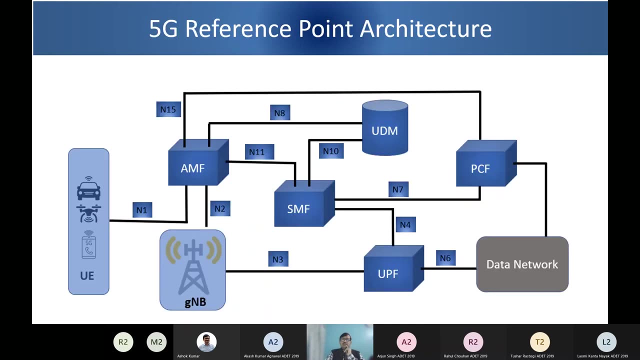 So when we say 5GS, we mean the complete network, from UE to NGC, To NG, RAN, to 5G core network and the data network. So that is our 5G system. Okay, so let's move forward. 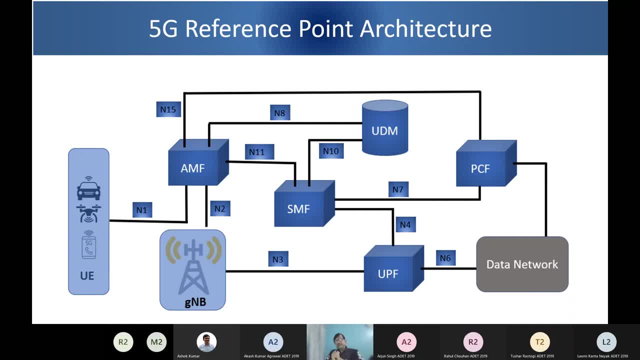 So I was talking about two kind of architecture which 5G has, in the sense that if you look at 3GPP specification, I would request that I had shared the 3GPP specification related to the architecture. At least you should scan through, right. 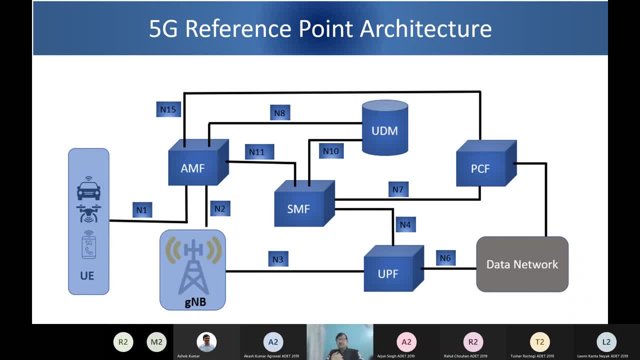 So you will see that every diagram is made twice, One in reference point architecture and one in service based architecture, So in a reference point architecture. why it is called reference point architecture? Because each network functions are connected to each other on a specific reference. 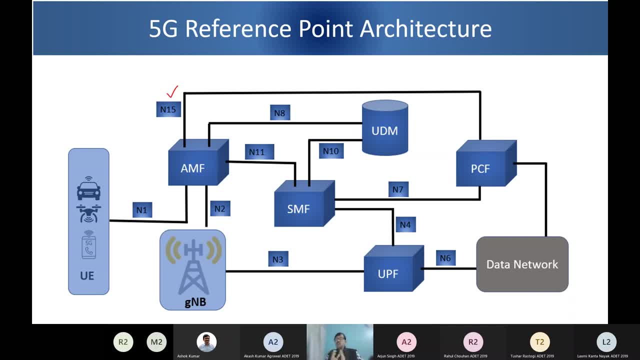 So they follow a specific protocol between the two right. So, and these are numbered like N15, N8.. In practice, the service based architecture will be deployed, But to understand the functionality, what kind of communication they make with each other? these reference points are discussed throughout the 3GPP documentation. 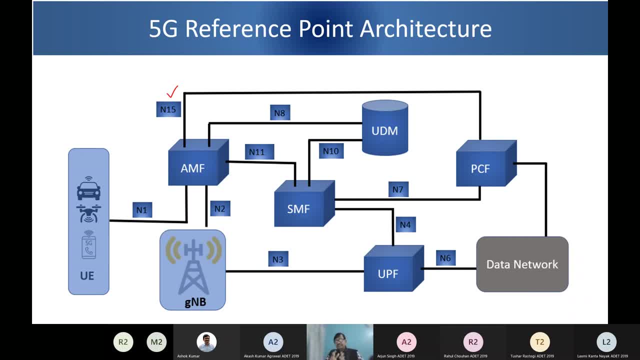 So we will start with reference point architecture and understand how these network functions are interacting with each other. In this picture I have only 3GPP documentation, So we will start with reference point architecture and understand how these network functions are interacting with each other. 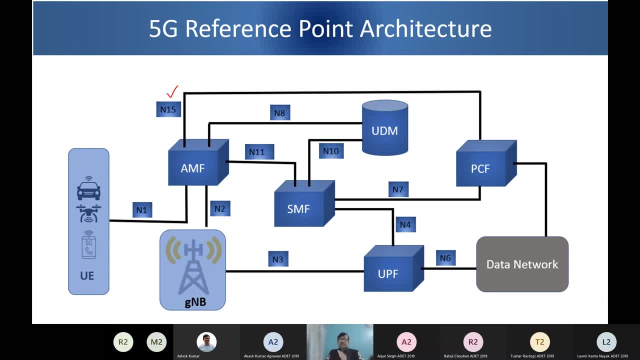 So we have taken 5 core network functions, That is, EMF access and mobility function, SMF session management function, UDM- unified data management, PCF policy control function and UPF user plan functions. And then we have taken the other aspects. 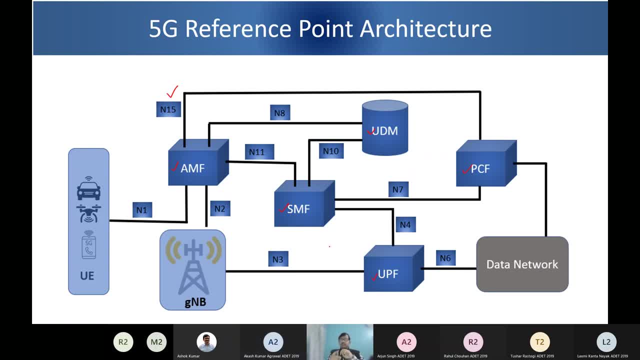 So these 5 network functions will be: Yeah, please go ahead, Sir. this. N8, N11, N10.. Are these subnetwork functions? Are these some transport protocol? These are kind of a point to point protocols, right. 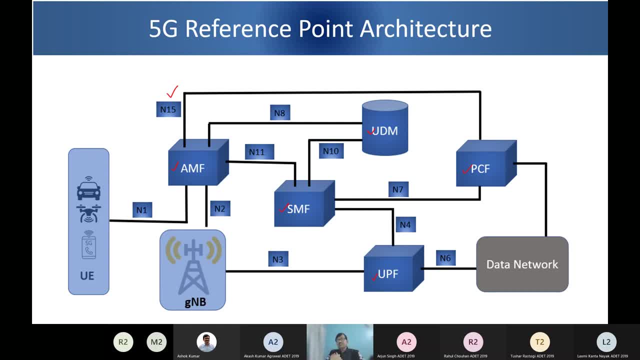 You can say that point to point. how they will talk to each other. Those protocols are defined right, But they will be communicating through fiber optic network. Can be any any type of network, So it because these are core network function, So they will be deployed. 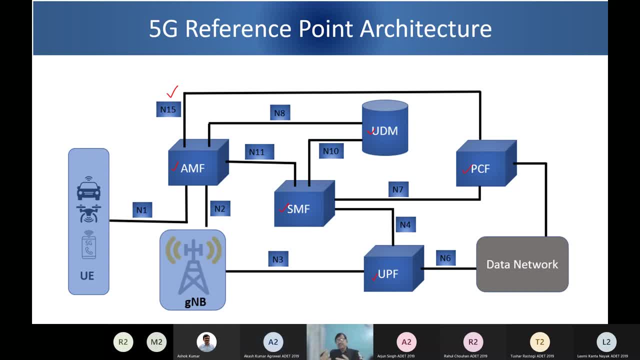 Okay, At the same location mostly, or it can be also deployed in a distributed way so that they in, as I am saying, in practice they will be deployed based on a service based architecture. That means they are connected on some kind of a network, right? 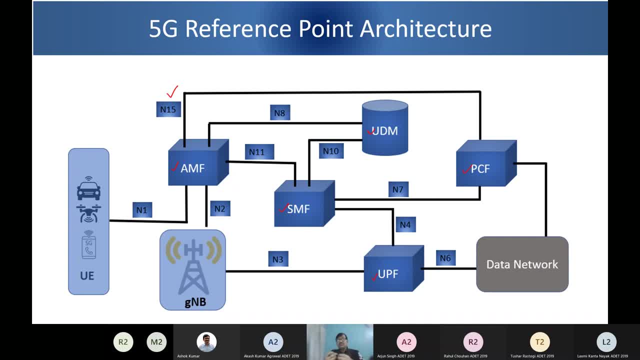 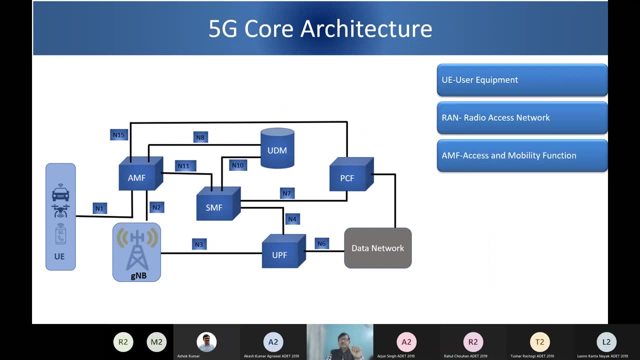 Some kind of a network. So underlying transport can be even radio, can be fiber, can be cable, can be anything, Doesn't really matter, Okay, Okay, So. so name we have understood. now Let us go one by one. 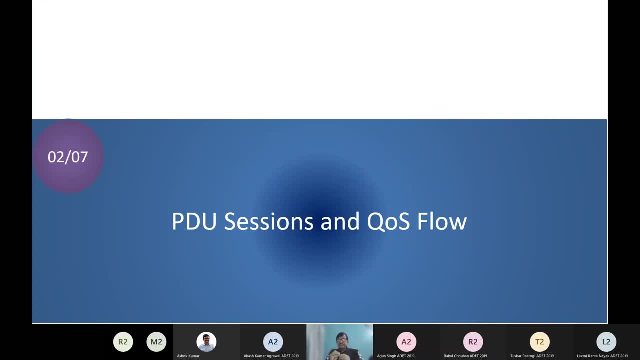 So first of all, before I look into each network functions, let us understand what these protocol data unit sessions and, and then what is quality of service flow. in a very brief, I have a separate session on QoS, So there is a separate session on QoS. 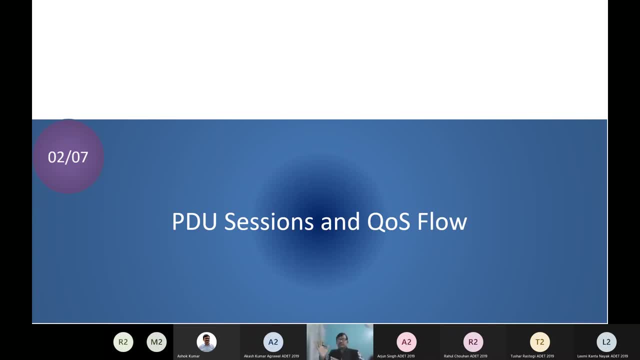 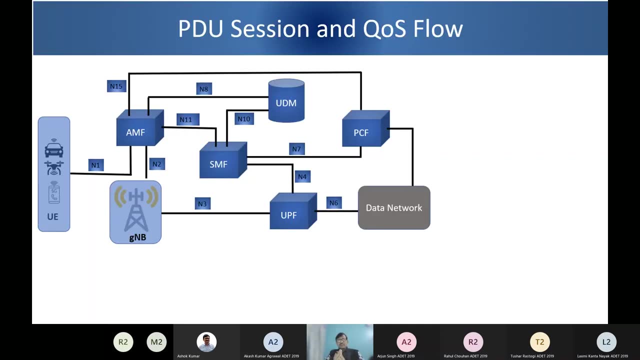 Okay, So there will go in detail, but before we talk about every network function, this is important, So let me ask you that the data flow, the user traffic data flow, will be handled by which all network functions. can some of you guess and tell me? 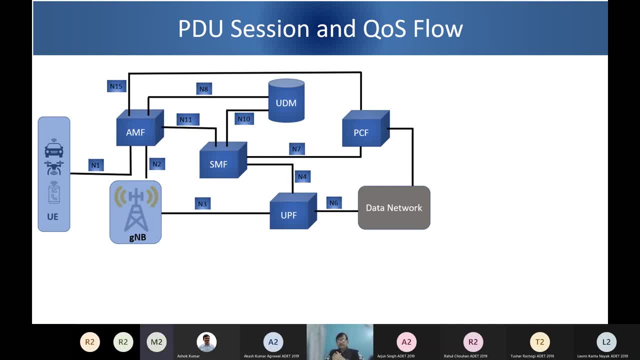 UDM. Okay, Okay, Okay. Am I Any one else? So PCF also apply that? I'm talking about just a flow of user traffic. How? because suppose uploading some data So it will go to which all network functions I'm talking about. 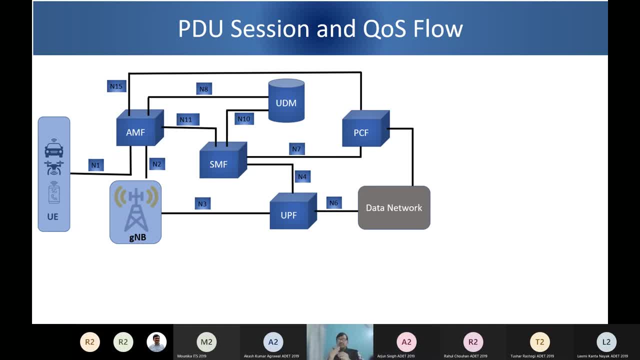 Just your user data right. Where suppose, uh, uh, UPV is uploading a picture right Of the data, is uploading a picture or a movie, right so which all network function will be used for that traffic? i'm not talking about the control signaling part, so leave apart control signaling. just look at the. 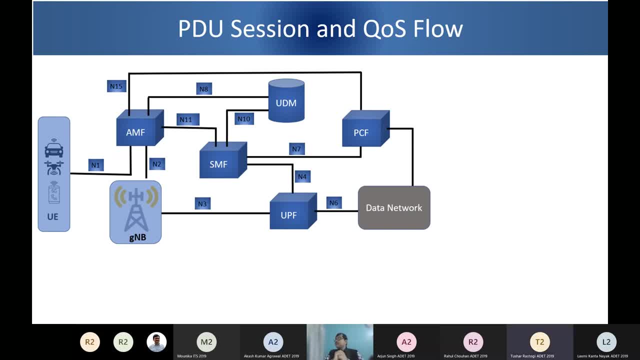 user data where it will flow, sir, your upf. it will take from gnb and then upf will come. sir, user plate function. yes, tussar is right. anybody else want to answer this? sorry, amf, also ml. okay, any other guess by anybody else? okay, so tussar was right. so if i just see, i segregate this. so this is your. 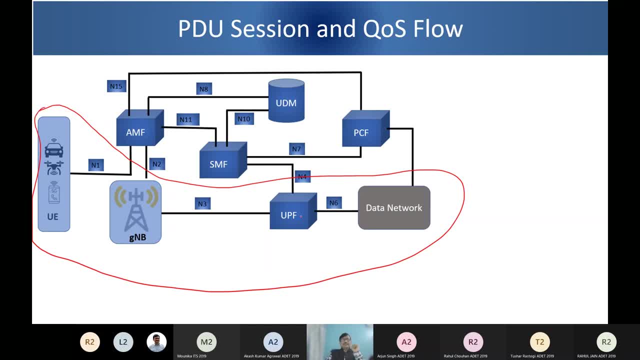 kind of a user plane. your user data flows from uv to z, node b to upf and to a data network. if you are accessing, say, internet, so it will be a internet data network. if we are accessing wise, it will be ims. if you are accessing something else, then that. 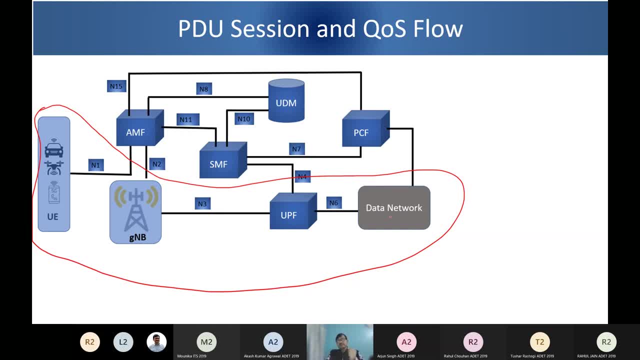 data network if your enterprise customers, your enterprise data, it will be accessing. so this is your user plane. so we call this as a user plane because actual user traffic flows through these network functions. is this clear to all? of you say yes or no. or in the chat box, you say yes or no. yes sir, yes sir. will it not go through amf? 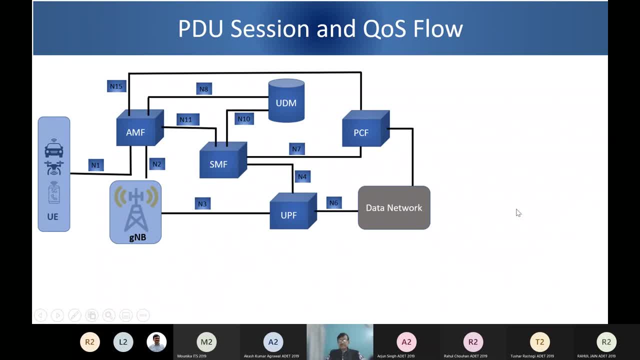 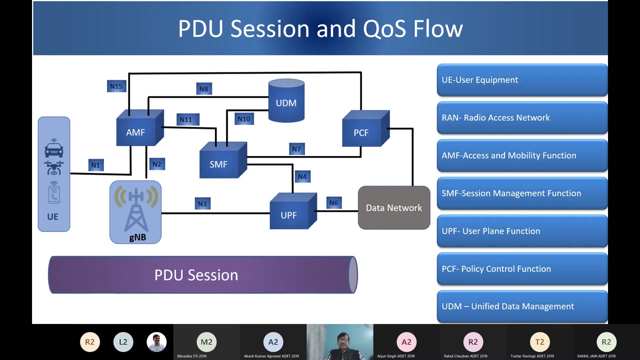 no, amf, only signaling part will be taken care, not the user plane traffic. so yes, not only amf, smf, udm, pcbs know where it will go. your user traffic goes only through upf to the data network, your radio upf and data network. so if the traffic has to go here, so that means the session which will 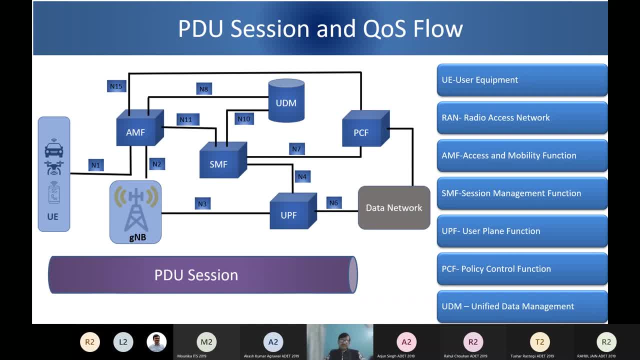 get created for an user has to be in this plane only, from user equipment to g node b, to upf and then finally to the data network. so whenever a user tries to access data either in upload direction or in download directions, what is created is PDU session. so PDU session is protocol data unit. 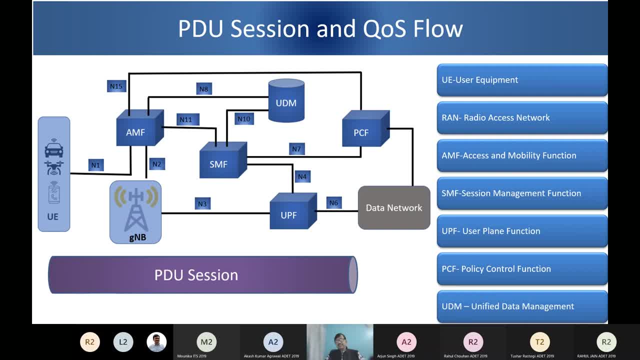 session. it's not packet, just understand. the name given is protocol data unit session. do you recall what we used to call this in 4g, Rakesh? let Rakesh answers. yes, sir, do you recall that PDU session, which is a kind of on which the 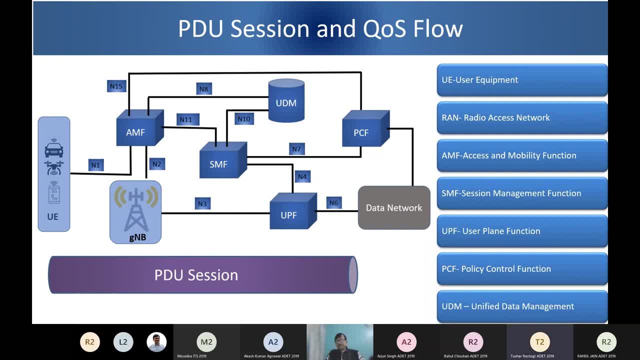 data traffic flows in 5g. similar concept was there in 4g. what was the name given to the? it was like some tunneling or something. yes, it is a tunnel, but I am asking about what is the name given here. it is a tunnel, but I am asking about what is the name given here. it is a tunnel, but I am asking. 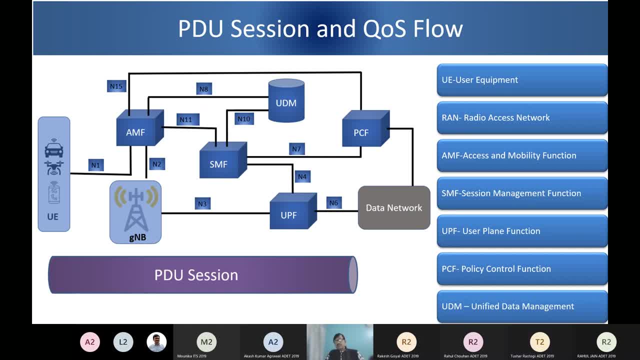 we call it PDU session. in 4g we used to call it EPS. EPS, yeah, yes, yes, yes, so it was called EPS session. here it is being called PDU session. there was another name given for EPS session in 4g, maybe Rahul, Rahul Jain, the name of EPS session in 4g. there was another name. 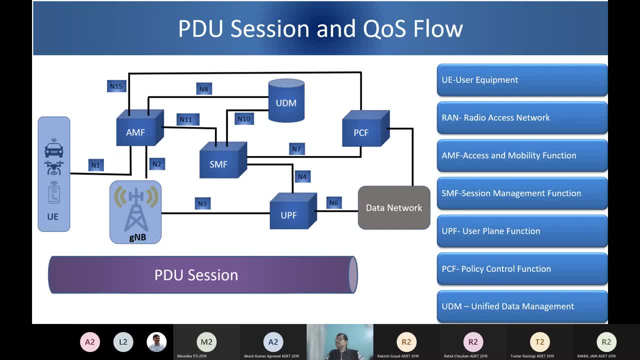 PDU session in 4g. maybe Rahul, Rahul Jain, the name of EPS session in 4g. there was another name given. do you recall Rahul Jain? no, sir, okay, Rahul given. do you recall Rahul Jain? no sir, okay, Rahul. Chauhan, Monica, anyone, anyone, okay, let anyone. 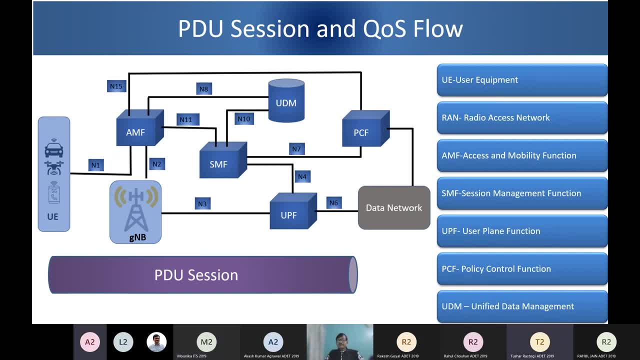 Chauhan Monica. anyone, anyone, okay, let anyone answer. so those were kind of a sub. inside the session there were certain tunnels, right? so other name given to EPS session was PDN connection. do you recall that PDN packet data connection, EPS session is equal to PDN session is equal to? 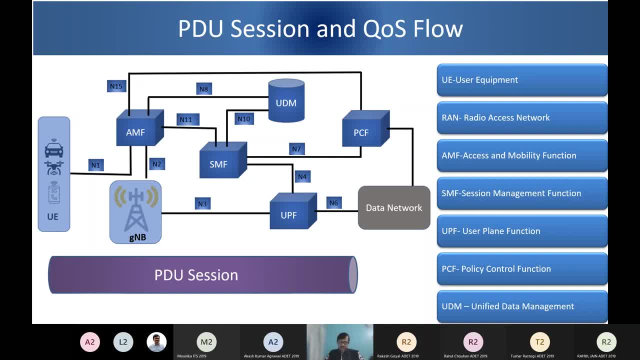 PDU session in 5g. so what is a PDU session? in fact, it is a series of connection. what it is? it is a series of connection from UE to Z node B, to UPF and then to the data network. it is just an connection, series of connection, starting from UE to Z node B. that is on. 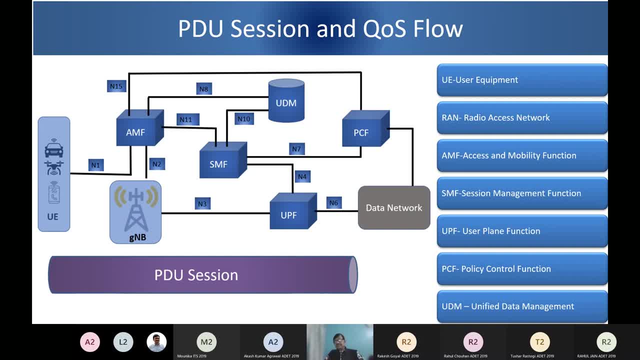 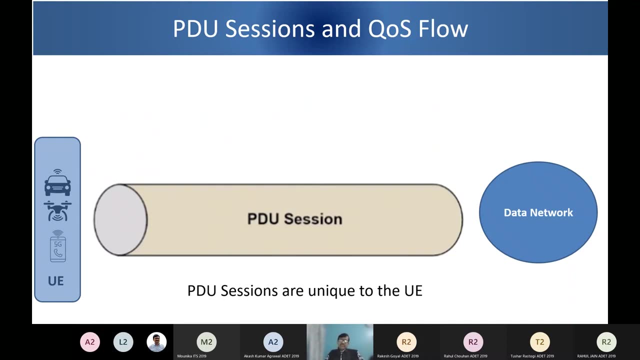 air interface, then to UPF- that is some kind of tunnel- and then to the data network. so that is your PDU session, okay, so I hope you recall your 4g, that when, whenever you attach to the network, what used to happen? do you recall that a EPS session is created for you, right? 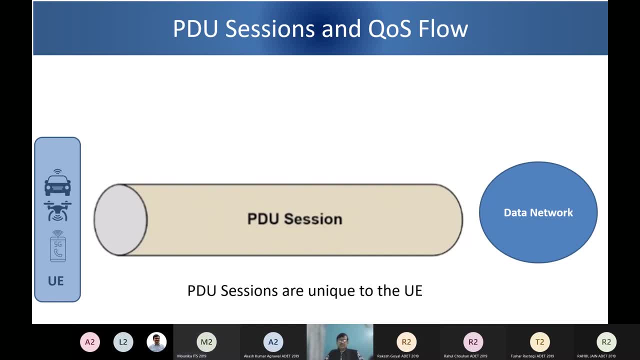 yes, sir, similarly in 5g also, whenever a user equipment connects to the network either for the first time, or maybe it want to upload or download some data in between, so a session is created for it and that is called PDU session. and PDU session will carry your traffic either in. 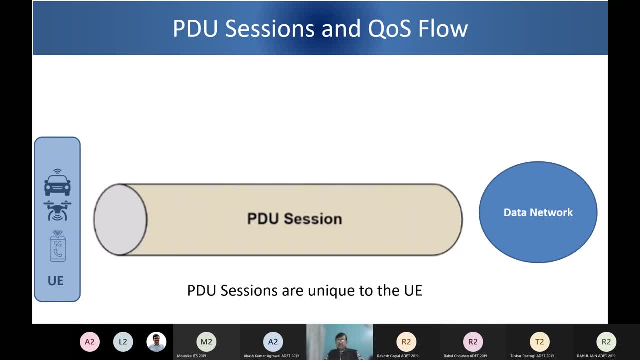 uplink direction or, in D Pizza, downlink direction. So end to end, we call it PDU session. Now the PDU session which got created is unique for a particular UE. That means one PDU session will not cater to. 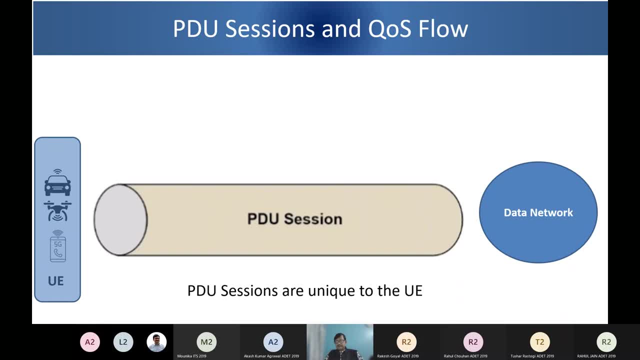 more than one user equipment. Is it clear: The PDU sessions are unique to a particular UE, But can a UE have more than one PDU session? The question is whether UE can have more than one PDU session. Any answer from any of you? Yes, sir, Yes, sir, Yes, sir Yes, One UE may have. 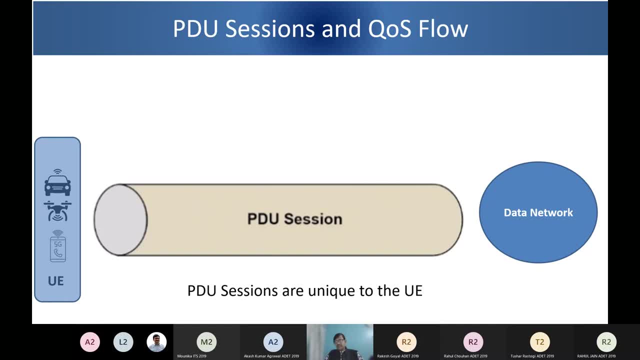 more than one PDU session. Can you tell me the scenario? What can be? scenario of more than one different applications: Yeah, May not be. May not be. Same PDU session can handle Quality of service. Carrier aggregation. Carrier aggregation can be. yes, 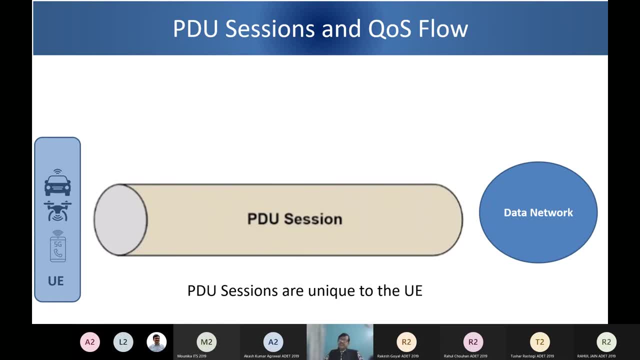 One of the example which I gave to make it very clear that in 5G we support, in addition to the 3GPP access, even we support non-3GPP access. For example, If you have, say, Wi-Fi at your home which is not 3GPP, which is not based on 3GPP. So 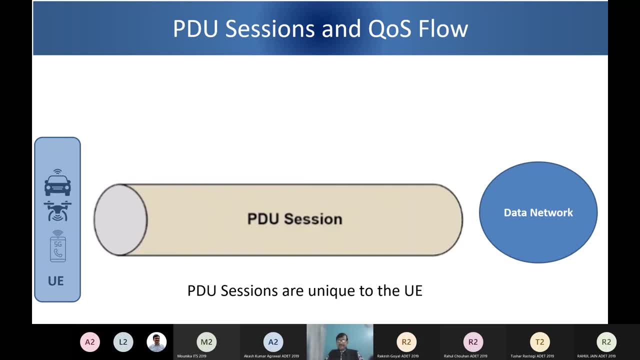 we call it non-3GPP access In 5G. such non-3GPP access can also connect to 5G core. That means 5G core will have multiple access. One is the new radio or Z-node bay. 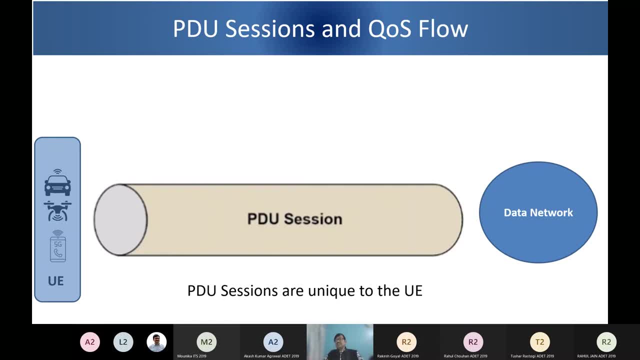 Other can be your Wi-Fi or it can even be a residential gateway. So 5G supports the multiple non-3GPP access and one device- suppose you have a 5G phone- can connect to more than one access simultaneously. That means my mobile is connected to new radio on air interface and also. 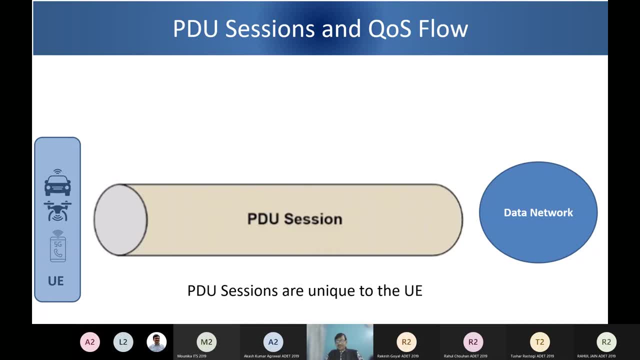 connected to Wi-Fi and getting connected to the core. In that case, if I am, if my device is connected to two access and I am having a combined data. So for me there will be two PDU session created, One on the new radio path, other on the Wi-Fi path, and finally, this will merge. 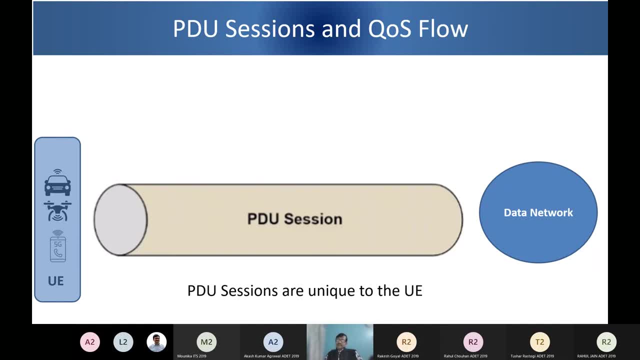 somewhere in 5G network and I will have an aggregate throughput, So an UE can have more than one PDU session, but one PDU session will be specific to one user. Now my question is: do you recall in 4G that EPS session used to have multiple quality? 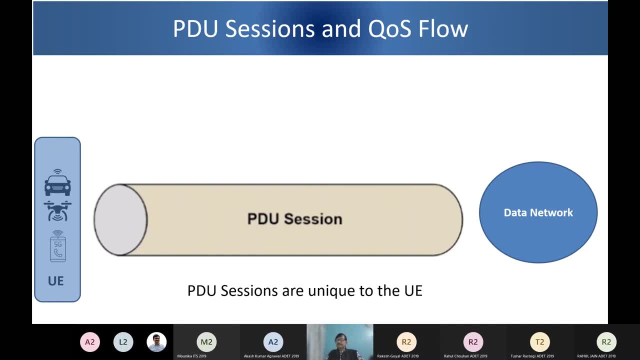 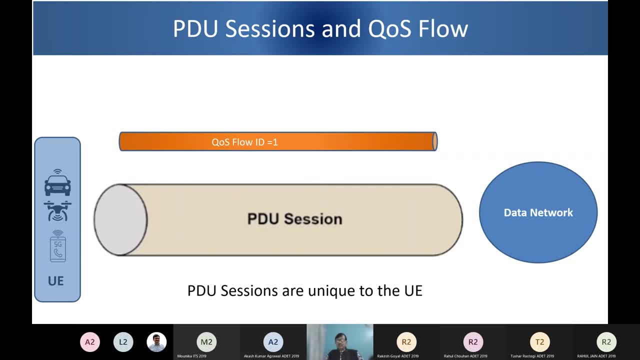 and so on, right? So here also you have. so, within a PDU session, there can be one or more QS flow, right? and here every QS flow is identified by its ID, right? So what we call it QFI, just remember QFI- quality of service flow ID. So every quality of service is identified in 5G by a number. 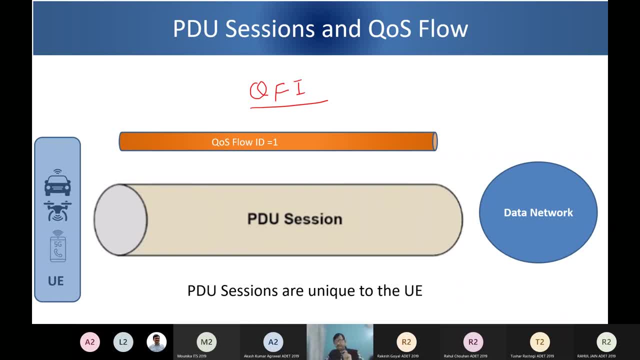 called QFI. So now let me explain you what happens when a user Is it similar to QCI in 4G. So QCI in 4G is equivalent to 5QI in 5G and it is not exactly equal to QFI. 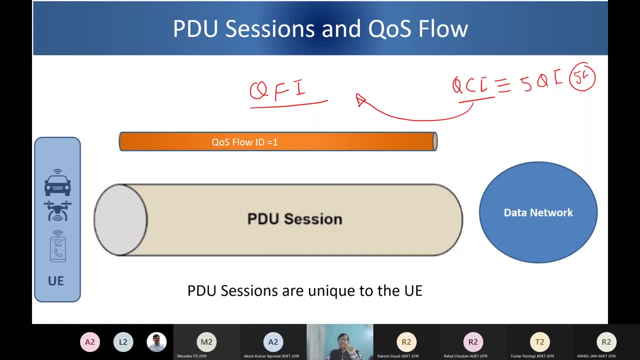 That is the difference, Because the QCI parameters- whatever parameter you have- is managed at radio interface level, Whereas there are certain other parameters at the other part of the tunnel right between, say, UPF and data network or UPF and gNodeB. we have different parameters, So QCI is only on radio. 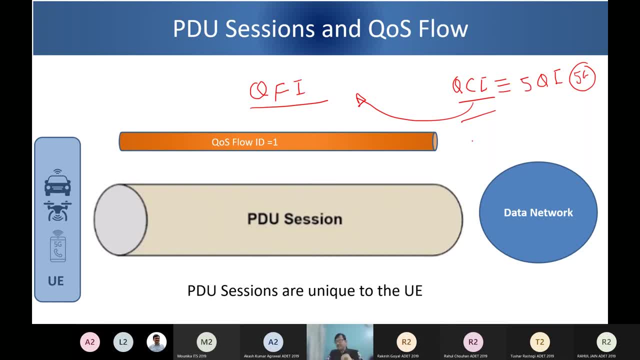 All the parameters of the QCI is on radio in 5G I am talking about and not on other aspects. So here the main identification for quality of service flow is the QFI and it is not equivalent to QCI. Please remember that this was a very good question and this is a doubt when you start reading. 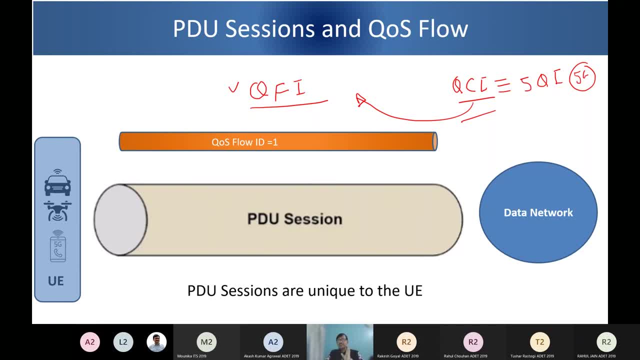 document. the first doubt you get is that QCI is equivalent to QFI. No, it is 5QI, which I will talk about when I take what I will discuss next. The QCI is equivalent to QFI. no, it is 5QI, which I will talk about when I take 5QI. 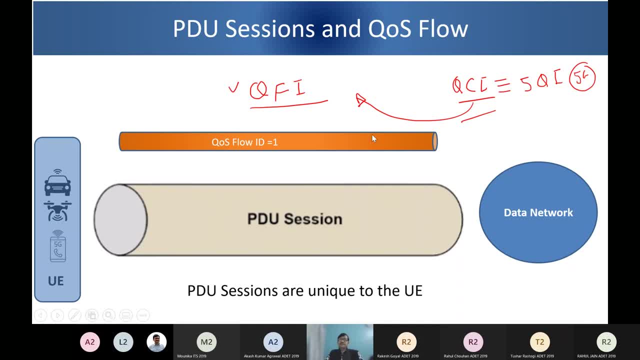 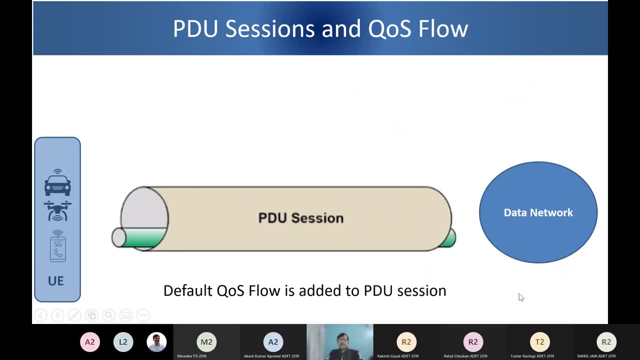 QCI is equivalent to QFI. no, it is 5QI, which I will talk about when I take 5QI- quality of service session for you guys. okay, now let me talk about what happens when a user equipment connects to the network and want to use data, so as in 4g- 4g also, you might have. 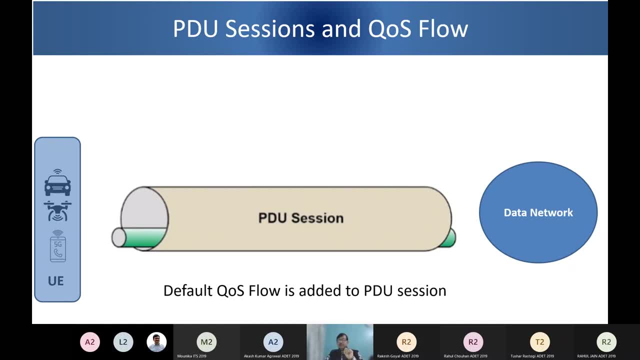 might be remembering that default bearer was created, right, you remember? you remember that in 4g. yes sir, yes sir, you had error and you had dedicated. here we call it, if i mean here we call it- qs flow only. so it is default qs flow. so whenever a user equipment gets connected to the network, a pdu session is created. 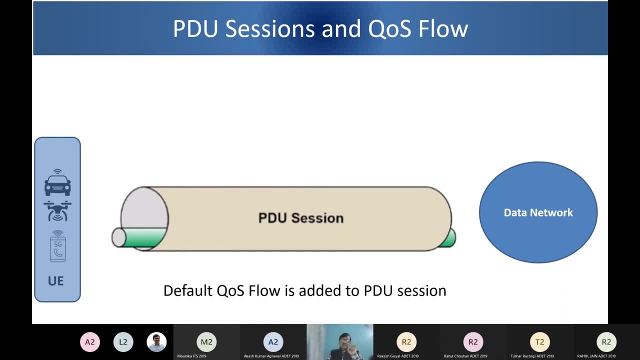 and, along with the pdu session, one quality of service flow is added, and this quality of service is a default quality of service flow and also it is non-GBR. What is non-GBR? Non-guaranteed bit rate, Guaranteed bit rate right. So default QoS flow is always non-GBR type right and this 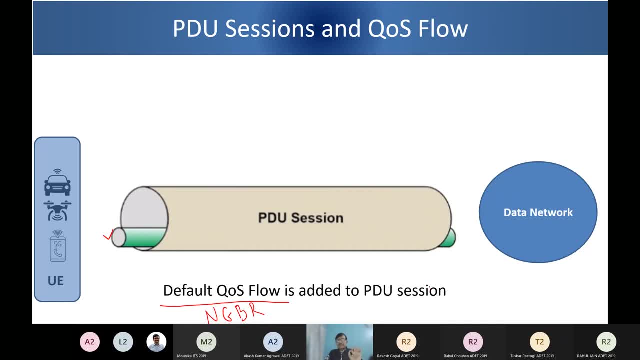 default QoS flow remains till this. PDU session is available, right. So PDU session can be actually modified, can be terminated, Suppose if no more data is being used by the user equipment. so it can be terminated, but it can also be modified. When I say modify, suppose 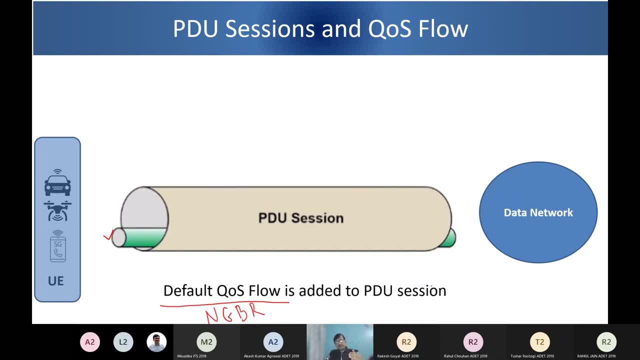 UV has this default QoS flow added and it want to use a service, Say, for example, suppose it want to make a voice call. So for voice call I need a GBR kind of QoS flow, right, And signalling of the voice is also a other kind of QoS flow that is non-GBR. So the 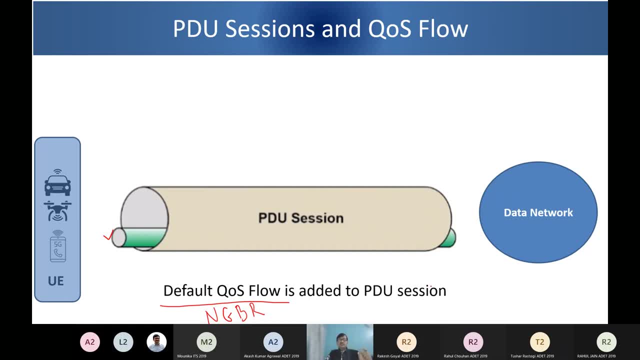 two QoS flow will be added when a user want to do a voice call in addition to the default QoS flow. Similarly, if user want to avail a streaming service which may require a different quality of service, So a separate QoS flow with GBR. 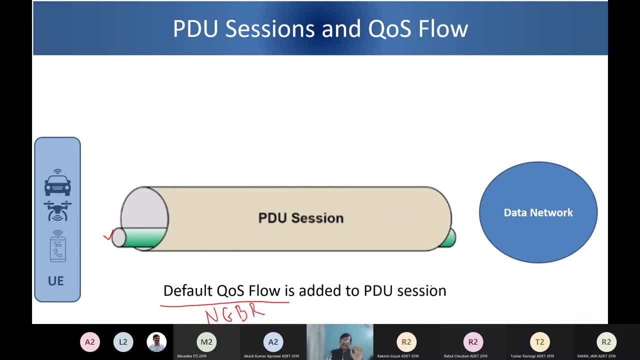 of QS flow will be added. So that means our PDU session may contain one or more than one QS flow within PDU session and those QS flow can be GBR type or can be non-GBR type and it will have various parameter defined to support that service. Any doubt till this? 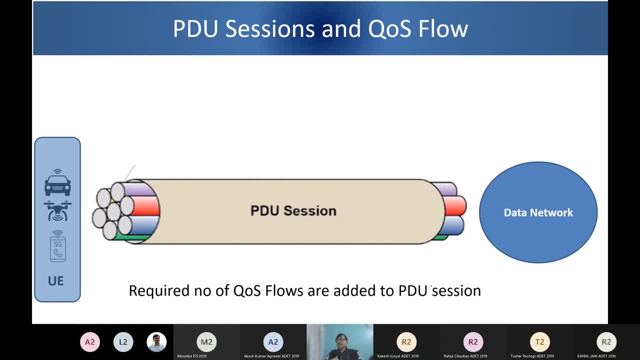 point. No, sir, Hello Sir, what is the QS flow is doing? So, basically, the QS flow is the lowest kind of a unit inside a PDU session where, for example, if you have a PDU session, for example, if you have a PDU session, for example, if you have a PDU session, for example, 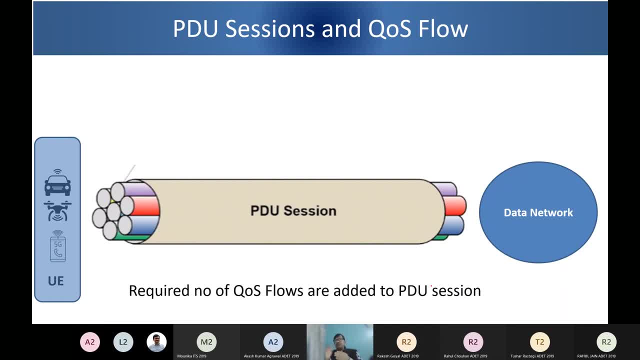 suppose, suppose a service requires X MBPS of guaranteed speed, So within the QS flow that much speed would be guaranteed. Then there is also a limit that it is not always on the guaranteed level. that is the minimum required. So the network will try to provide. 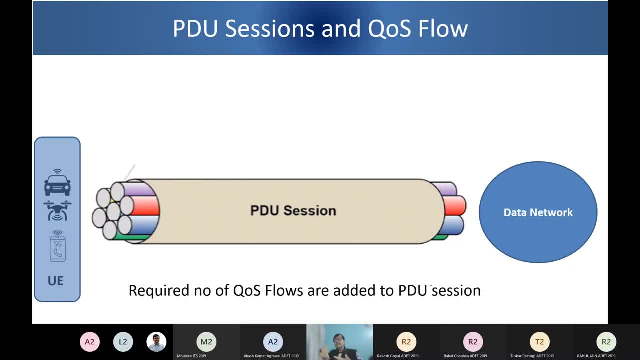 more than that. So there is also a limit of maximum bit rate MBR you might have. So the MBR will be managed within the QS flow. It will be managed in a way that it will have a minimum guaranteed bit rate and there will be a maximum bit rate also. it will. 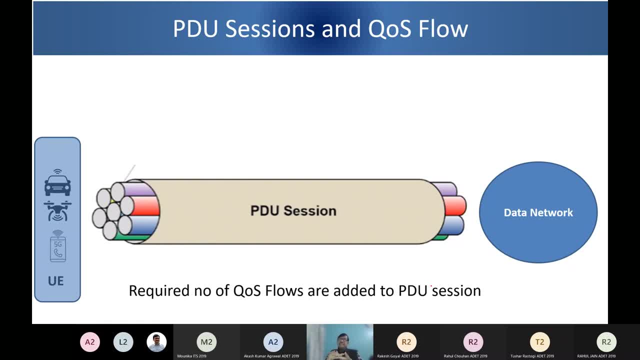 not go beyond that. Similarly, there is, there may be, a latency requirement, So that latency has to be maintained within the QS flow. So resources are allocated in such a way that all these aspects are taken care. Is that clear to you? 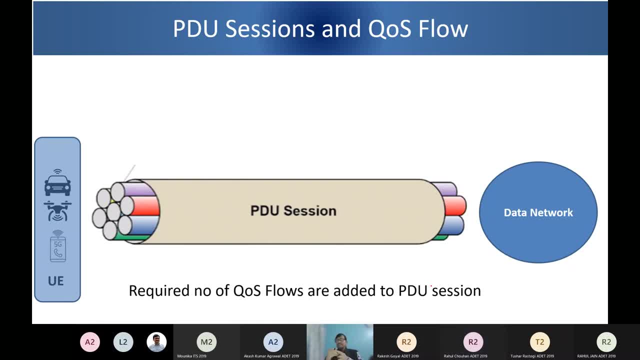 I have a question, Sir. one PDU session can have only one default QS flow or it can have multiple default QS flow. Default QS flow is only one, and then it can have many other QS flow and default QS flow is non-GBR, and then you can have n number. 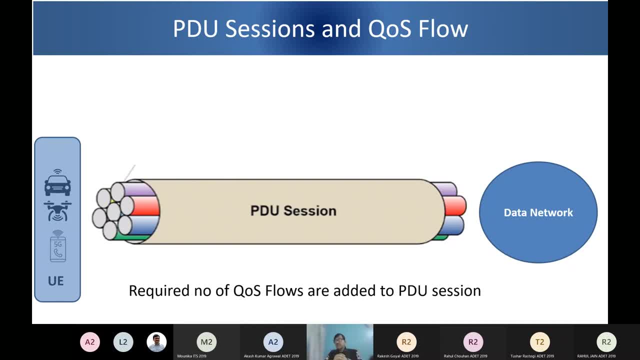 of QS flow flows, depending upon what user equipment is trying to access, and those QS flow can either be non-GBR or non-QS flow. So you can have any number of QS flows, depending upon what user equipment is trying to access, and those QS flow can either be non-GBR or 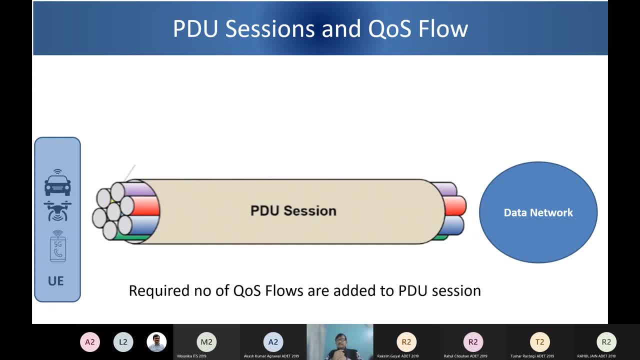 can be a GBR. Okay, So similarly in 4G, in each EPS session we can have one dedicated and one default and multiple dedicated BRO channels. Yes, I mean similar concept here. The difference is somewhere else which we will talk about. 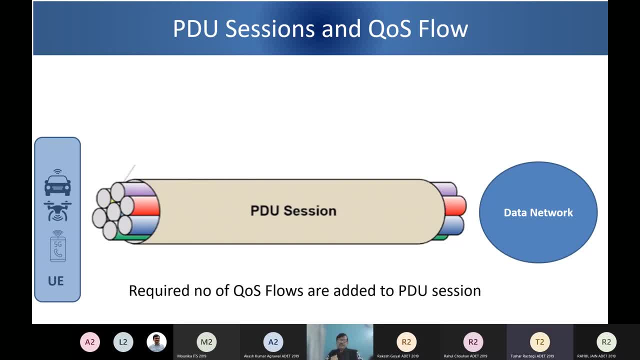 when we will have session on quality of service. Hello, excuse me, sir. Yeah, please, Sir. you have told that between UE and data network there can be non-3GBP access. Yes, sir, Also in that, also whether QS flows are there. or is it something different there, sir? 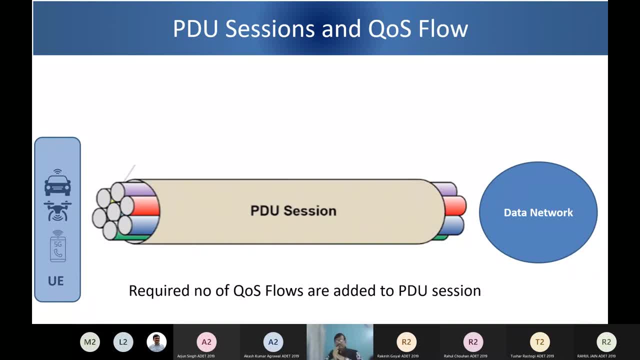 So there also we will manage quality of service right. There also there are ways where tunnel. So for example, let me tell you that suppose it is a non-3GBP wireless access, right. So it is not radio, It is just a maybe a fiber between the two or some kind of bandwidth. 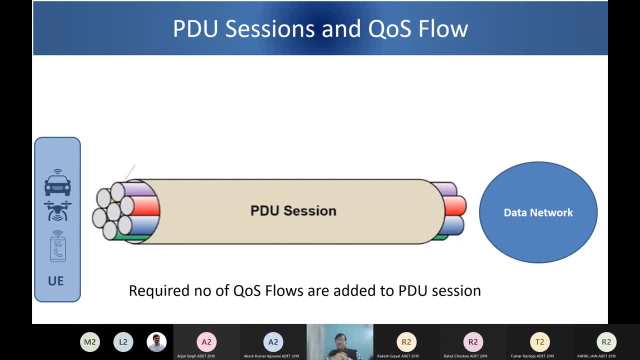 Backhaul is there, So there also similar tunnel would be created for So each PDU session. So that means we will manage QS flow in non-3GBP environment also. Okay, So like there will be one default QS will be there and multiple depending upon. 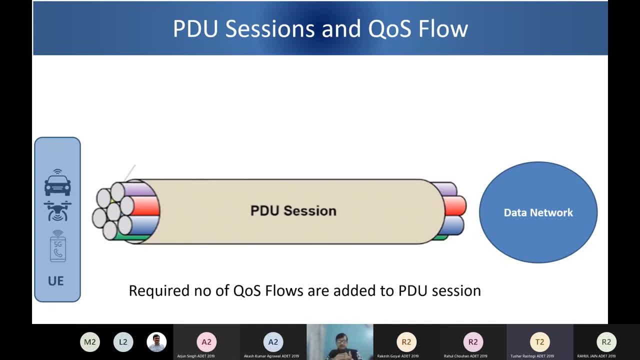 the application. there will be non-GBR and GBR QS flow like that only: Yeah, Yeah. So basically, if you Okay, Okay, So basically, if you Okay, Okay, So, basically, if you Okay. 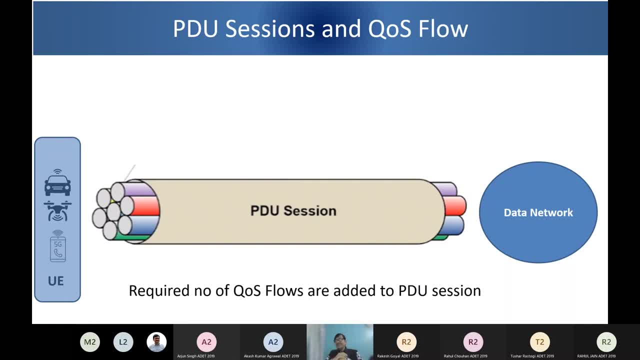 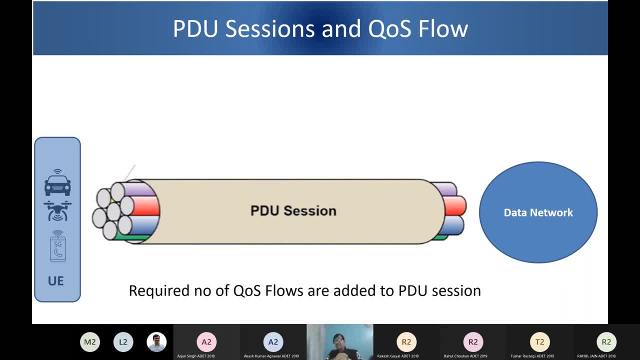 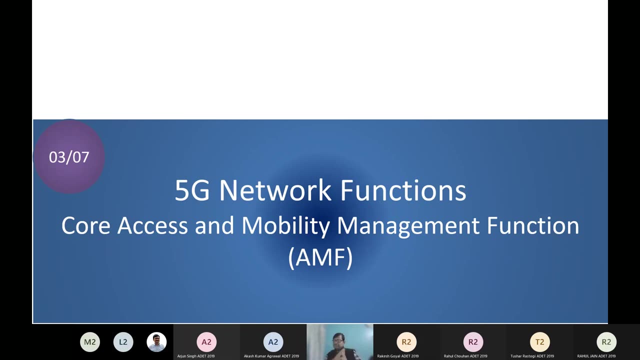 just scan through, There is a picture given how those PDU sessions are there for non-3GBP, which I will do it today itself in the first half. It will make you make this concept clear. Okay, So now let us come to various network functions of 5G, What exactly they do In. 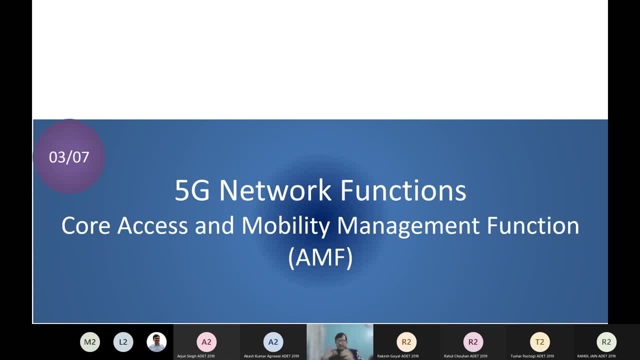 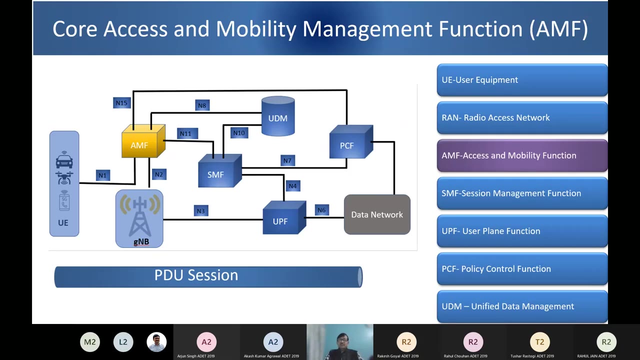 a very, very, a kind of a from a top level. we are not going into procedure part, which is a very complex one, So we will just be talking about the broad function of these five network functions which I have chosen to explain ok. 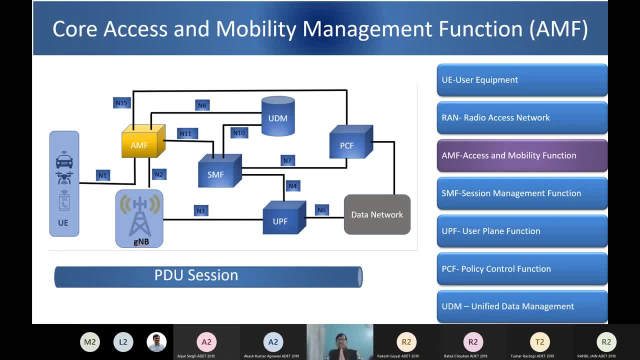 Just see this again. I have come back to that reference point: architecture. So what we are trying to cover is the AMF. Before I say tell about its function, let us see where all it is connected. So just see, it is connected to your user equipment on some interface N1, it is connected. 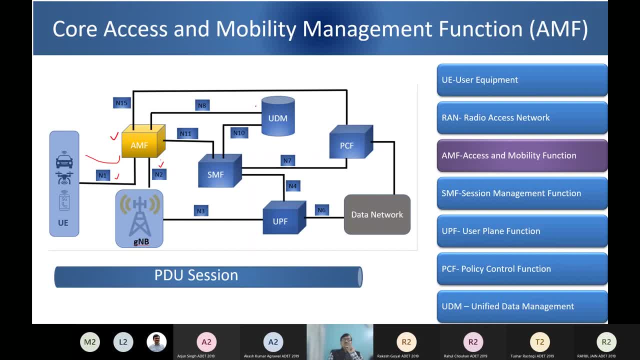 to your gNodeB on N2, it is connected to unified data management and it is connected to policy control function and also it is connected to SMF session management functions. So five interfaces is connected. It has two different network elements. 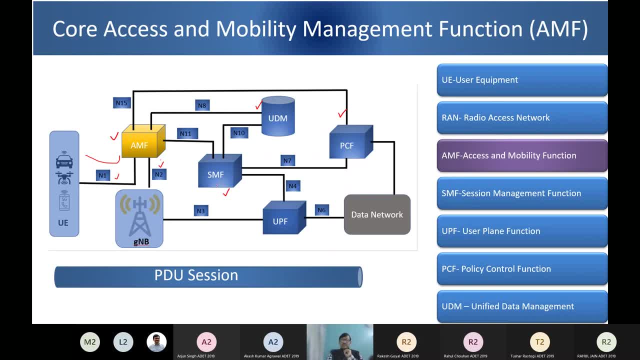 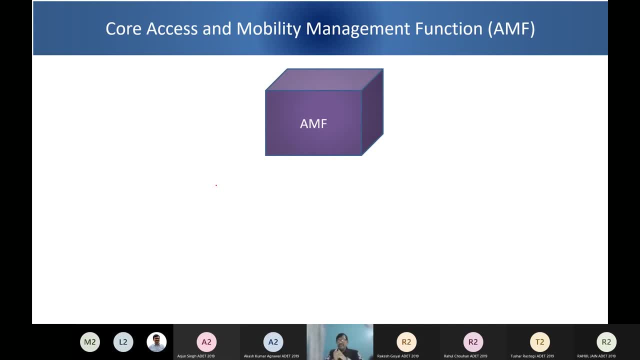 So let us see what functionality it supports. So, as the name suggests, name itself is access management right, So that means that means it has to manage access of some entity. then the name is mobility, So it will also manage the mobility part of it. 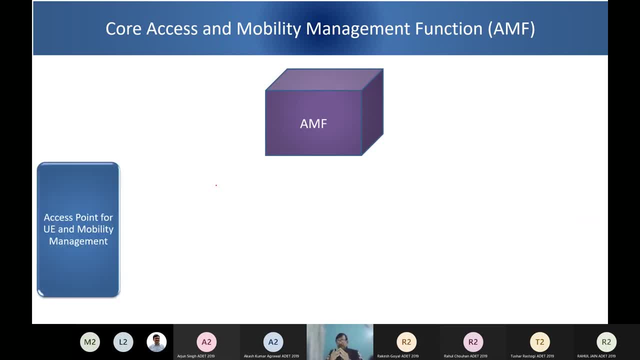 So let us start. So basically, for users, Ok, User equipment: if user equipment want to talk to the core equipment- 5G core- the access point for user is the AMF. The user is always accessing core network through AMF, right? 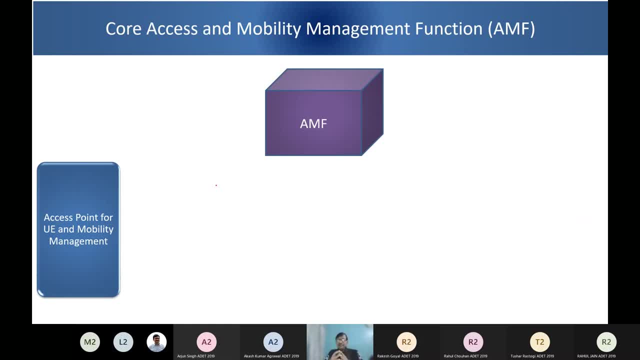 Is that clear to you? And second, Yes, sir, Mobility management. So when the user moves from, say, one gNodeB to the next gNodeB, The management of that mobility is controlled by AMF. Even user can move from one AMF area to other AMF area. 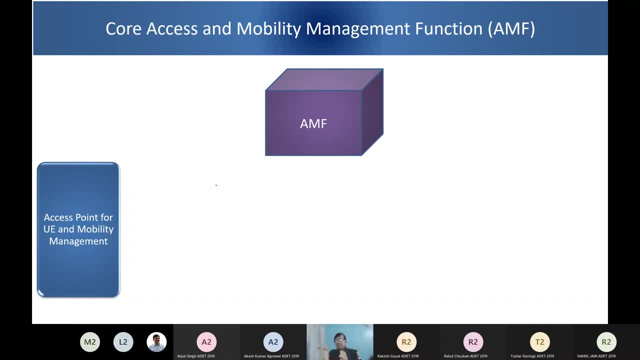 So that context exchange between the two is also handled by AMF from the respective network. There is a possibility that user equipment is from a 4G network, It is coming to 5G network And from 5G network It is going back to 4G network. 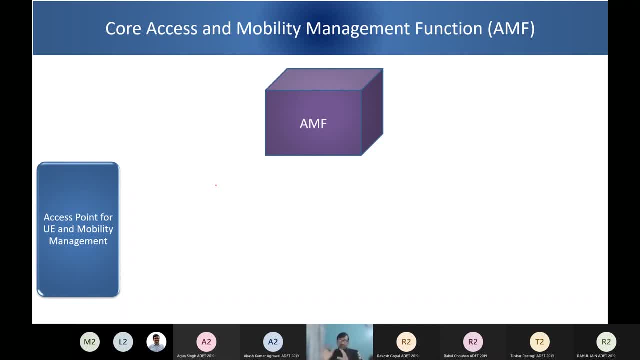 So that kind of mobility is also supported in case you have a 5G device, So that mobility will also be handled by the respective AMF and in 4G side it will be your MMA. So what we say, it is an access point for UV and also it does mobility management. 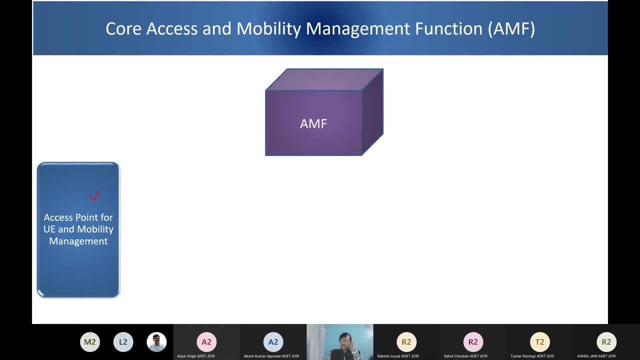 So before I proceed, May I ask you that this AMF function is equivalent to which network function or network element in 4G? Can somebody guess? May be Rahul Chauhan. Rahul, are you there? Yes sir, Yes sir. 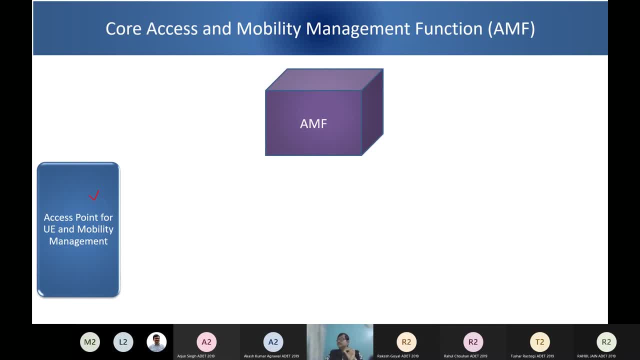 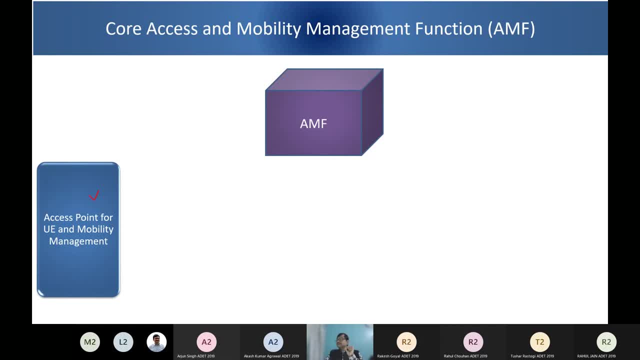 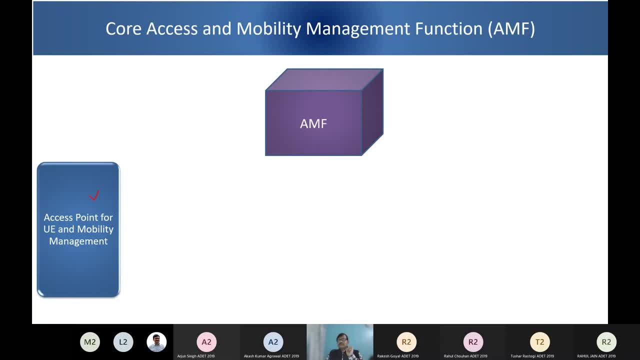 Monica, Sir, I am not sure. Ok, good, good, so quickly you can say that you do not know. so that, uh, lakshmi arjun nakas, any one of you? yes, yes, yes, very right, so m m? e is the equivalent network function. uh, but mme was doing something. 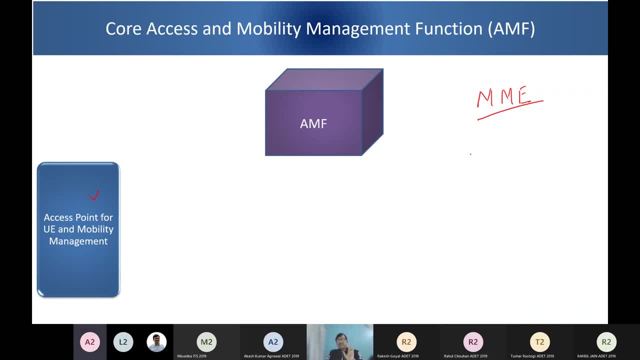 more, which we'll talk about. so at least whatever amf is doing was being handled by mme in 4g network. so mobility management entity name also says no, mobility management was also there. okay, now just uh tell me that the amf. so which network? function uh in either 4g or 5g? 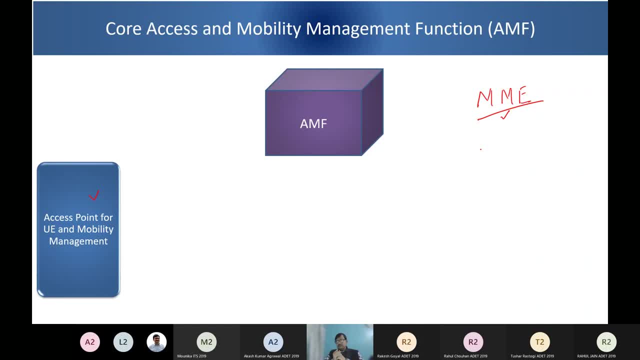 knows the location of user equipment. any idea occurs? can you repeat the question? my question is that the user locations where a ue is located, because suppose, uh, uh ue is somewhere and some incoming data call is coming for that particular ue, right, or a call, a voice call is coming, so the network should know. 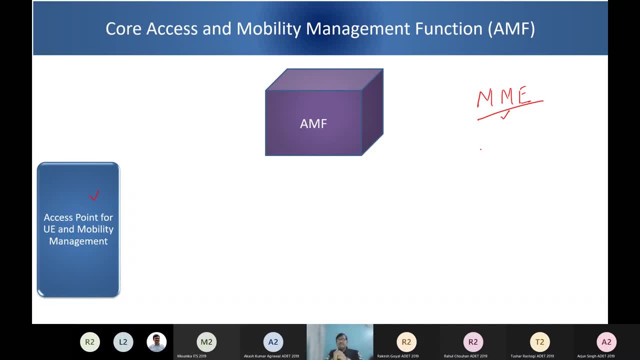 that where it is. so where ue is located, a network should know that. so in 5g amf knows the location of the user equipment access and mobility function knows the location of user equipment right or the subscriber location. but suppose uh. my question is that suppose user is active, it is uh in the sense that connected and and some kind of 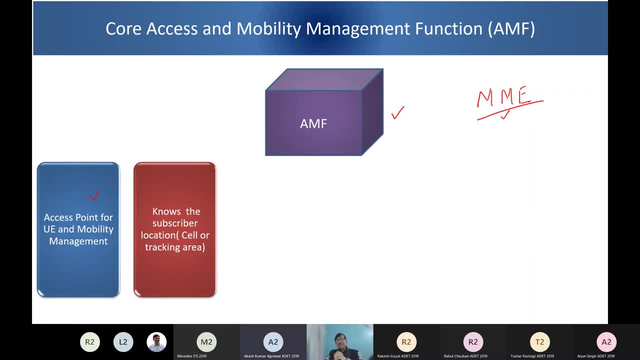 pdu session is already created. in that case amf will be knowing the location, but up to what level? my question is: up to what level? that's me. can you guess the tracking area? my question, my, my question, was that amf, i mean the user equipment, is active at that moment. in that case, up to what lowest level? 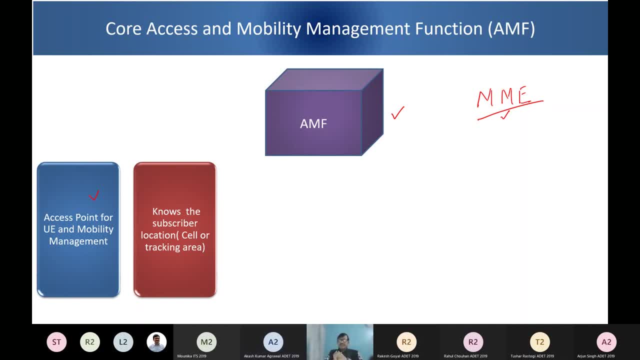 amf will know the location sell id. yes, yes, very right. so when user equipment is active, so amf will know that in which cell id the user is located and accordingly it can page and find the user equipment and data exchange can happen. and suppose now user equipment is not active. so then 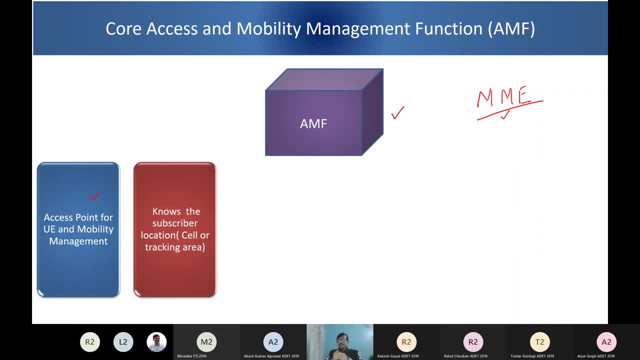 what amf knows about user equipment where it may be located. monica was answering that, monica, ranking area yes. so my next question is: what is tracking area lakshmi? what is tracking area lakshmi? just guess what is the tracking area. tracking area means i think it is a it's consists of one or more. 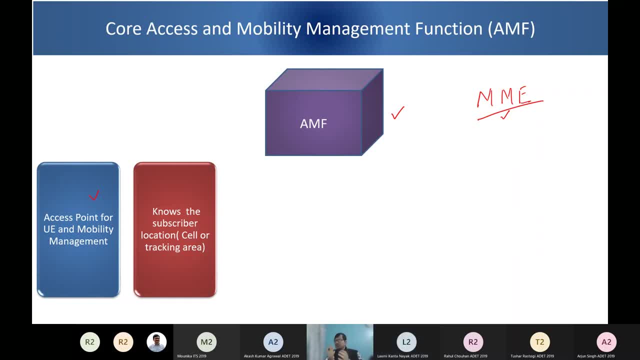 node base correct: one or more cell. you should say sorry, right. so one g node b may have, say, three cell. if there are three sectors, so one g node we may have three cells. so not necessarily that all the cells are part of tracking area, so a cluster of cells. 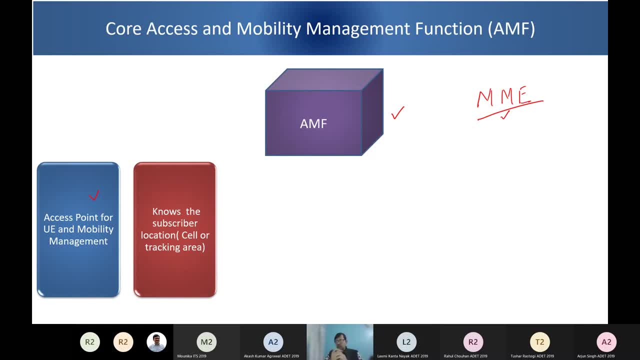 is a tracking area, so amf will at least know the tracking area of that user equipment if it is not active, if it is, say, idle, so it has to page in the entire tracking area. right, it has to send a paging message to find out that ue in the entire tracking area and the user equipment reads the. 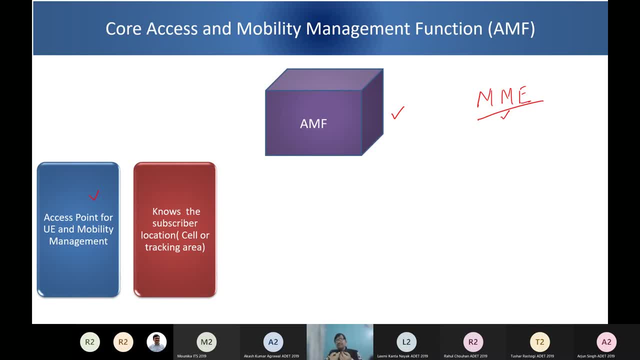 paging message and and and can identify that whether the message is for just that ue or not. so that means paging messages are read by all the ue in the area and there is an identity inside the paging message and it knows that if this message is for me or not, and if the message 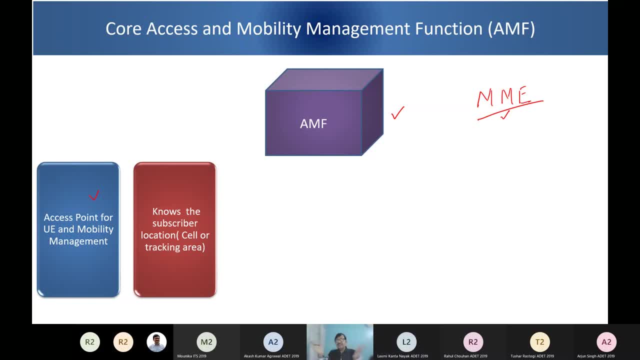 is for it, then it, uh, i mean, wakes up and makes a connection and and data exchange takes place. okay, so there is a new concept in 5g which was not there in 4g, called registration area. so let me ask some of you- uh, maybe arjun and akash should answer that- then what is registration area? 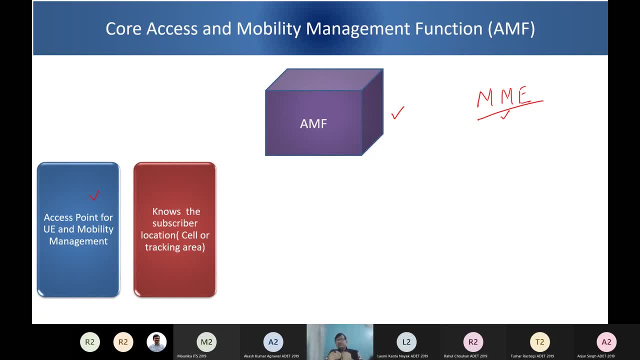 so we have now know the tracking area, we know the cell id. now, what is registration area? this question is for arjun and akash lakshmi. you can mute your mic like it's a some sort of list of- like more than one, or tracking areas, sort of tier tagging area. 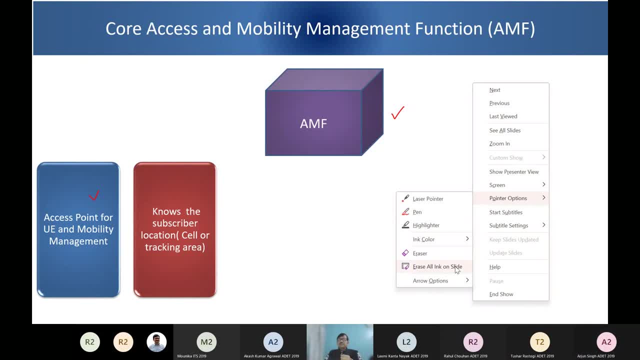 list. yes, you are right to some extent. so which tracking area would be added in the list for a registration area? any guess? akash nearby whenever i mean a user is moving, okay, okay, okay. so basically it is based on the mobility pattern of the user equipment, for example, suppose, suppose, uh. 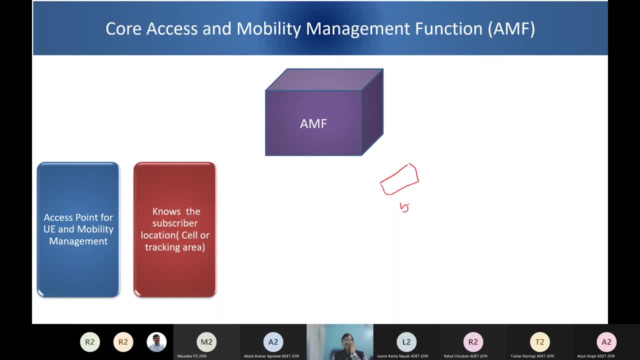 in a bus. suppose i have a bus and in this bus a iot device is there. that means it has got an 5g connection. so it is a kind of a ue and this bus travels from, say, anand vihar in delhi to new delhi railway station, right, 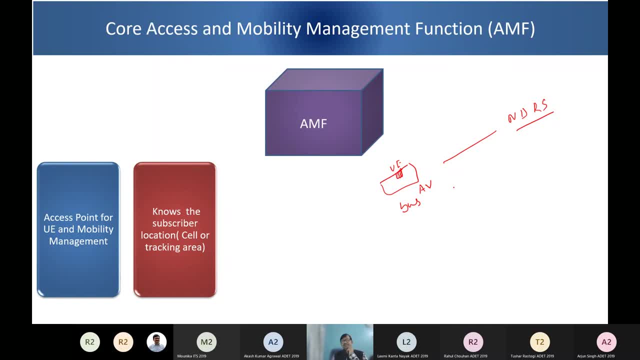 so this area, if you see, may consist of very various tas, right ta 1, 2, 3, 9 and so on, tan. okay, so this bus every day goes new delhi, comes back. so system knows that this bus is going from anand vihar to railway station on daily basis, so it will create a registration area for. 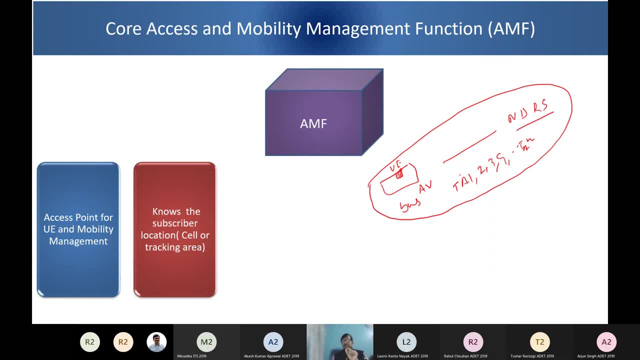 the specific ue like this, that it will consist of all these tas. so, and whenever uh ue is in idle mode, the paging will be done in the registration area, right? so what is the benefit of having a registration area instead of tracking area? it will become a faster, precise identification. 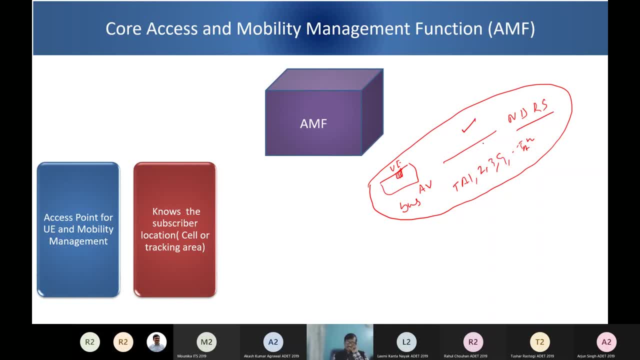 like, it will be very easy to locate the users because we know that area. yeah, so main idea behind defining registration area was to reduce signaling overhead. to reduce signaling overhead. so how this signaling overhead will be reduced. akash. so how this signaling overhead will be reduced. akash. 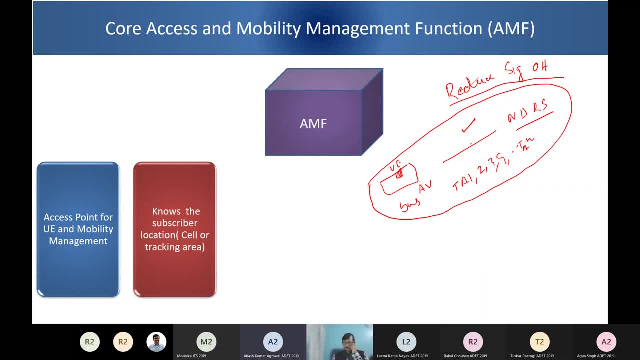 uh, because now, uh, it will automatically predict what. what is the next cell is going to be. so without, i mean, from the core network, it doesn't have to switch to the new cell and it will automatically switch. okay, let me explain further. suppose there are ta1, ta2, ta3, ta4, right, let us assume that there. 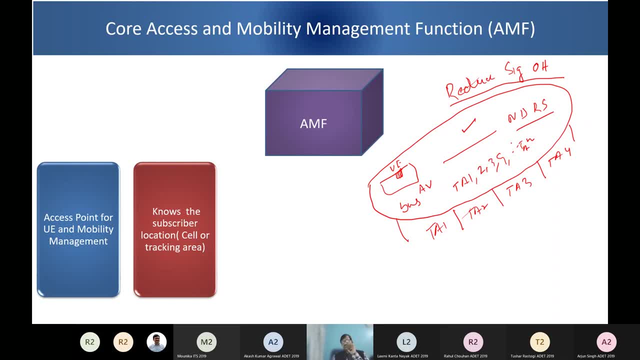 only four tas in a registration area. if this registration concept was not there, then your user equipment: when it crosses ta1 to ta2, it has to do an update with the mf. that is called mobility update, right again from: if it moves from ta2 to ta3, it has to do a mobility. 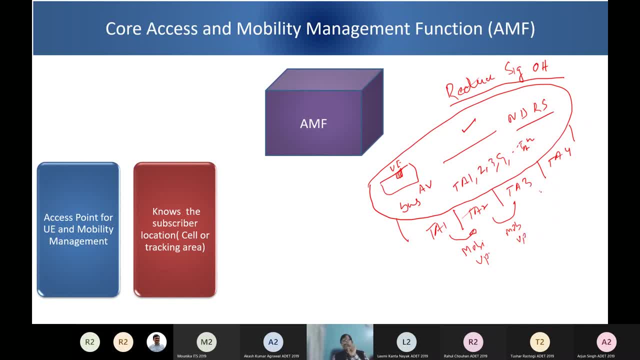 update 4g it is. it happens like that. and then again it has to do a mobility update, and then again it has to to do a mobility update and again, while coming back it has to do So. it has to do n number of mobility update which is adding to the signaling right. So and also the battery. 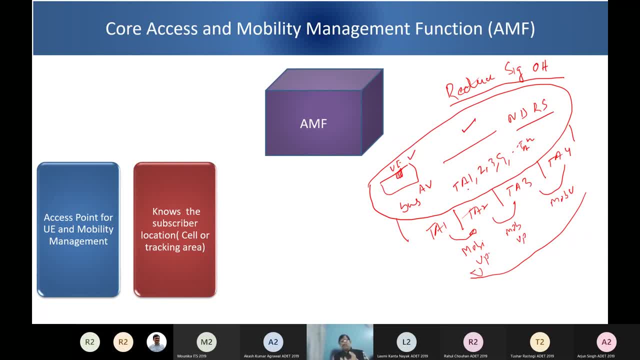 of that chip will drain, because every time it has to go, because go active and do a mobility update right. So with registration area concept, we have reduced a huge amount of signaling overhead. Is this clear, Akash? Yes, sir, but I have one question. is that is? 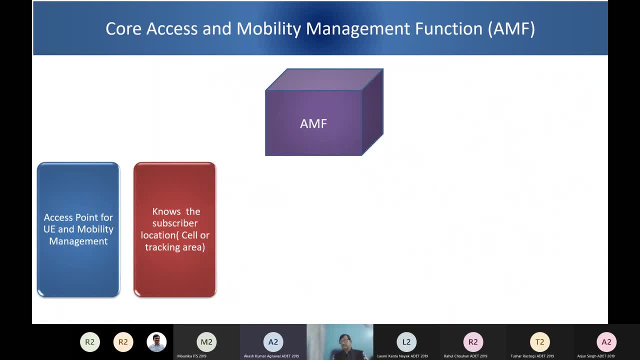 it the requirement for the. I mean the location. the position of the device needs to be more accurate for 5G. So location is nothing to do with the location of the device. So location is nothing to do with the location of the device. So location. 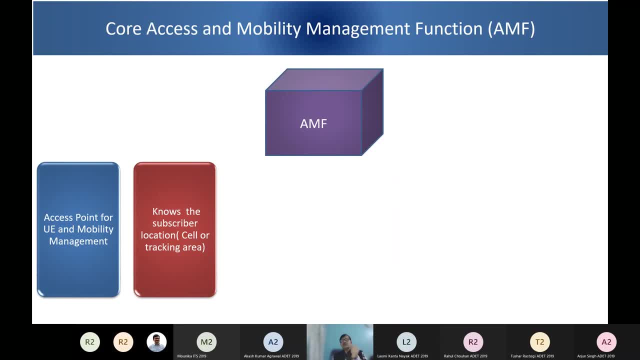 is nothing to do with the location of the device. So location is nothing to do with mobility update basically. So location will come suppose the bus is programmed to provide location right, So that location will come as a data right. So whatever is, 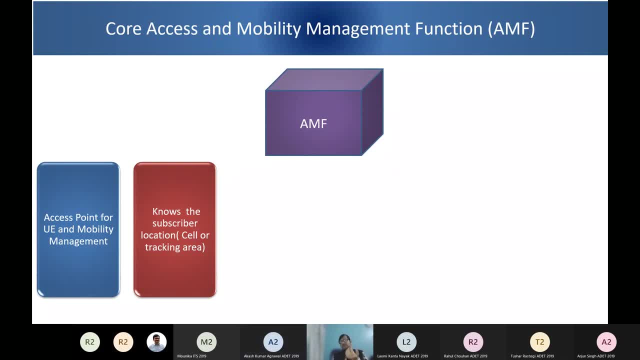 programmed. suppose you have programmed that every 5 minute it should pass on the location, or 10 minutes. So at that point of time it has to just send a small data message to the server and done So. signaling are over and above the data, So those are user plane, data, So user plane. 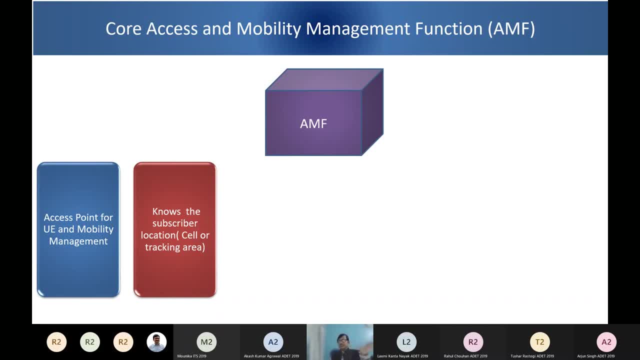 data. whatever you have defined for that IOT device, it will be doing. there is no doubt about it. but we are reducing the signaling overhead, right, Suppose, sir. but if there is a car nearby which is also travelling parallelly to the bus, but somewhere they take a detour. 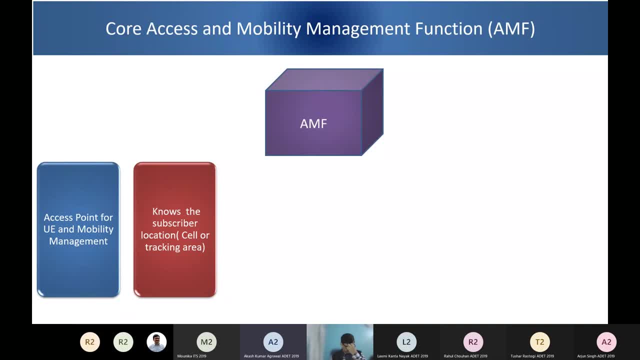 from the bus. So is it is in the, I mean the core network- get confused if their location is not accurate. No, no, no, So it is not about So here. registration area is unique to a user. This concept is: 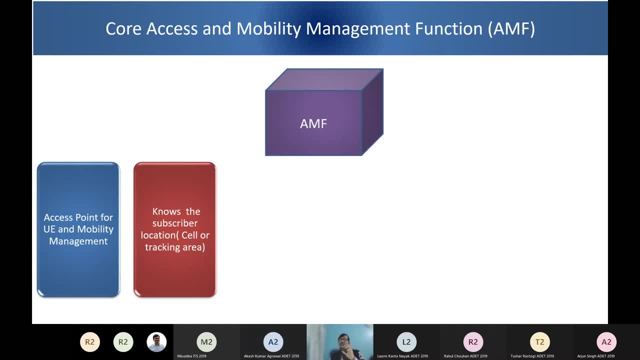 very new. Earlier, the straight tracking area was common kind of right. Yeah, It was not a unique to a particular UV right, So it was not specific to a. here we have made registration area unique to a device. and not only that, there is one more concept. 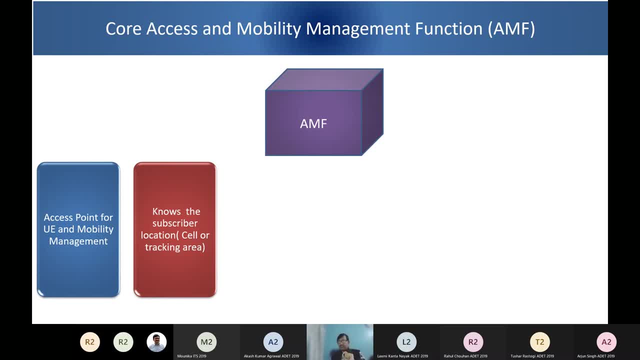 One is that when you provision a customer into the database, you can define its registration area first, from the day one, If you know that this particular user is an IOT device and it has to always remain at one location. Suppose it is an static IOT device. Suppose your fridge. 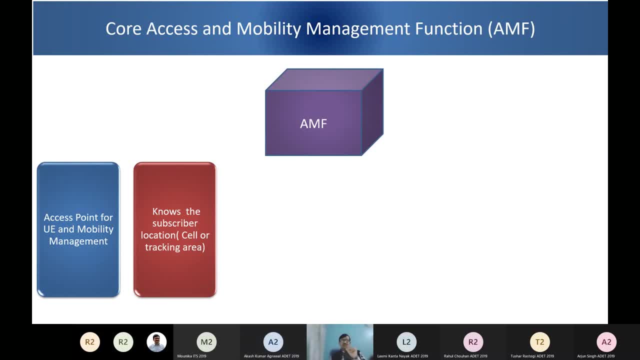 is having or your TV light is not working. So you can define it as static IOT device. So you know the precise location where it is located. So you define its registration area as only a kind of a particular cell, right within that cell only. it has to remain right. 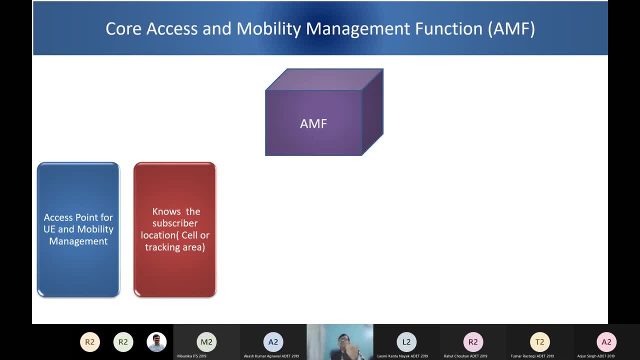 So it will not do even a mobility update, It will only do a periodic update, right? So that is the concept which has come in 5G, that, depending upon the mobility pattern of a device, registration area would be set. that is one. 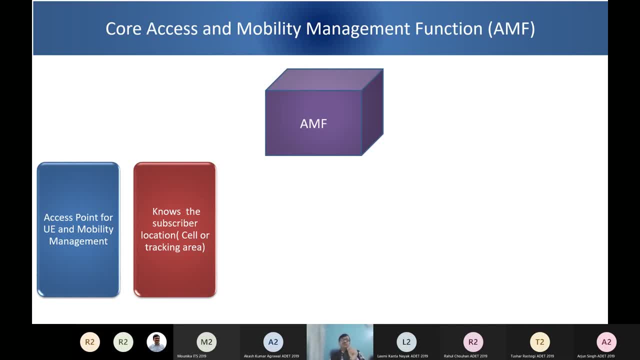 Second concept is that it learns. Suppose, when my number is provisioned, then it may not be having a registration area defined for me properly, but over a period of time they will notice that I go to my office that is anti-aparate from my home that is in Vasundhara. 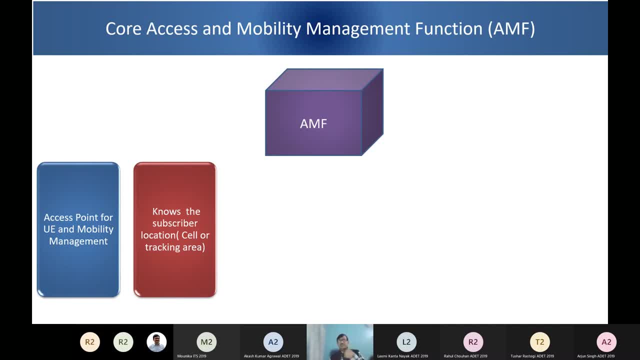 So I go. that is a 20 kilometer stretch. I go and come back So they can define this as a registration area for me after learning that my mobility pattern is this. So these are the concept which is a new in 5G. Shall we proceed. 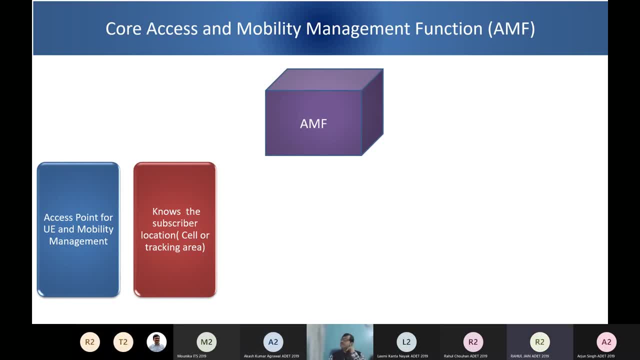 Okay, Okay, sir, Sir, is this registration area flexible, like, Yeah, Let us say you are going daily to office, but for, let us say, for a month you go on a tour and then new registration area. So you have a new registration area will be defined there. 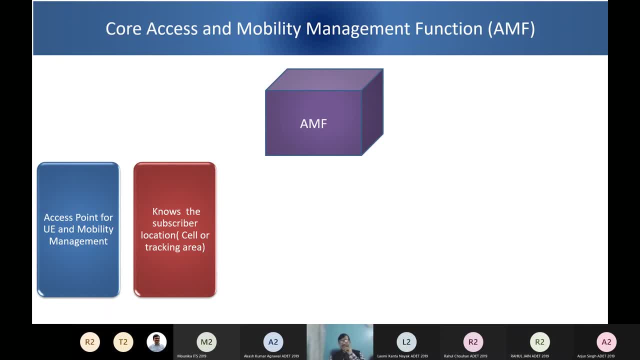 So it learns, As I said that it is a learning right, So it will see the pattern which is regularly used, right? So if you have start using a regular pattern, suppose you are in Delhi and now in Bangalore, So it will learn and make that as a registration area. But 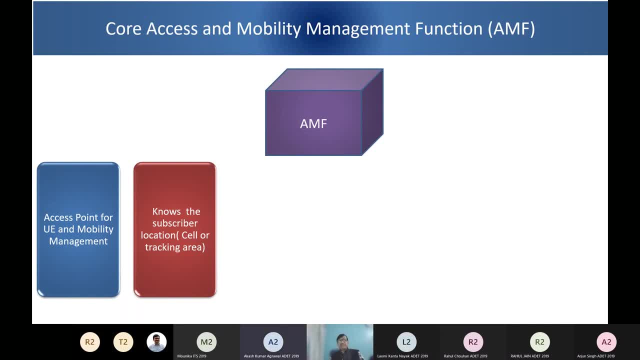 if you are going for a depend upon what is getting configured- that for how long they will learn your about your mobility pattern and will accept as a registration area. That depends upon the configuration. So AI ML kind of a thing will come into picture for. 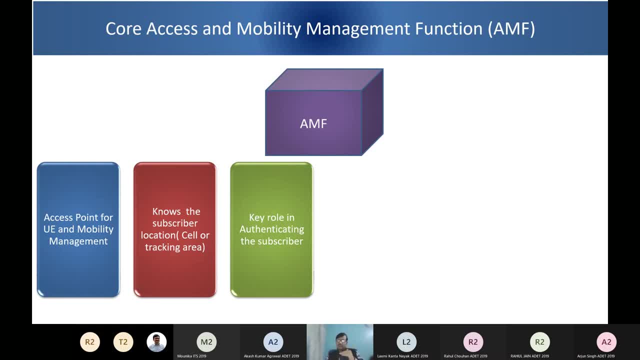 such aspects. Okay, So now that we know that user equipment accesses core network through AMF, so that means AMF has to play a key role for authentication of the subscriber. So in fact, AMF doesn't do authentication, but it plays a role in. 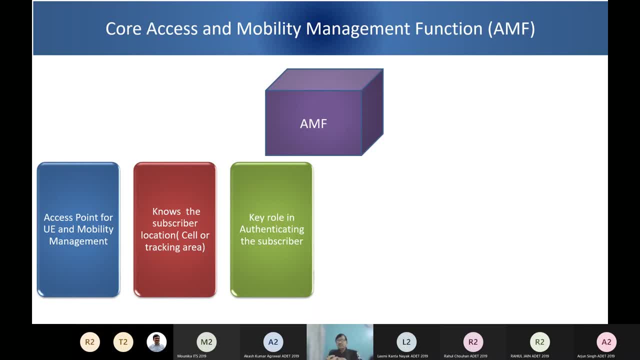 the sense that somebody is coming through you, so you are opening the door or closing the door, kind of. so you play a role in authenticating the subscriber. Of course, authentication has to happen using the AUSF and UDM, but it plays a key role. 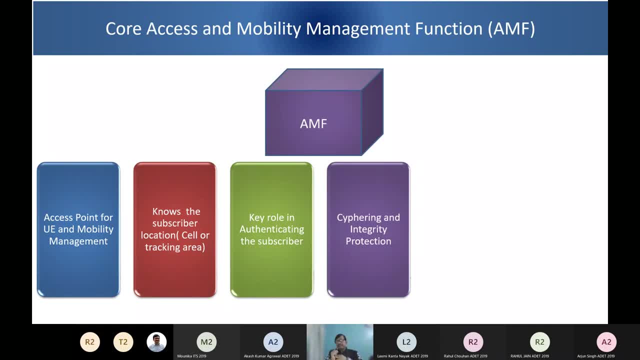 Next is ciphering and integrity protection. Let me ask: what is ciphering, then? what we are talking about? When I say ciphering, what I mean? maybe Monica? Yes, sir, The next function of AMF is ciphering and integrity protection. So, what time? what we mean by ciphering? 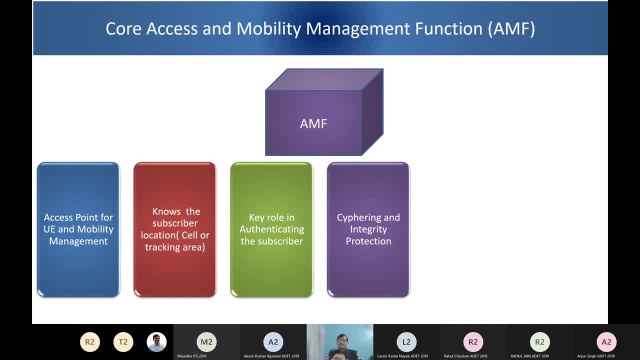 Ciphering is encrypting, Right Encrypting, And second is the integrity protection. What that mean? Integrity means like the message will be unchanged, It will be sent as it is. Like no unauthorized modifications are not, will not be allowed. Okay, So maybe if somebody else want to, 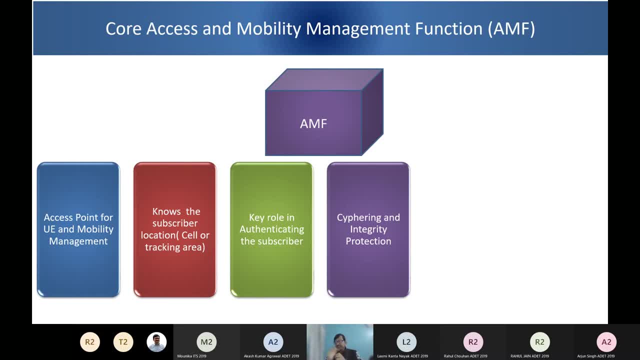 pick up this question and answer in a better way. Monica, you are right, But let me ask anybody else. Okay, sir. So, sir, if you like to add up on this, Ciphering means encryption of the data, and integrity protection is like whatever I am. 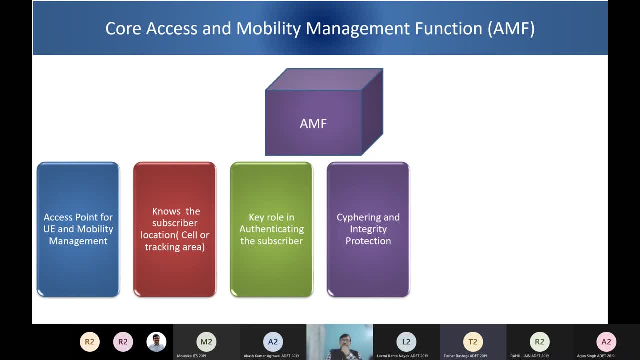 supposed to send the same information is received. It has not been modified in the middle by someone. So I think for that we generally use the hashing, We hash that and at the other side also we check Whether the same hash is received, so that through that we can get integrity. sir. 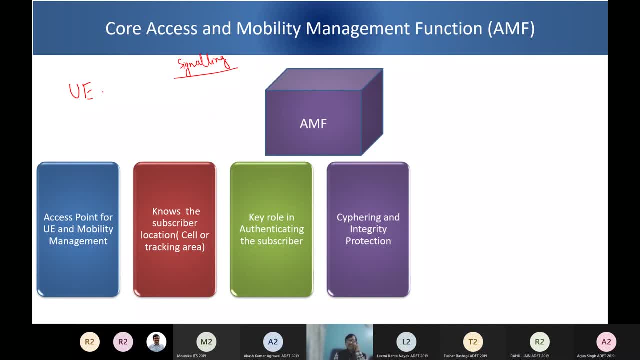 Yes, So to Sarah is right. So basically what you are saying- that when something is being sent to AMF and it is a signaling, so we know that you interact with AMF is just the control signaling. So one is the ciphering part, that whatever data you are sending, you are encrypting. 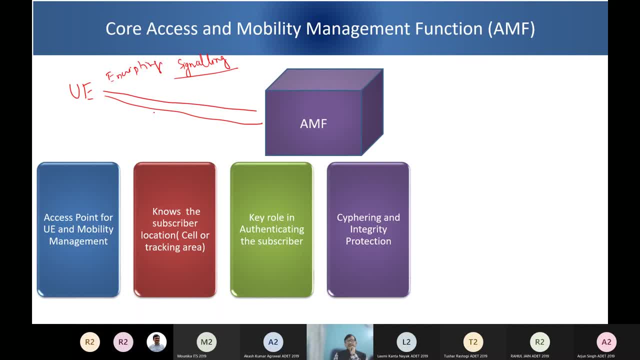 right. So when you are encrypting, that means no one else In the middle can access to it because it is already encrypted. It is a kind of a garbage. Even if you are able to somehow intercept this, it will be a garbage because you will. 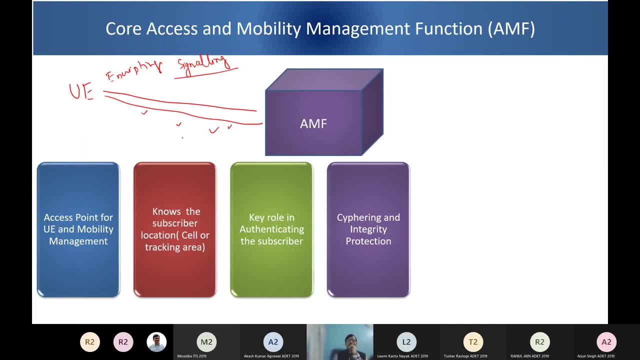 not be able to decrypt unless you know the keys right. And when we say integrity, we have to ensure that, yes, it is coming for the UV from a intended UV one side- Okay, It is coming. It is not that a fake UV. Suppose there is a fake UV right And it starts sending. 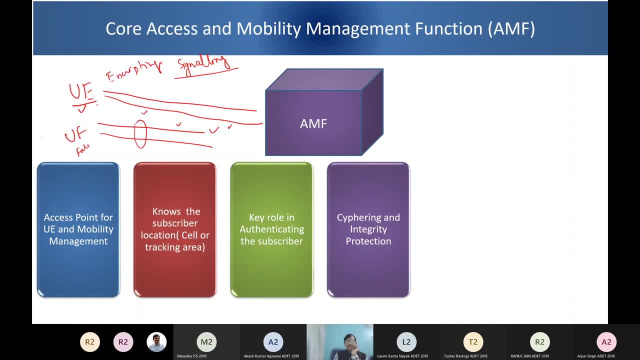 it will use encryption, everything fine, but it is not coming from a genuine UV. So this is your integrity. So that means UV will verify that whatever is coming from AMF is coming from the right AMF. AMF has to ensure that whatever is coming from UV is from the same. 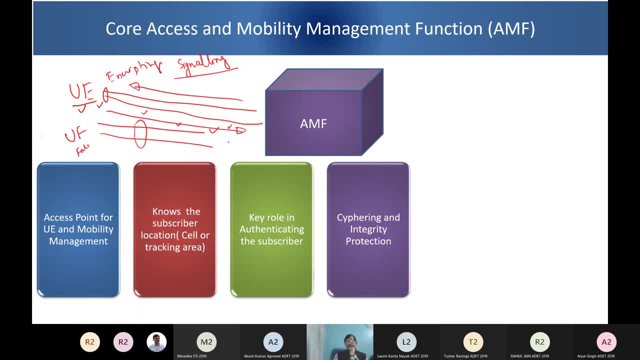 UV which it knows It is not from a fake UV. So that is your integrity protection. Okay, Now the next function of AMF is providing a temporary ID called GUTI 4G. also, we had concept of GUTI and you guys have perhaps studied, So maybe you have read the technical. 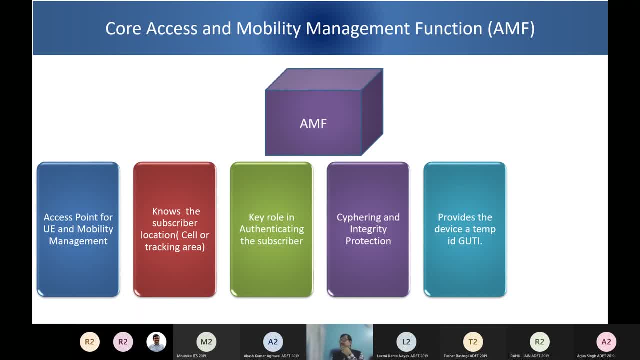 information. I do not have to go into detail now, But the model is called GUTI And it be. let me ask, Rakesh, if you are aware about GUTI. So it is in 4G. it is like RNTI, which is equivalent to RNTI. 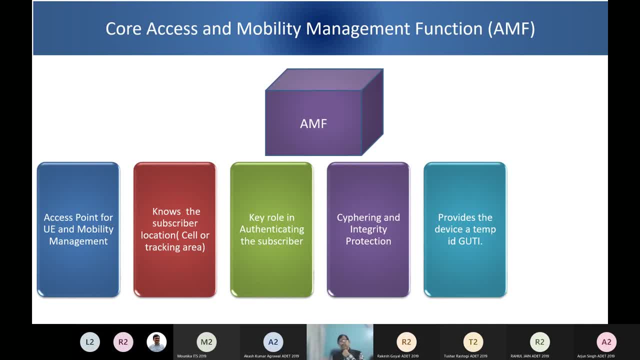 No, no, it is not RNTI. RNTI is only on to the radio, that is between eNodeB and user equipment in 4G, and here gNodeB and user. we are talking to core now, So it is not RNTI. 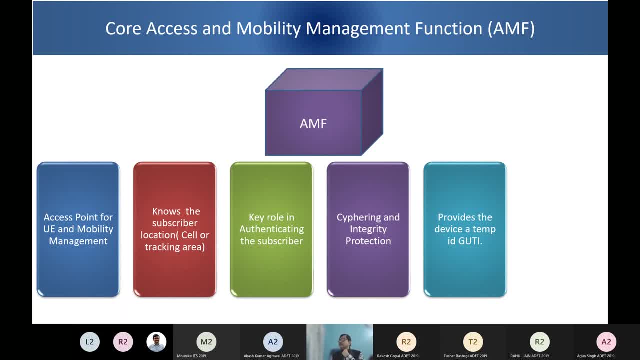 Okay, so maybe Tushar. what is GUTI, Sir? what I remember is like to keep IMSI confidential, sir, Very right. So you are right, You are very right. So just recall and tell me. 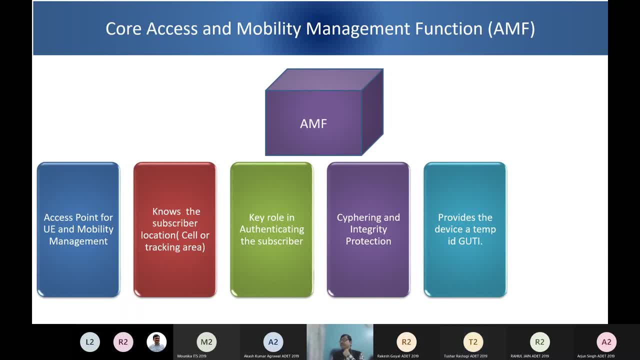 I know this, only I remember that. So you are right. you are right. Let me ask Akash Akash if he is He is aware of Sir. it is a combination of three IDs, in which, no, I do not remember sir. 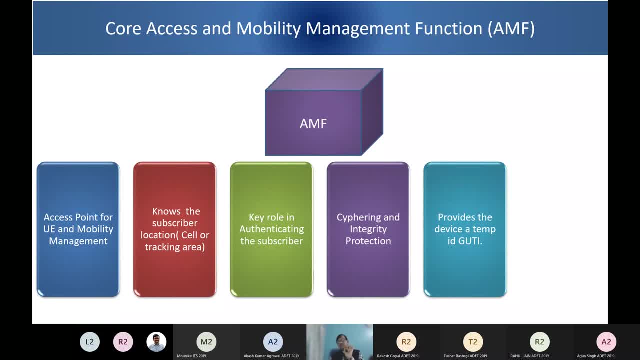 Okay. So let me first tell you. it is GUTI means Globally Unique Temporary ID. What is it? Globally Unique Temporary ID, Okay, And which? Which network function allocates this? It is allocated by AMF. 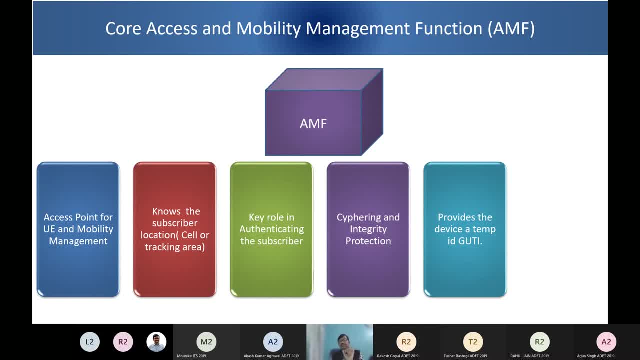 So just remember that AMF allocates a temporary ID called GUTI, Right? So let me just explain what Tushar was trying to say. So suppose you have a user equipment, Right? So user equipment when it accesses. 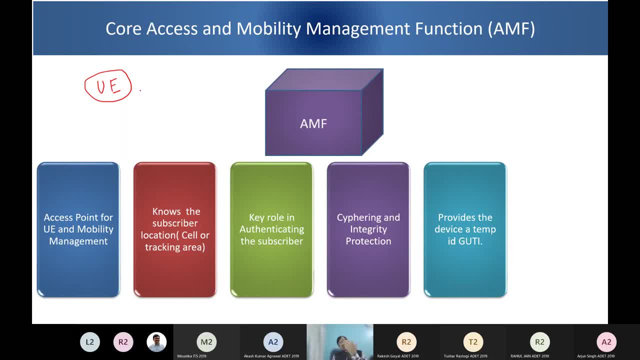 The core network. it has to prove its identity. Right, It has to prove its identity. So it has got options. So either it can send IMSI or it can send a temporary ID that is GUTI If it is already allocated by AMF. 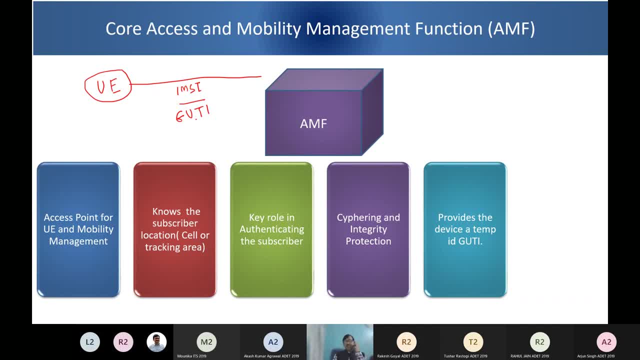 Right. So for the first time, When you will try to access the network Right, When you will try to access, It is not allocated GUTI as yet. at that point of time it uses the IMSI. In fact we call it SUPI in 5G. 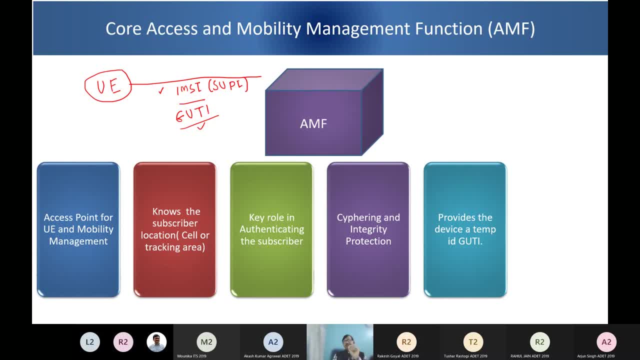 SUPI is Subscription Permanent ID. In 5G we call it SUPI. Basically, one of the SUPI can be IMSI And thereafter, once a temporary ID is allocated, it uses the GUTI on-air interface, So that 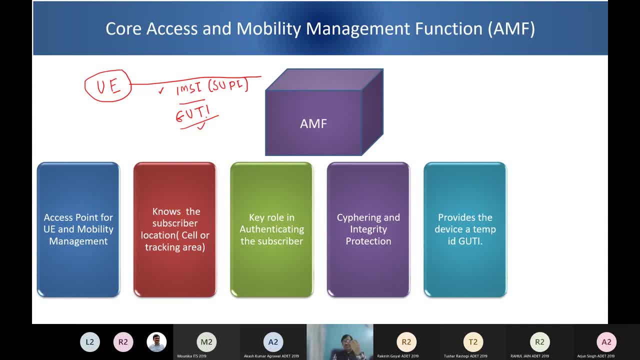 I mean it becomes more secure that it is not using its permanent ID. One more thing which I would like to tell you: that here in 5G, very different from 4G, even IMSI is not kind of transmitted in a plain text. 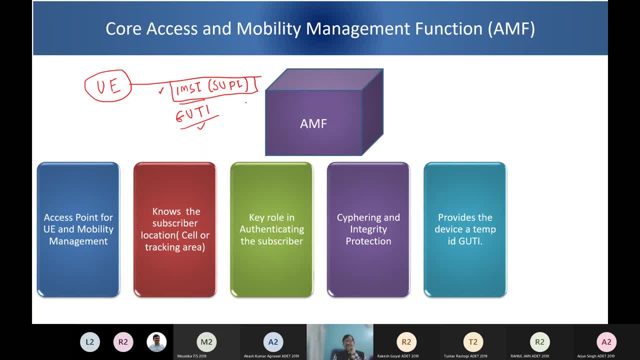 These are encrypted And then only it is sent on the air interface and encrypted one is known as SUKI Subscription, Concealed ID, Right, Right, So many new terminology: SUPI, SUKI, GUTI, Right So GUTI is Globally Unique Temporary ID. 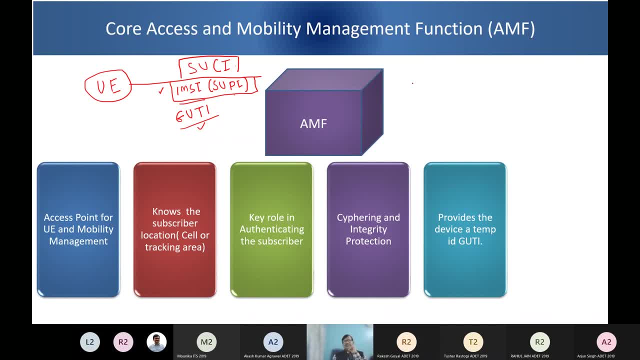 So what happens? that AMF creates a table of SUPI and GUTI. Right. So AMF, when it allocates a temporary ID to a user equipment, it creates a table of SUPI and GUTI. GUTI is your, just like IMSI. 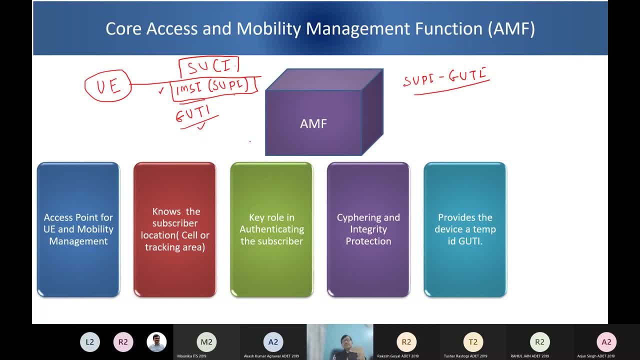 Just consider IMSI and GUTI, And whenever UE is trying to send a GUTI instead of SUPI, it knows that which SUPI it has Its identity AMF already knows because it has created a table, So it provides a Globally Unique Temporary ID. 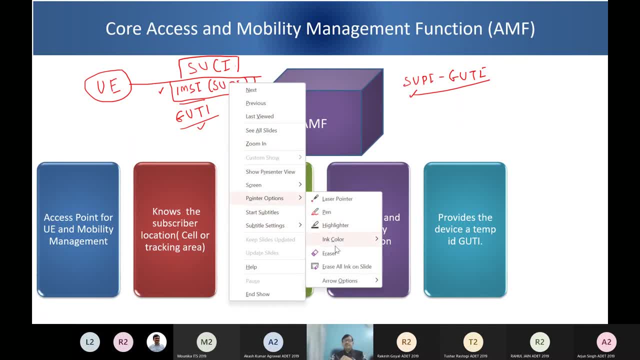 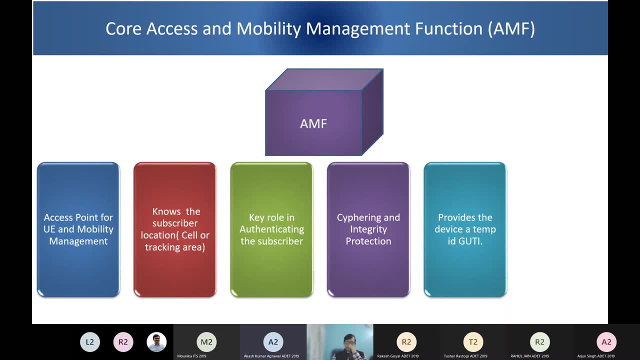 Any doubt on this? It is very important. Any doubt on Sir. why is there need to, Sir? why is there a need to provide a temporary identity? I mean, if the IMSI or SUPI, whatever you call it, if it is encrypted, if it is transmitted. 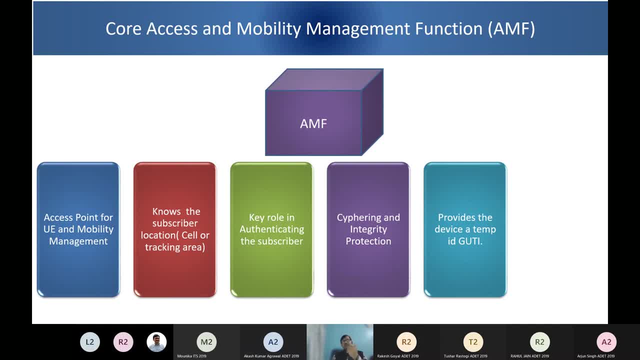 in encrypted manner. You are very right, You are very right. So most vulnerable portion of the network is the radio interface, Right Yeah, And if somebody is able to somehow know the identity of a user equipment, For example, if you are able to somehow know the identity of a user equipment, you will. 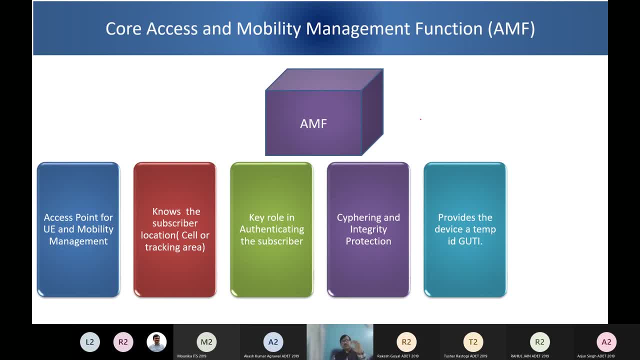 be able to create a fake UE. So to avoid, I mean so even we are kind of concealing the ID and sending onto the 5G network. But we also do not want to reveal that because if somebody has the key it can kind of decrypt. 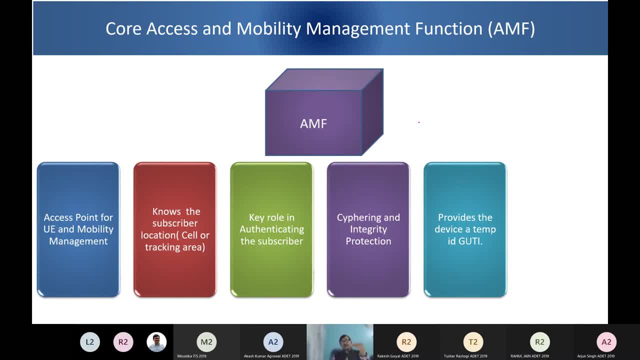 and have it right somehow. But we use temporary ID. So only for the initial access. we use SUKI. that is also encrypted. But at all other location- I mean occasion- we are using the GUTI on air interface So that if somebody is even able to kind of intercept GUTI, decrypt GUTI, it will not. 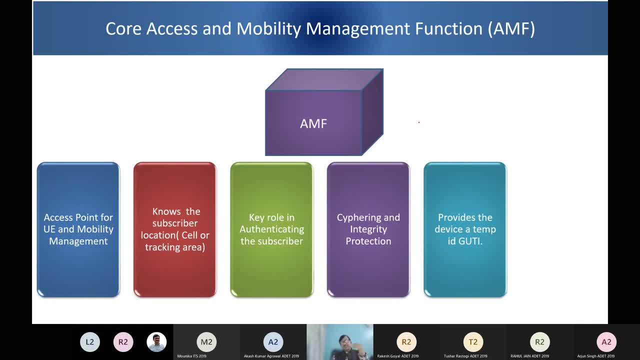 come to know the real identity of the user equipment. That is number one. And that GUTI is also not permanent, in the sense that for a particular UE, GUTI will changing, will keep changing. For example, whenever there is a mobility update, AMF will allocate a new GUTI. 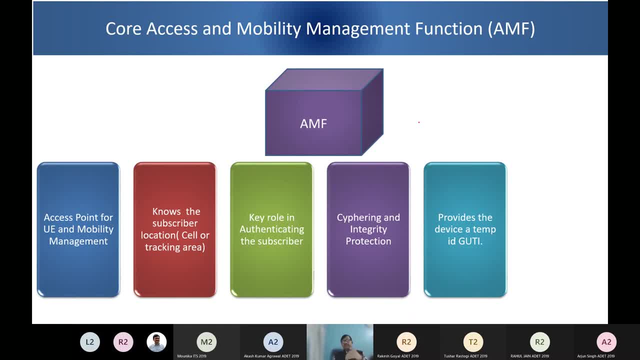 Whenever there is a periodic update, AMF will allocate a new GUTI. So GUTI is also changing. So just to keep the identity as private as possible, These aspects are being done. So now, somebody was trying to ask question. 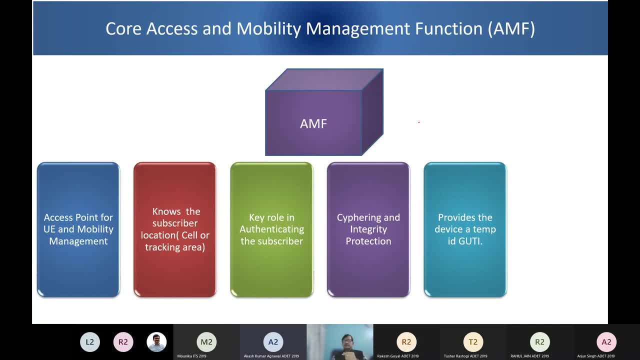 Yes, But whenever a new SIM card is issued- either SIM card or maybe eSIM, iSIM, whatever you can call it- So the network, the operator or the network, it provides a set of keys to that particular device, right? 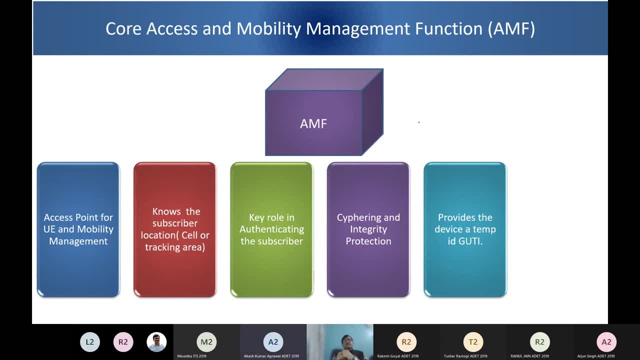 Device, or you can say SIM And using that key, only that communication is happening. Now, if it cannot be- I mean impersonated by another, some rogue device- then what is the need of doing? much more encryption than that. I mean using this temporary ID. 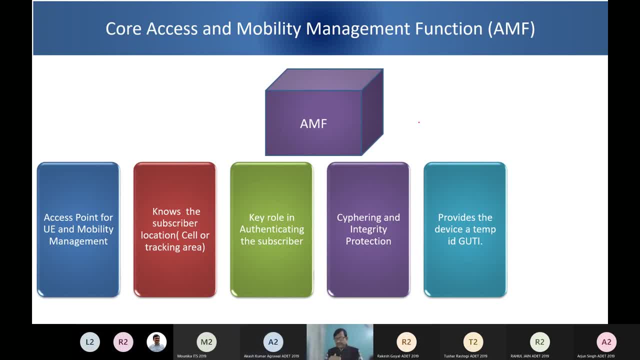 So you should Akash, you should consider these as layer of securities being built, right? So these are various layer of security, right? So one layer, two layer, three layer, four layer, Even if there is breach happening on one layer, I mean he will not be able to reach. 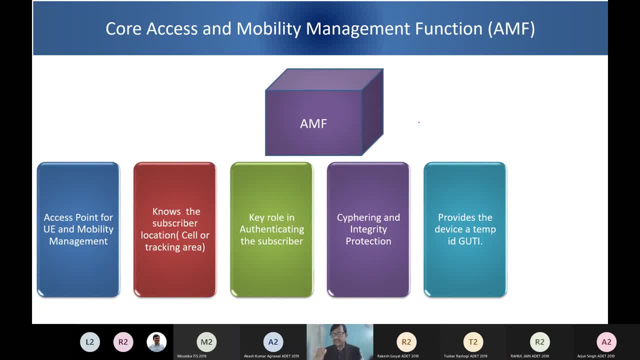 through the second layer and third layer and fourth layer. So these are various layers. So those keys which we are talking about is used for integrity protection, For example, if the keys- same keys- are provisioned in UV and the same key are there on other. 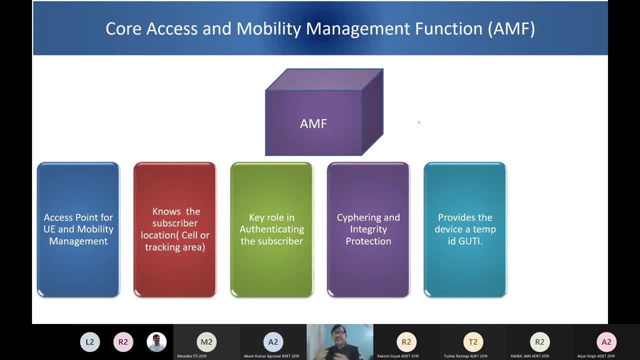 side. keys are not exchanged but some kind of hashing. we do it and send it And through a challenge, and then we receive and we kind of open by the key and see whether the same token which I sent has come. So this is for integrity protection, in the sense that UV knows that it is interacting. 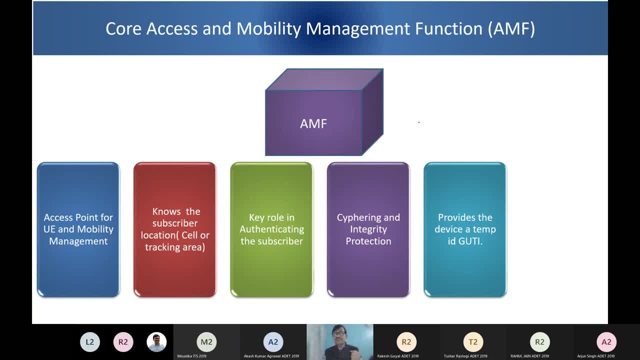 with the right network and network knows that it is interacting with the right user equipment. So there are. these are the authentication mechanism, We call it 5G, Akka, And in addition, the user access Identity is its MC or other other other soupies variables. 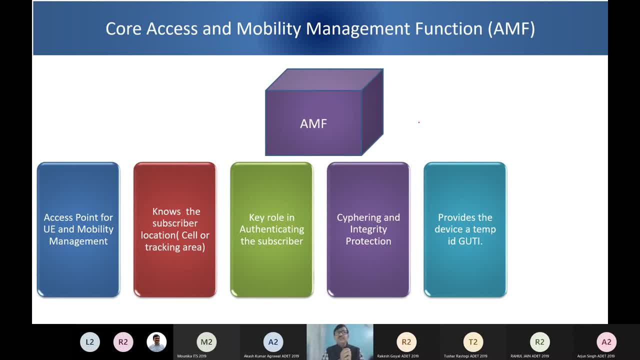 So that is also to be kept secret And that's why when encryption is done, that decryption is not even done by EMF, It is the corresponding private key is with UDM right. So that's why I said EMF plays a key role in authentication, because it also it may 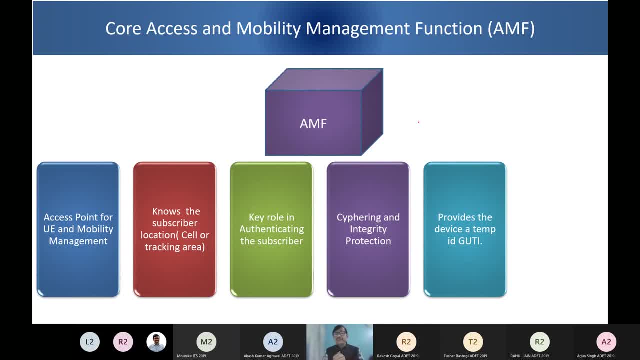 not be able to decrypt A Suki which is coming into soupy. So it it goes to UDM which has a private key corresponding. It decrypts and then tells EMF that yes, this is the soupy right. 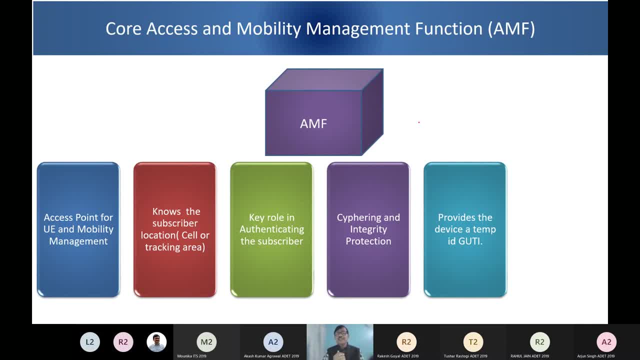 So that then it it creates a table of soupy and Gooty and allocate Gooty to the user equipment. So there are layers of security built in. Is that? I think there may be the reason that this may be the reason behind the physical 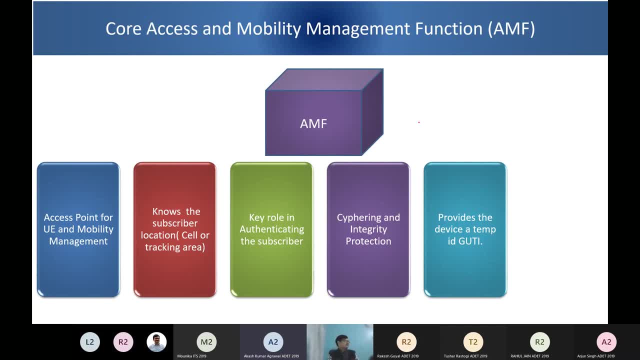 sync, Because if anybody can get access to a physical SIM and then he copies those keys, then multiple sessions can be created using the same key right. So in order to avoid such a- I mean such kind of a breach, maybe there's a temporary. 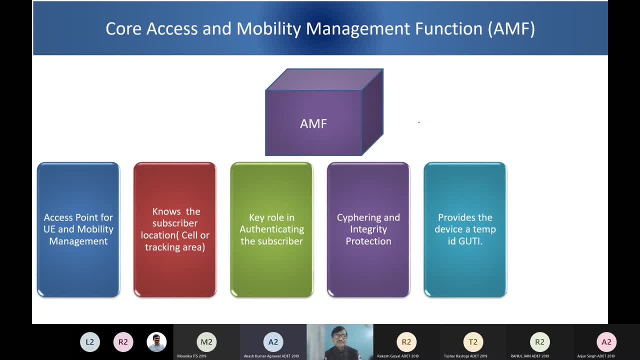 identity. I mean, I don't know, I just came to my mind because a physical SIM can be. I mean, so we are having a session on SIM. I ID me itself, So today confirmed. So Germany, somebody will be taking the session. 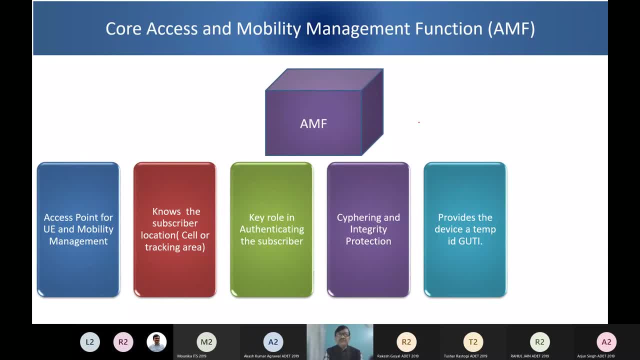 So so many, many security protocols are used inside the SIM and he will take one hour session, So I hope the technicality inside would be covered there. So let us learn that aspect in that session, right, Yeah, Okay. 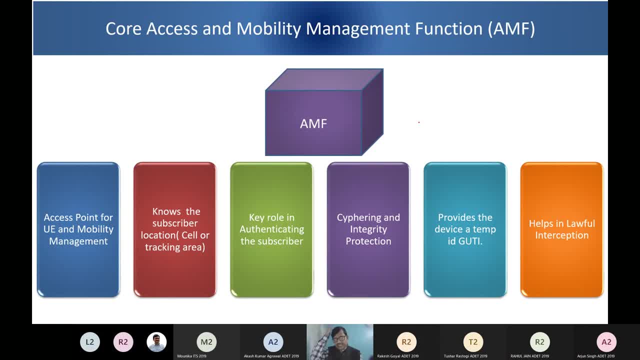 Okay, And the finally, since AMF knows location and various metadata, so it also helps in lawful interception and access point of AMF is again kind of AMF. I mean access point for UE is AMF, So the interception, it plays a role in a lawful interception which we have. 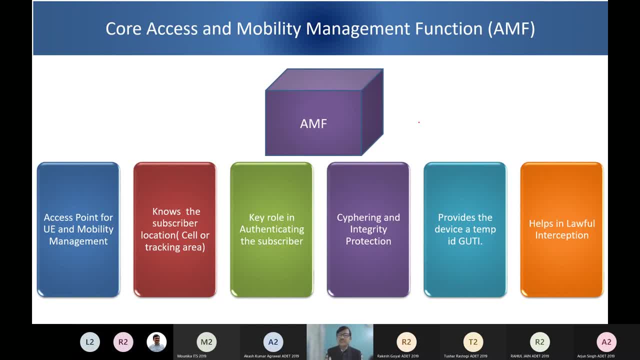 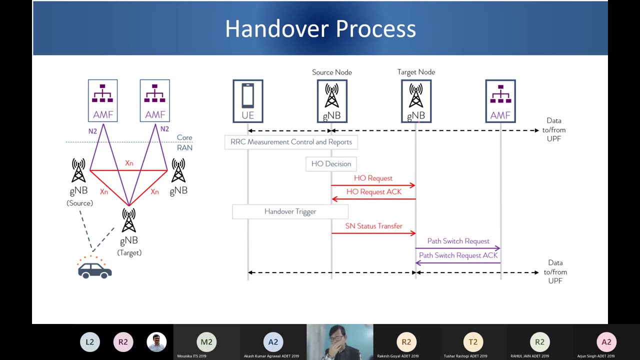 So, just see, we we were able to cover only one network function function, that is, AMF, and we took almost one hour, more than an hour. ok, let's, let's look at a very, very brief handover process, because AMF also does mobility management, so just. 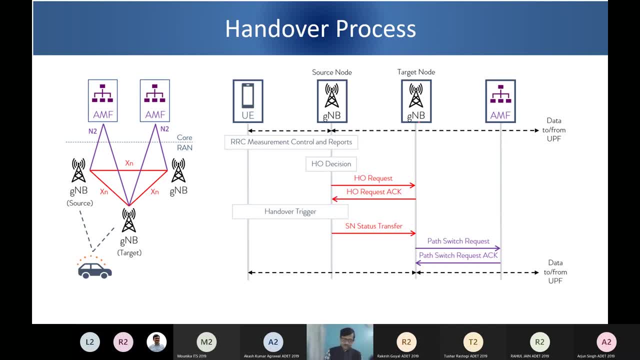 see this an example in a very, very simple way. so suppose this is your user equipment. this is your user equipment, which is, say, a vehicle, or say an user is sitting in the vehicle and it is being served by this g node b. so we are calling this as a source, g node b, right? 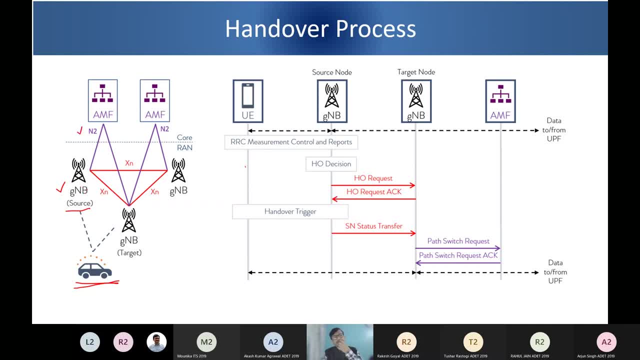 and being handled by, say this, AMF. now there are other g node b in the area. so when vehicle is moving what it does, it measures the signal being received from all other g node b nearby right. it measures and it kind of reports the measurement to the connected g node b where it has, I mean g node b which is the source g node b for. 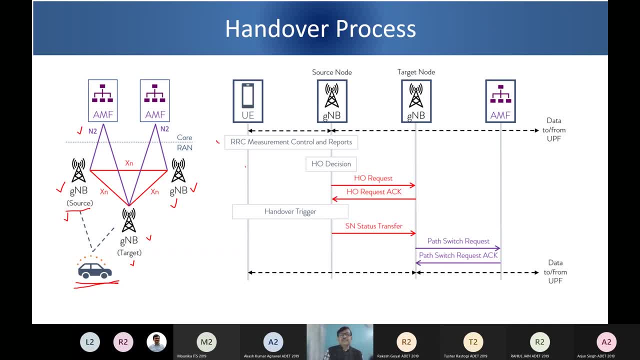 it. so this we call it RRC: measurement, control and report. so it is basically measuring the signal quality, signal level etc. and reporting to this g node b. Now the source g node b is the source g node b. The source g node b is kind of seeing these parameters and decides whether now it has. 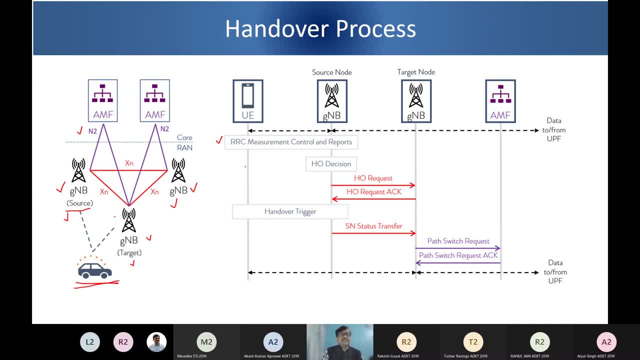 to handover to the next g node b. so when the signal quality, signal level etc. is much better compared to the source one, so it takes a decision, we call it handover decision. so source g node b is taking a handover decision, right, so they have an interface. 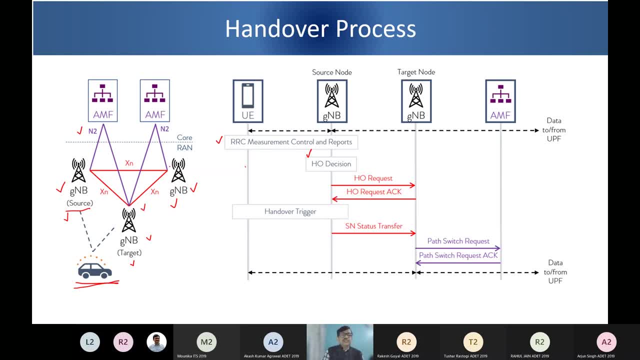 So they have an interface with all other g node b, xn interface, we call it so. on to that this handover will take place, and of course the AMF controls it. so now, if suppose this g node b is, say, connected to this AMF, right, so here even the AMF transfer will also take place. so once this g node b has 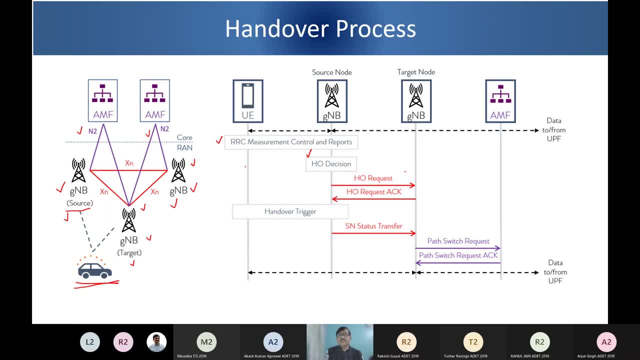 taken a decision of handover, It will ask the target g, node b for a handover. so request and acknowledgement will happen and then handover will be triggered. so the- I mean all the context- will be transferred to the next g node b and also to the next AMF if AMF is changing. if it is not changing, 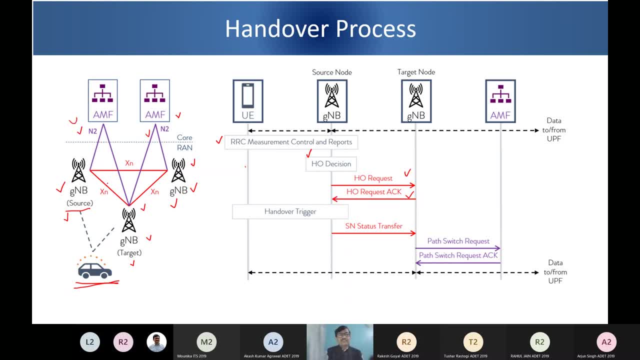 then this AMF will remain. so what is required is the path change. we have understood about the PDU session which is coming from g node b. Now the path change is happening That instead of this g node b now, traffic will come from this g node b, so this g node. 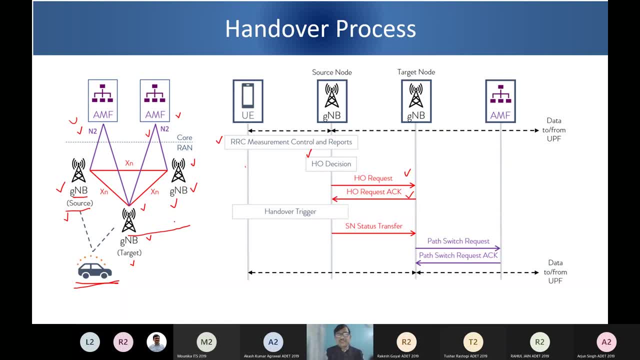 b may have a physical connection right, physical backhaul onto the core network. so path switch is happening. so path switch request that AMF takes that decision and then path switch acknowledgement and finally data goes to the UPF through other g node b now. so this is a very, very high level. 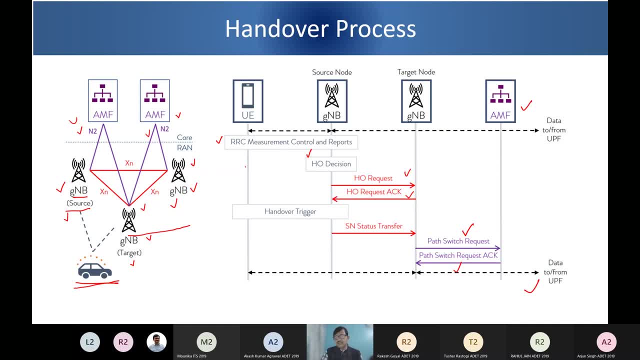 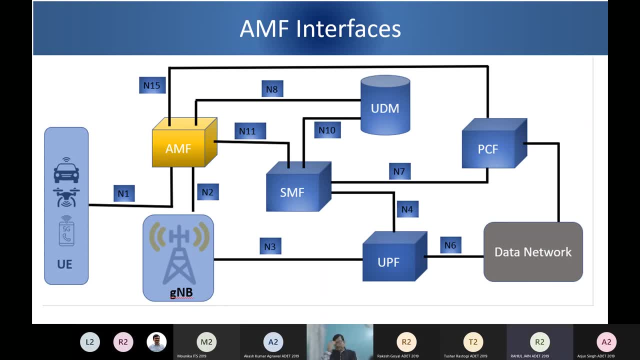 of handover process for inter-g node b. okay, so now we have a. yes, Sir, as in 2G, when the other base station signal goes beyond a certain limit of that we are receiving from previous one, then handover occurs. so is that the same procedure followed? 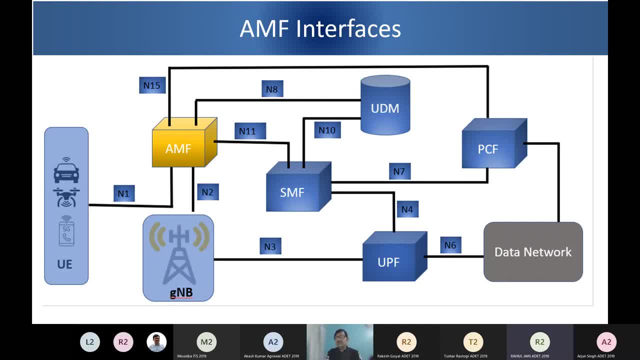 in this You are addressing it significantly high. you should see me, you should say it's similar. yes, you should say it's similar. so exact procedure may vary, but it is concept wise it is similar. now let us talk about various interfaces which amf would be having. so just see what are the 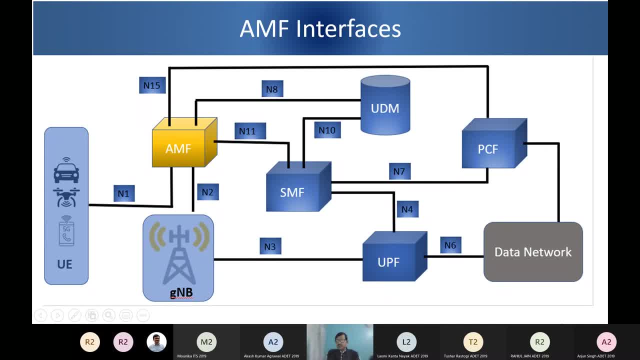 interfaces. so what is the interface with the user equipment? just tell me that. what is the name of the interface? and one and one and one. so all those signaling. we call it nas, i think uh, gbg sunil sir was explaining this, as is what access stratum? so this is non-access stratum kind of a signaling. 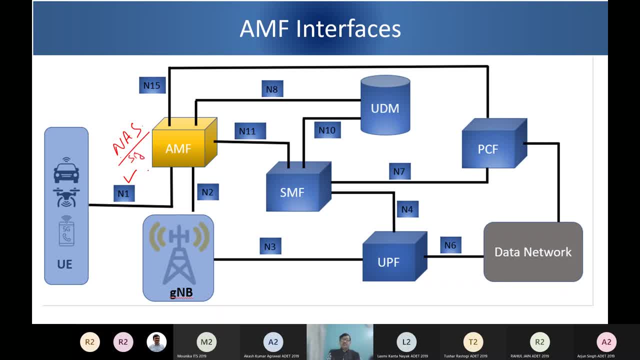 right, which is signaling is happening between ue and the core network and g node. of course traffic comes from g node b. g node b is kind of a transparent here. so n1 interface is for nas signaling between ue and the mf. now all those mobility management and all 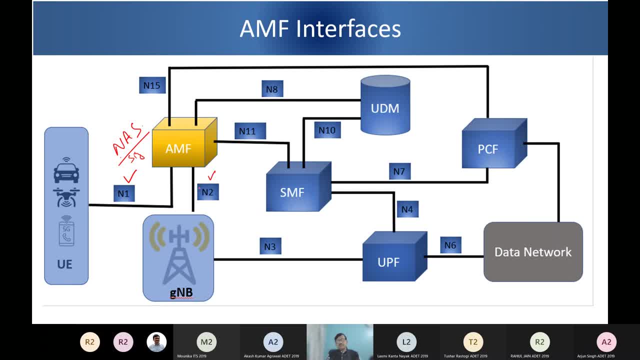 is on n2 interface. amf controls the mobility and amf has to consult udm because the subscriber data will be there in the unified data management. even the data network profile will be here. so it has to consult which user to be allowed a particular service or not. so it has to access udm and then uh policy control functions. 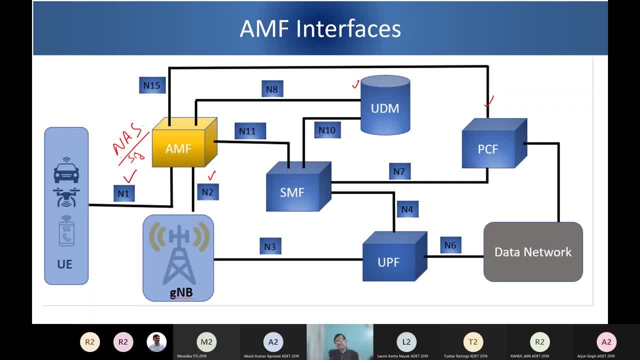 so it also talks to policy control functions, because policy related decisions are taken by pcf, so it also uses pcf services. on n15 interface. i would request that you should try to remember these interfaces. okay, now let us look at the n15 interface. now let us look at the n15 interface. 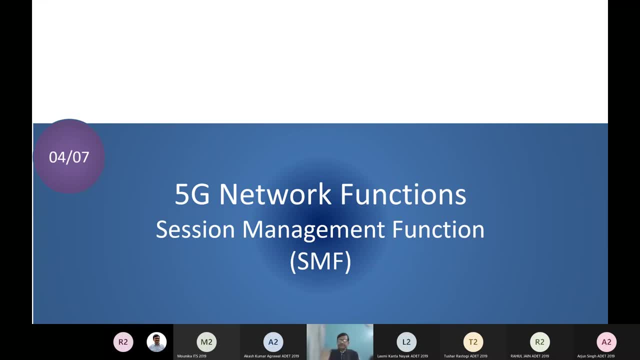 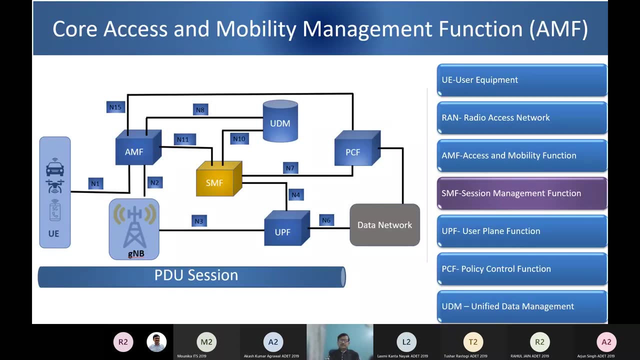 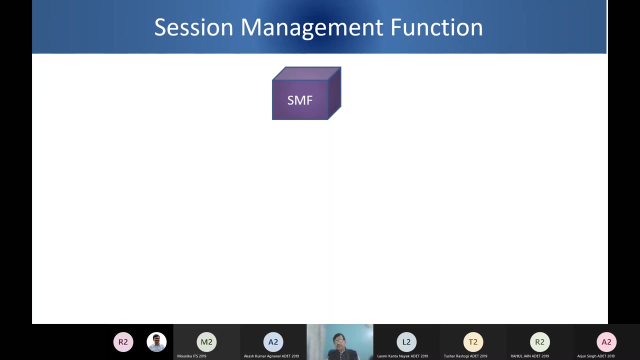 now let us look at the next network function, which is smf. smf is your session management function. just see where it is located. it has also got interfaces with amf, udm, pcf, upf. we will talk about that, okay, so, as the name suggests. so before i uh tell you the functions, let uh can somebody? 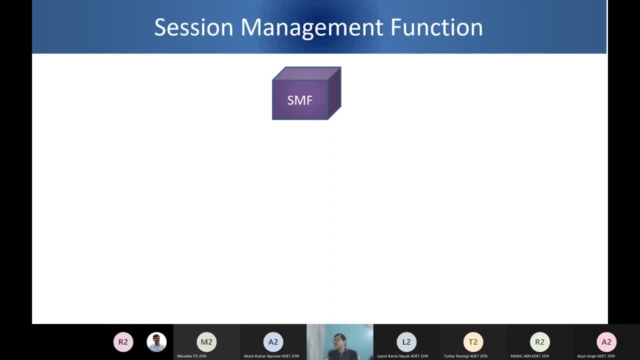 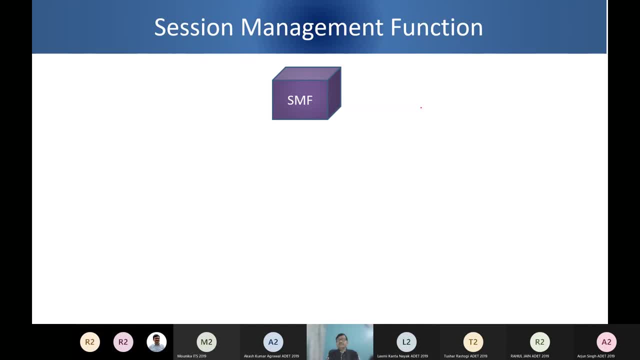 so what is the equivalent network function of smf in 4g? Is it STW? I'm not sure. No problem, Monica. Yes sir, Did you hear my question or should I repeat? No sir, Can you please repeat it, sir, please? 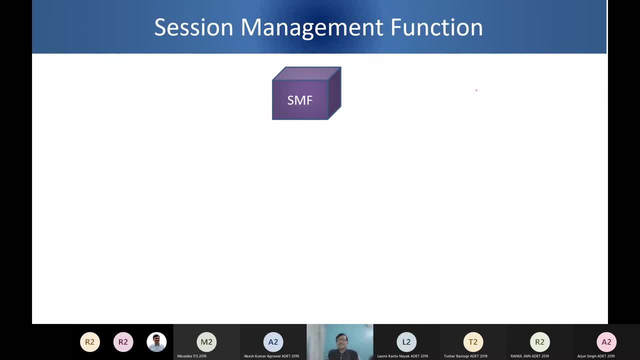 My question is: what is the equivalent network function of this SMF In 4G? Yeah Session. Okay, Rahul Chauhan. Sir, it might be MME only. So Akash have answered right. So basically, mobility management entity in 4G was split. 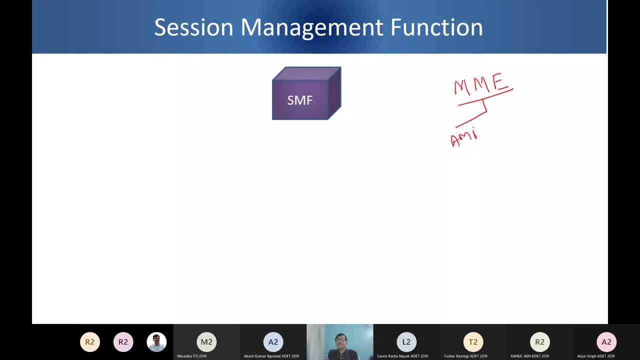 Split into two parts, one in 5G, AMF and then SMF, right, So session management function and AMF function in 4G was being done by MME itself. Okay, So, as the name suggests, what could be various functions of SMF? 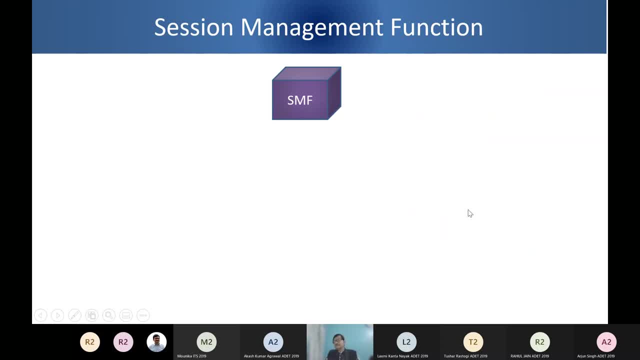 Any one of you Do you recall I talked about PDU session. Yes, sir, We need to establish and maintain a PDU session. Yes, So the creation of a PDU session, modification of a PDU session, termination of a PDU session. for that instruction is given by SMF. 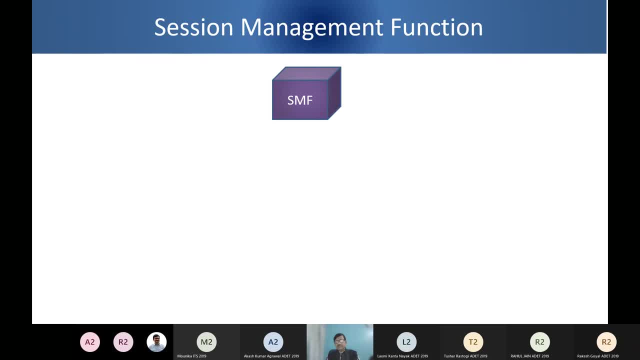 I mean SMF does that? I mean instruct all the relevant network functions below in user plane to create. So basically Creation, modification and deletion of PDU session. So session management is done by SMF. What is the next function? 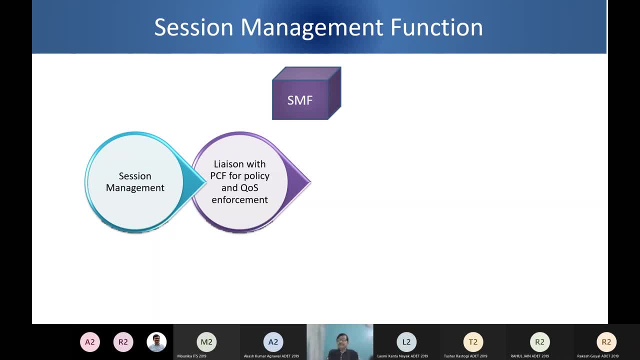 So the next function of SMF is about quality of service. Quality of service- Yeah, Just a moment. Yeah, So quality of service. So can somebody guess what SMF will do in terms of quality of service? Any guess? 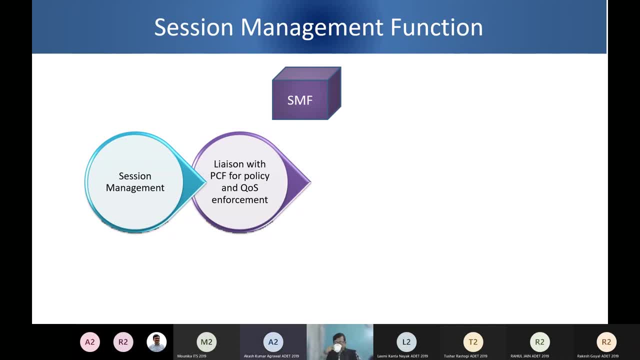 Akash: Yes, It will assign a particular QoS. It will assign a particular QoS to a particular PDU session and it will- I mean it will make sure that QoS, I mean that QoS is enforced, Just like slides. 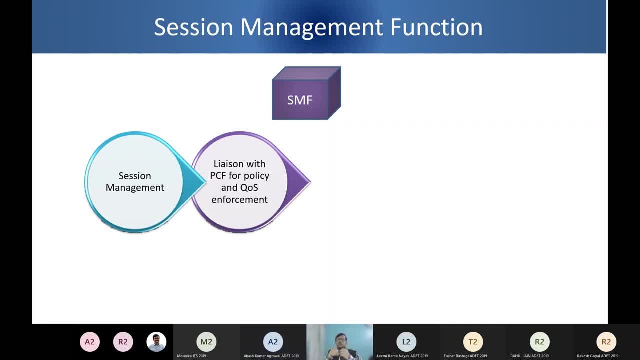 Yeah, right, So you are right. So basically, if you look at SMF, it gets- we call it- PCC rule from PCF policy control function. There is a network function called PCF, So it lies in with PCF and gets PCC rule against that particular user which want to access a particular service. 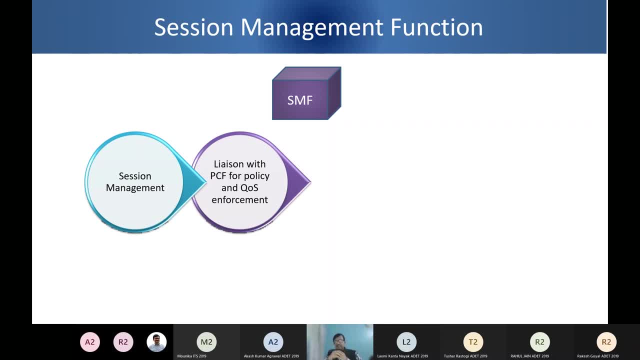 So the PCC rule which it gets it uses to enforce quality of service onto the PDU session. So it is not independent for doing all these aspects because it has to lie in with PCF for PCC. So it is not independent for doing all these aspects because it has to lie in with PCC rule. 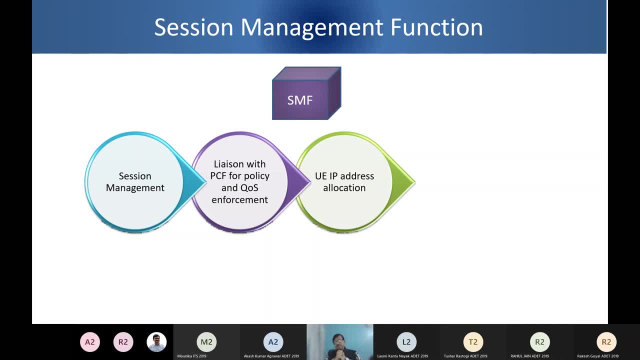 What exactly QoS flow to be applied Now? the next function of SMF is that if I am saying if the traffic is an IP traffic, it will get IP address. My question here is that: why I am saying if? Why I am saying if? 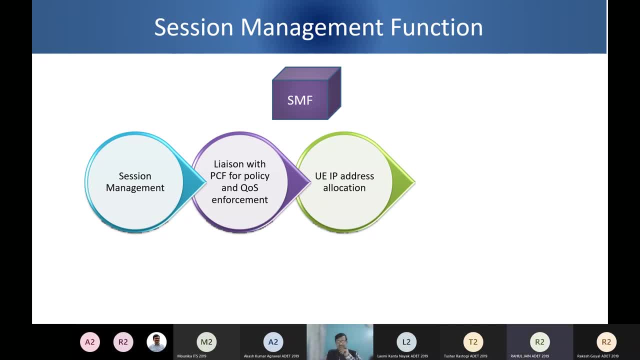 Sir, you said all the traffic is not IP traffic. Yes, All the traffic is not IP traffic and hence only if this is an IP traffic it allocates an IP address. Otherwise, for a say, structured data, no IP address is required. 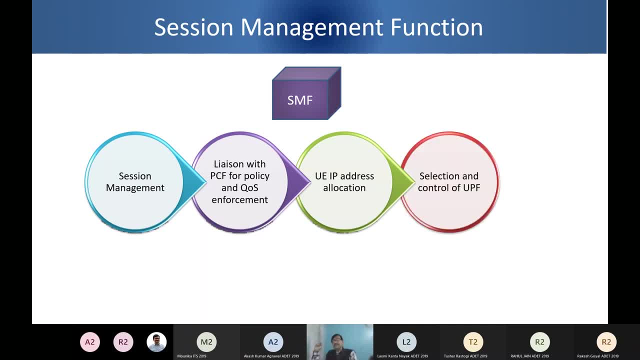 And this is the difference, One of the difference from 4G. Now we know that PDU session, the user plane part, is from UE to GNB, to UPF and then to the data network. So one of the responsibility of SMF to select and control a right UPF right. 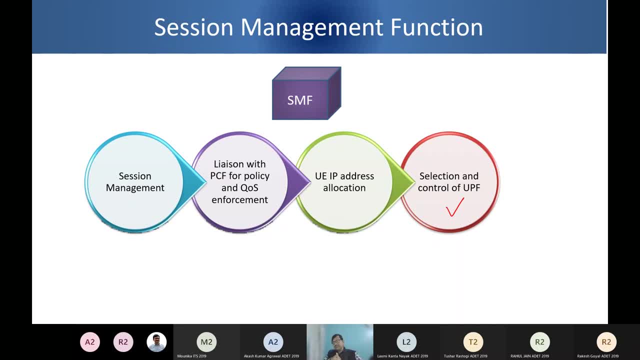 Why I am saying right UPF. Can it not select any UPF and serve the user? Or it has to select the right UPF. When I say right UPF, what I mean by that? Select the proper GNB which is having good signal strength. 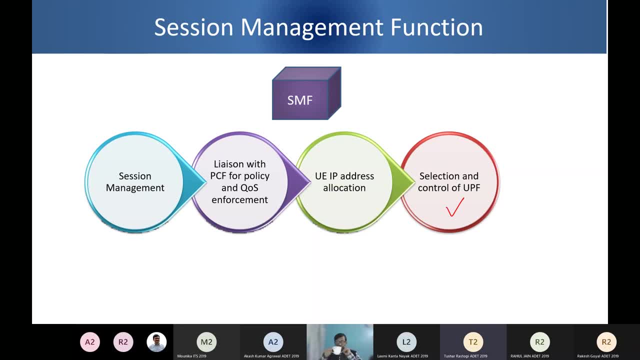 Why I need to select the right UPF, Sir? because since different QoS parameters have been decided for PDU session, So whether resources are available in that particular UPF or not, For that it has to see which UPF can specially reach to that. 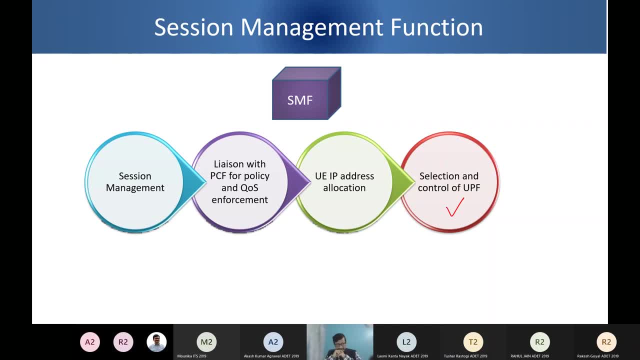 Ok. So, sir, let me tell you something else. For example, suppose you, as a small startup, Is running the gaming service in Bhopal, Right? So you are connected to a 5G network on a particular UPF. 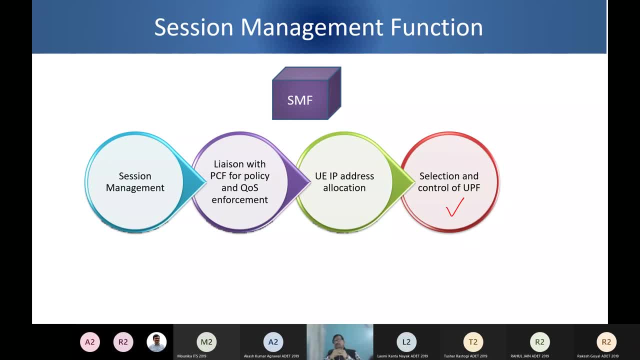 which is located in Bhopal, in Bhopal right, Suppose a user wants to access your service, then which UPF SMF should select? The UPF which is connected to your service, Tushar, Yes, sir, So that's why. 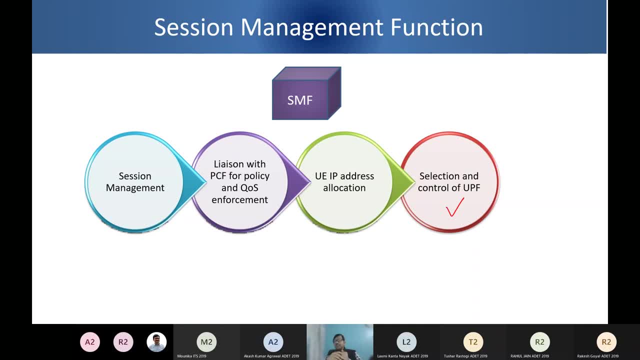 I am saying it has to select and control a right UPF. So there may be multiple UPF connected to different data network or different applications and user accessing. if is trying to access a service which is handled by a particular UPF, then SMF has to select a particular UPF. 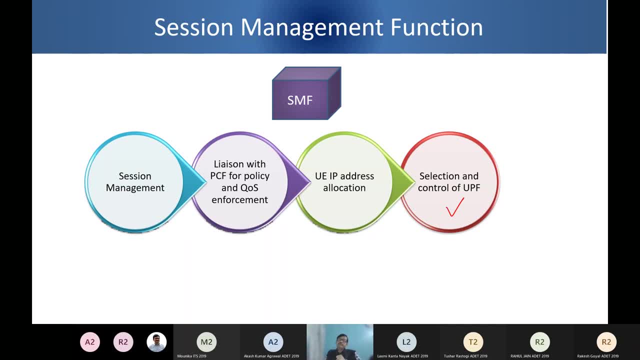 or at least an UPF which is connected to the other UPF. Okay, sir, Okay. And the next is about quality of service. There are some details which I will explain. So SMF in respect of quality of service, because it has to maintain a quality of service. 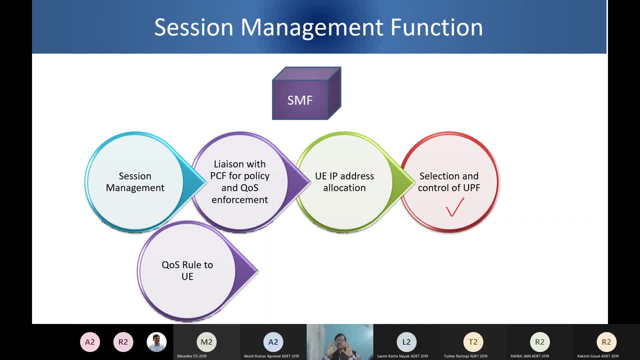 for a particular service. So it does create three things. One is called QoS rule- quality of service rule- which is sent to the user equipment because for uplink traffic it has to identify and map which QoS file is being sent to the user. So QoS is the quality of 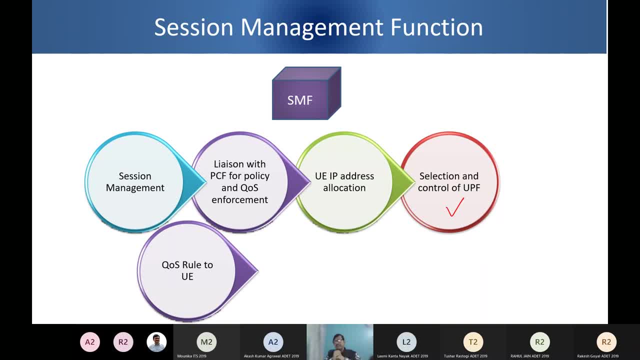 service which is sent to the user because for uplink traffic it is to be applied which quality of service ID QoS has to be applied. So basically, it filters the IP traffic and apply a QoS file. That filtering is done based on the QoS rule provided by SMF to the UV. 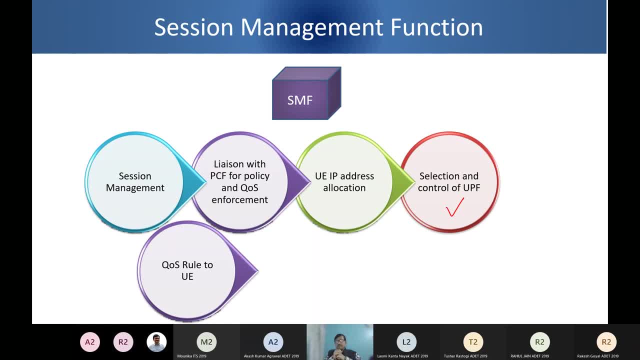 Am I audible? Yes, sir, Yes, sir, Okay, Okay, Okay, Okay. So the next, that was UE. Now the G node B, the radio resources. So the radio resources. lot of QS profiles are there which is to be managed. So which profile will be kind of? 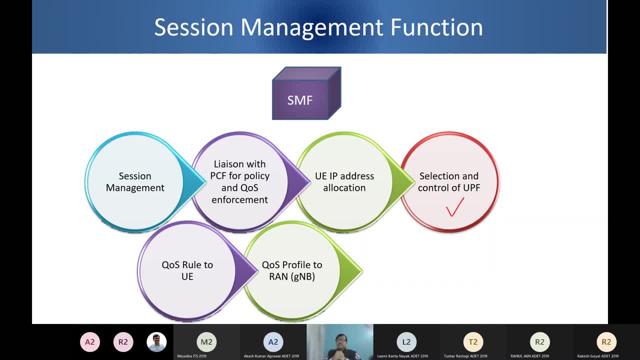 applied for a particular QS. that profile is given by SMF to the G node B right. So your 5QI or equivalent QCI in 4G goes to kind of a G node B And then on other side 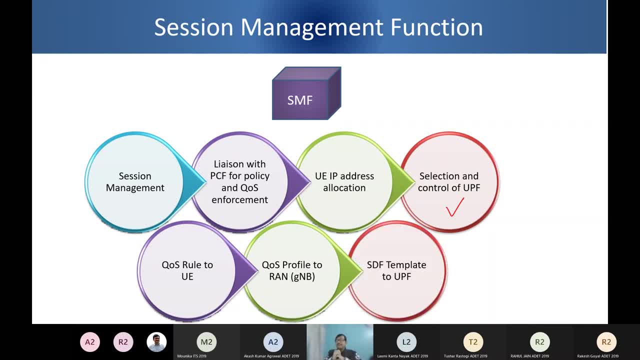 you have UPF, So there we provide. we call it SDF template. So three things just remember: QS rule to UE, QS profile to RAN and SDF template. this is also called PDU rule. PDU rule- packet data. 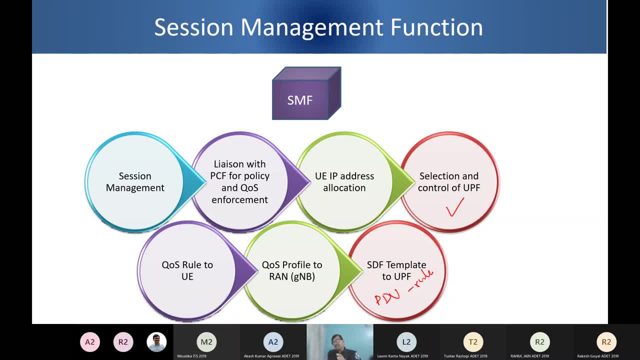 rule is applied to UE. This is also a kind of a filter. when traffic in, say, downlink directions are coming, it segregates into different bunch of IP flow and allocate a QFI- quality of service flow ID, depending upon what service it is, So that filtering is called, I mean. 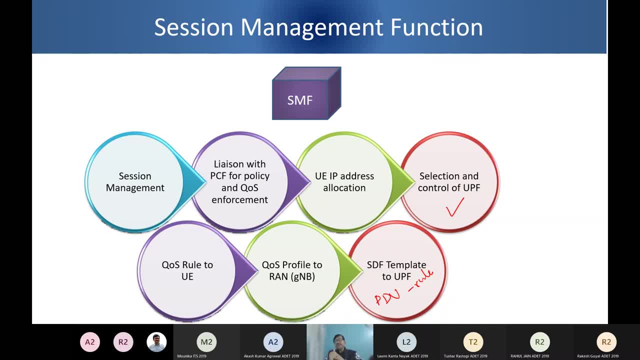 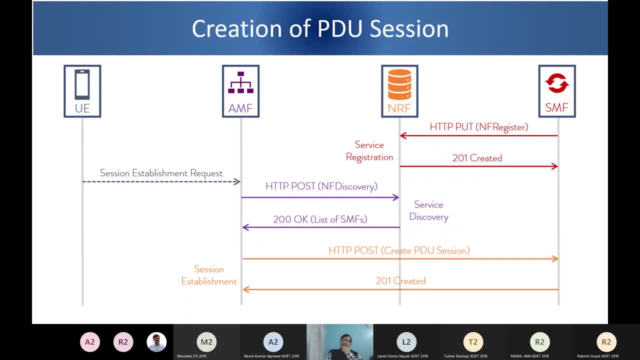 is done through SDF template or PDU rule provided by SMF. Okay So, guys, I would like to complete all the five network functions and then give a break. Is that okay? Yeah, So other network functions are small and, in the sense that happened, quickly, So let's. 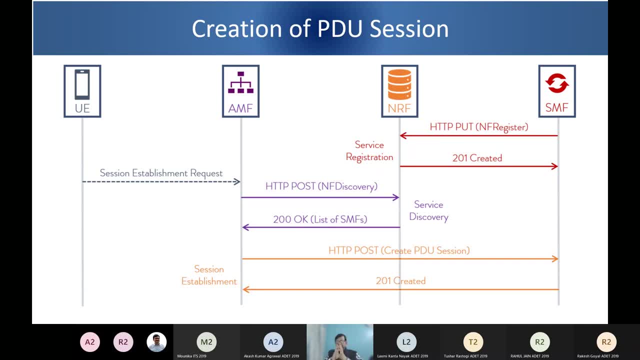 do and give you a break. So now let us look at how it works. So one network function which I have not talked about is called NRF Network Repository Functions. What it does is that whenever a new network function is created or modified, it has to register onto. 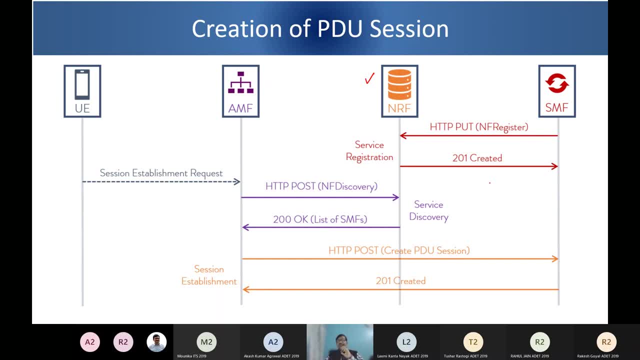 the NRF. So NRF will contain kind of information about all the network function. What are those information that can be profile of that? and also the address, either IP address or a fully qualified domain name, that is its address kind of right. So NRF knows each and every. 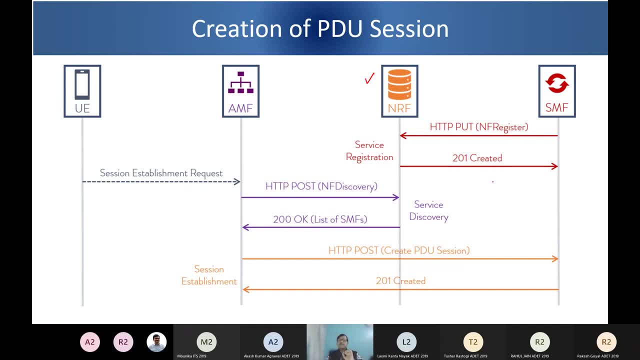 network functions and all its instances right, their profile and their location In this example suppose. yeah, please go ahead. Can you please repeat what is the network function? This is NRF You are talking about. like NRF has details of all the network functions and all its stances. 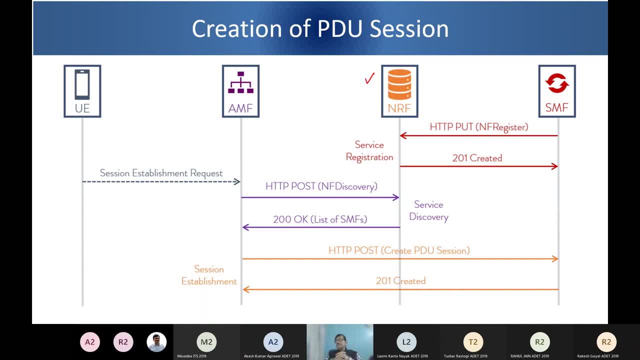 of it. So what do we mean exactly by the network function? I am not able to get it. So: network function. So AMF is your network function. access and mobility function is a network function. All these blocks are like network functions. 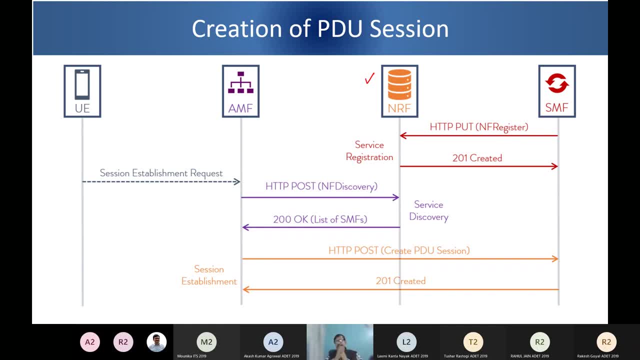 Right. So all are network functions right, Providing some kind of service in the control center. In addition to this question, you said whenever a new network function is added, so then NRF will be updated like this: So are the network function are? aren't these fixed, or they are? 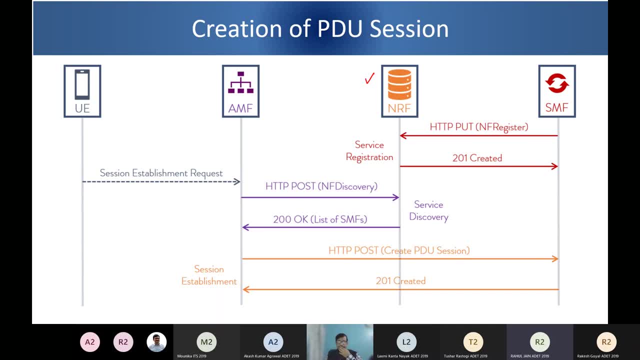 variable, like some network may have different number of network function. Yeah, Yeah, So it is. it is very, very flexible, Right, So you can have N number of different functions. Right, So it is. it is very, very flexible, right So you can have N number of service. 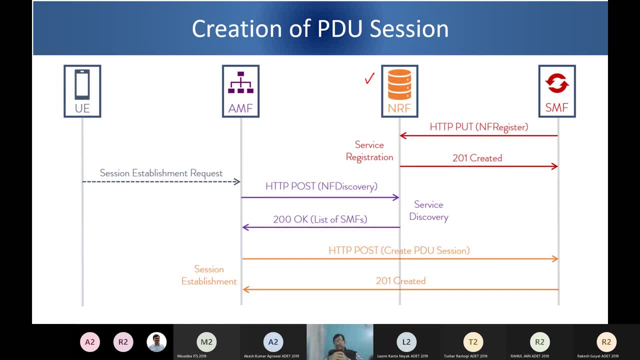 of amf instances, right. so suppose if your traffic is high then you have many amf instances working. as you grow, i mean day by day in a traffic, you have to add more number of amf, right? this amf has nothing but software pieces running on a cloud or net, uh, any, any hardware right. so once 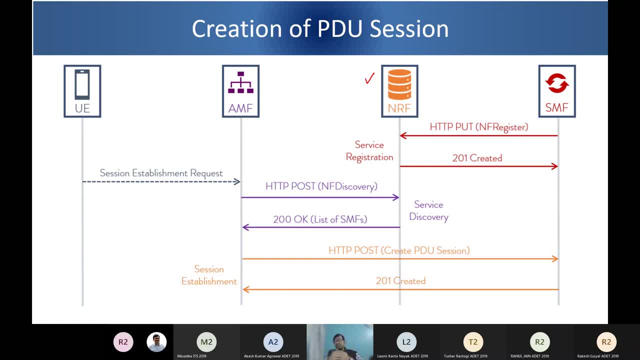 your traffic is growing, you need to add more and more instances of amf, right? so i meant, apart from this five, six network function, other network function may also be there or only these are there. so there are. there are 15, 16 network functions, so five i am trying to cover in this. 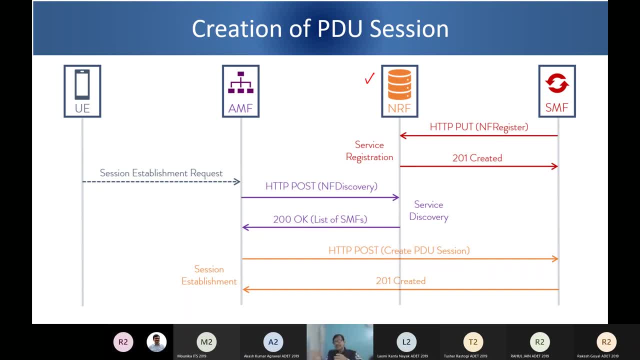 session and five i will be covering in the next session, i mean today itself, and five i'll be giving you assignment. okay, so major part again. i actually wanted to ask that in any network, are these all network functions? are number of these network function is fixed uh like different network function not uh like. 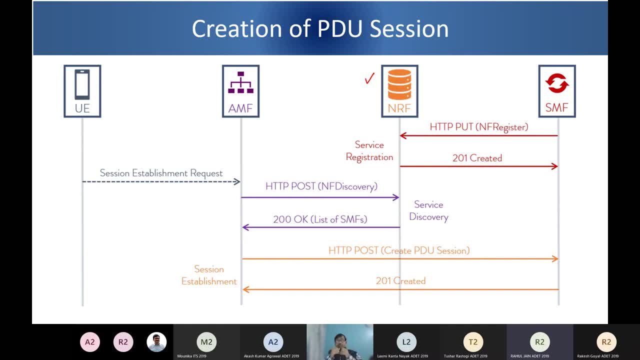 amf will be there and smf will be there another. so will this be fixed? these five network function which i am talking about are the building block and will be available in each 5g network. there are certain network functions which may be there or may not be there, for example i'll talk about. 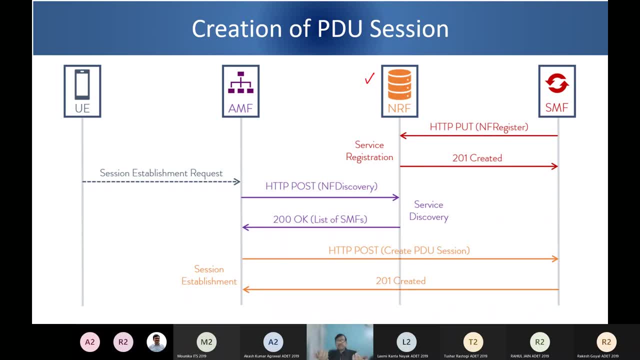 networks, slice selection function. so suppose, uh, if, if id network hypothetically is not using the slice function, right, so it may not require an ssf right. and suppose you are trying to create a private 5g network, so where billing charging is not a requirement for you, so those network functions. 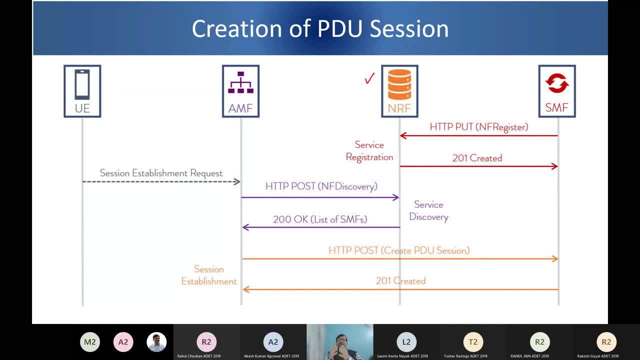 related to billing charging you may not be having in a private 5g network you may not require, uh, laughable interceptions, so network functions related to laughable interception you may not be deploying to depend. suppose it has also got sms function, so suppose you are not offering sms service. hypothetical, you need not deploy sms function. 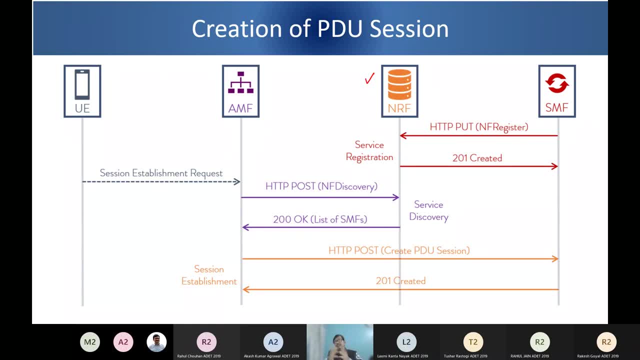 so, depending upon which service, which native service you want to actually offer, you will be putting the network function. so there are certain building block which is required for any kind of 5G network and there are certain network function for a specific service. Okay, sir, Understood. 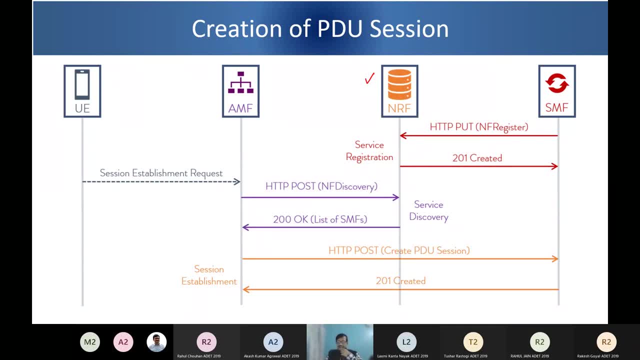 Okay, Good, So okay. So here, as I said, that all other network function, whenever they are installed they register onto NRF, So NRF will have address and profile of all network functions. So let us take an example that a new SMF is created, So it register onto the NRF and then it gives: 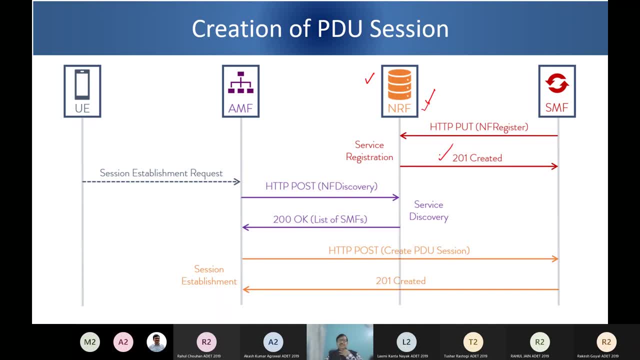 the acknowledgement that, yes, it has been created. Now let us take an example that a user equipment want to make a PDU session. a session establishment request is coming and that will come to AMF right, because the UE access to the core is with AMF only. So now AMF has to direct. 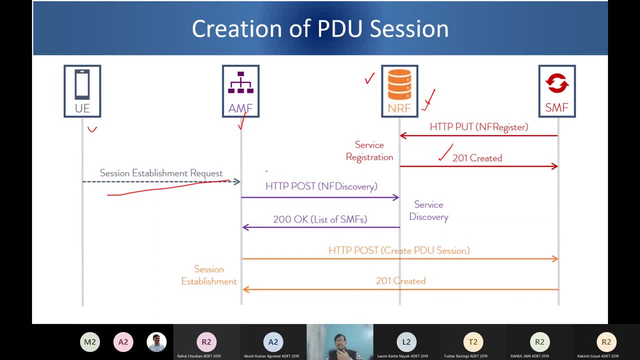 one of the SMFs Right. There may be many SMF in the network. So how to know how many SMF are there and which is the correct SMF? So it does a discovery. So NRF function is the discovery. So it. 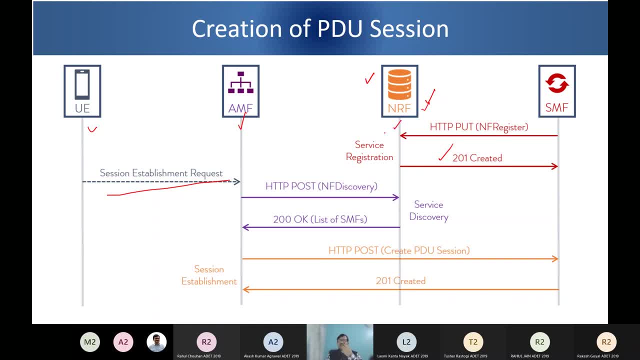 will trigger NRF, talk to NRF and say that tell me the list of all the SMF with their profile. So some kind of request will go and it will provide list of all SMF with their address And also their profile. AMF will choose the correct SMF reading the profile and the request. 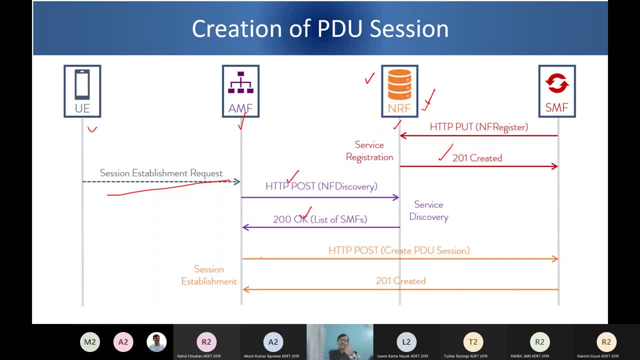 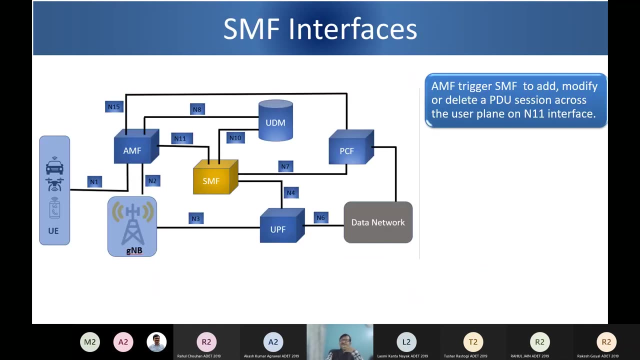 coming from the user And once that is done, then it instructs SMF to create a PDU session and SMF does that. So this is a kind of creation of PDU session, the role of SMF. Okay, So what are the interfaces of SMF? 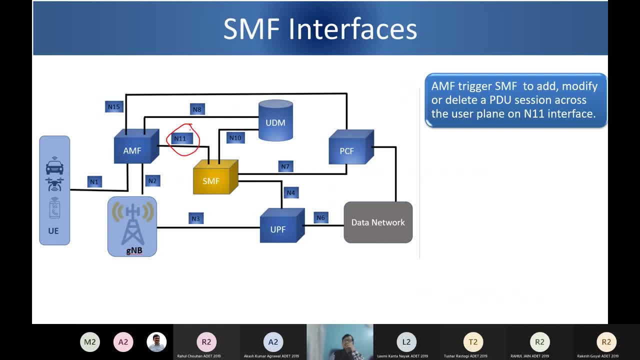 So now let me ask. it is also written that N11 interface is between SMF and AMF. Monica, tell me what is the purpose of this N11, one of the major purpose, Sir. once the user wants to start a session, then AMF will communicate SMFs to create that. 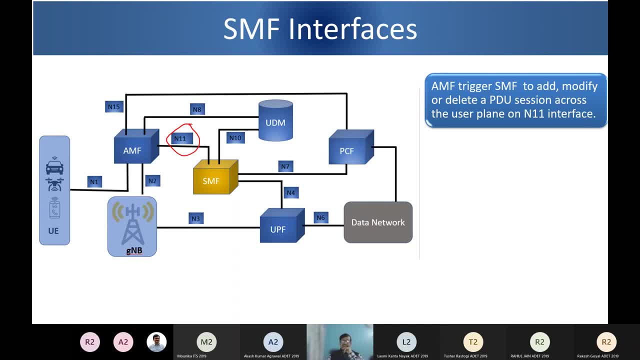 session. Yes, Yeah, AMF. instruct SMF to create a session on N11 interface, Now N7,. who is going to answer this N7 interface? Maybe Lakshmi? Yes, sir, So I was asking about N7 interface. 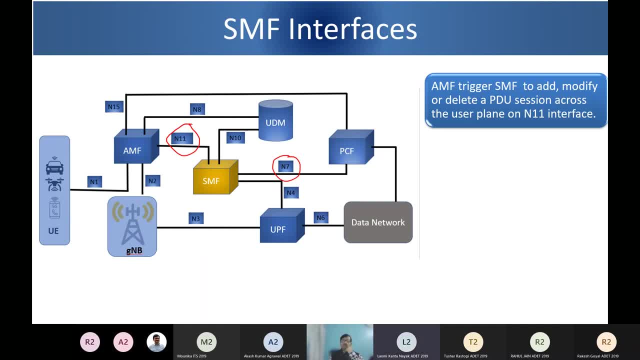 Yes, I just discussed. I discussed that SMF will receive PCC rule from PCF. That means policy related aspects or the instruction it receives from PCF. For that purpose we have N7 interface. Now somebody tell me the N10 interface. 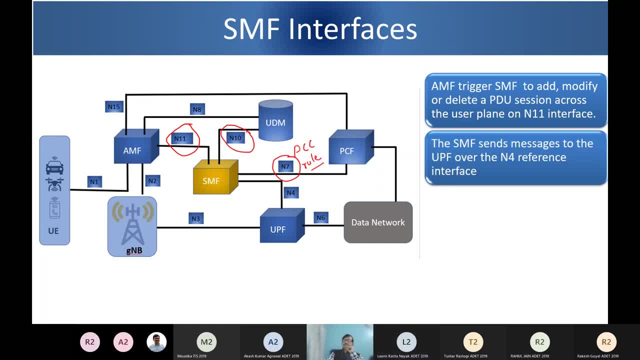 Okay, Then, and then QoS rules. It will authenticate the subscriber based on the subscriber information stored in indie. so authentication is already over. then only amf is asking SMF to create a session. It is just a subscriber profile which SMF wants from UDM. so that correct kind of QoS. 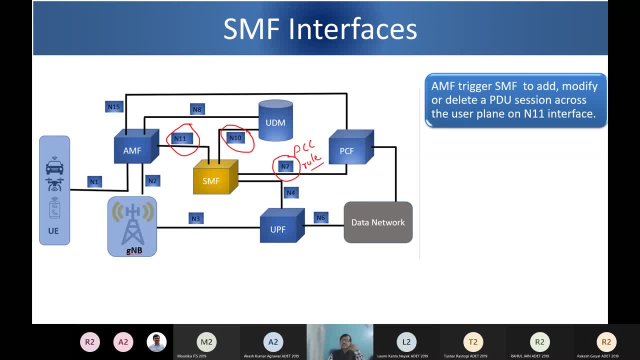 whether a particular service which trying to access is actually subscribed by the customer or not. So it is to access MF issuer- Yeah, exactly, the subscriber profile and data network profile. And what about N4? Between SMF and UPF maybe? 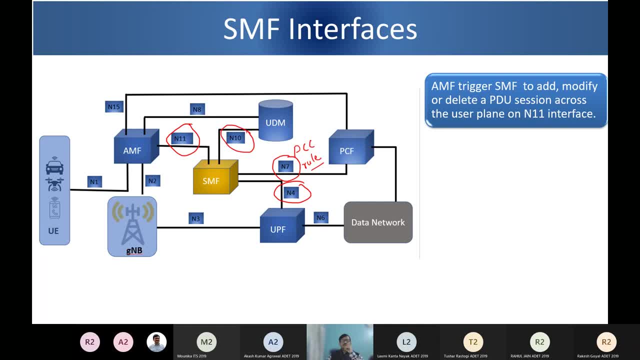 Rakesh Goel. So maybe the QoS? Yeah, So PDO session has to be created here right in the user plane That is, between UEG NodeB and UPF. So actual user plane has to be created by UPF. 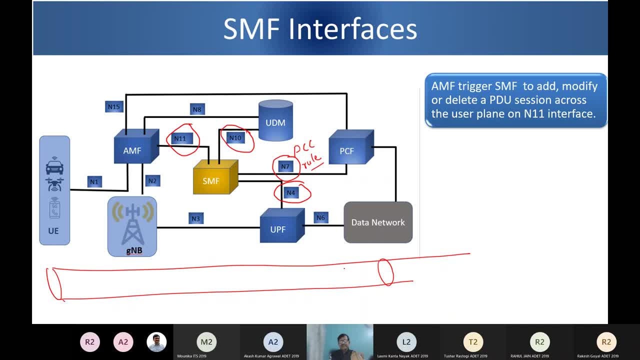 itself right And QoS flow is also to be managed by UPF. So SMF instruct: first of all it has to select an UPF, write UPF and also ask UPF to ensure the quality of service what it is telling. 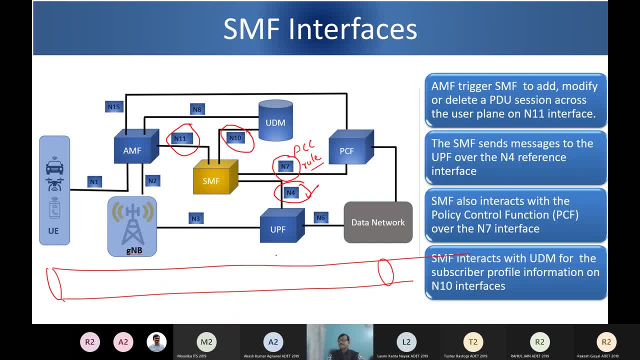 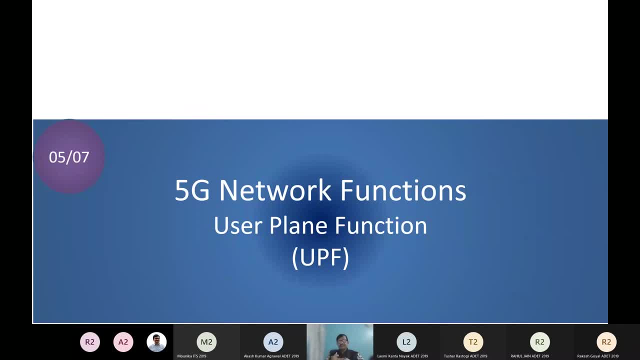 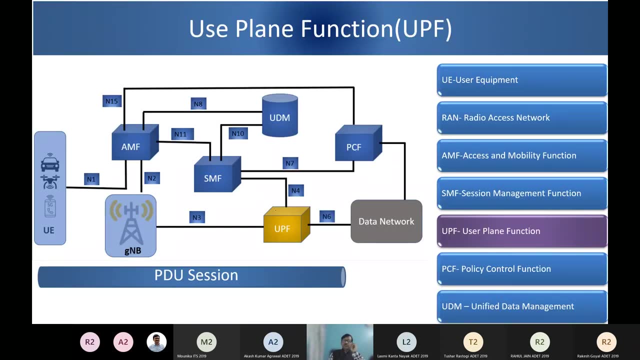 Is that okay? Yes, Okay. Now the next network function is user plane function. So I think we have already covered this somehow. So user plane function is in the user plane itself. It is part of the PDO session. So PDO session flows through UPF, UEG, NodeB, UPF and then to 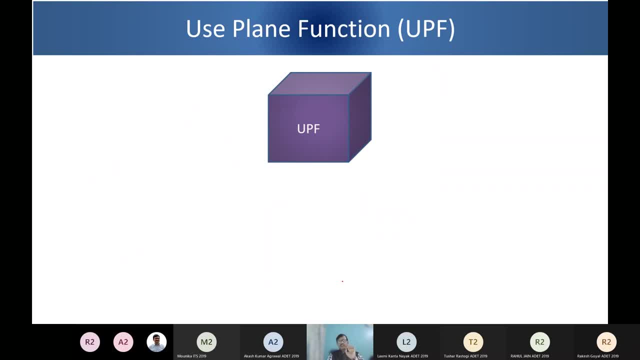 the data networks. So it is right sitting into the user plane. So that means the actual data forwarding, etcetera will be done by UPF. Now tell me when a user equipment is moving from- suppose this is a UEG- from one gNodeB to other gNodeB, right From this area. it is coming to this area, So your gNodeB is changing. So, for example, this is going to the user plane, This is going to the user plane And in this case, the data network will beUBF suдержined. 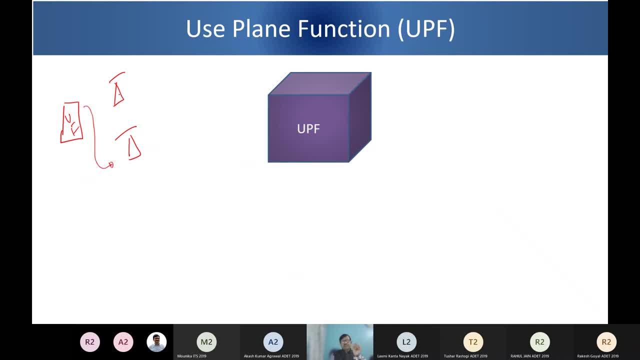 that related to良用. cecraft is going to the part of the code 구, changing from, say, g node b 1 to g node b 2. what is remaining common? can somebody tell me that? what is remaining, which is same as earlier, even if a? uv is moving from one g node b to other g node b? 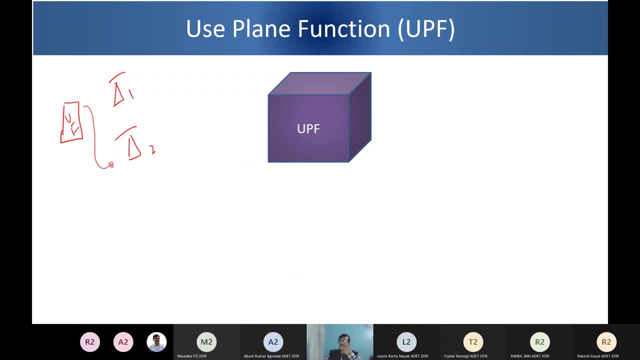 registration: yes, the registration area, no, i'm telling about you, tell me, the network function, amf, amf. so amf is not in user plane, right? i'm talking about the user plane traffic, one g node b. it has moved to the other g node b so as as we discussed that. 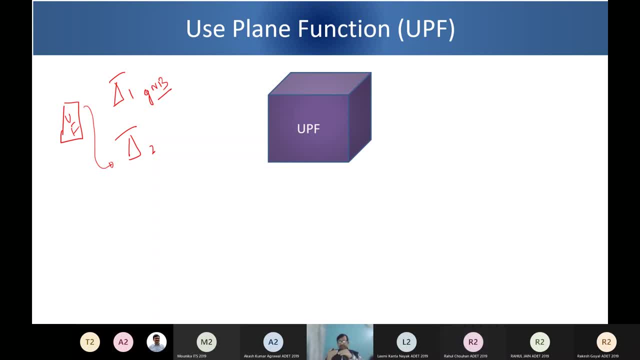 the- i mean the path change is happening. your predu session, which was from g node b 1 now is through g node b 2, right, but which network function is the g node b 2, right? so amf is not in user plane, right? i'm talking about the user plane. 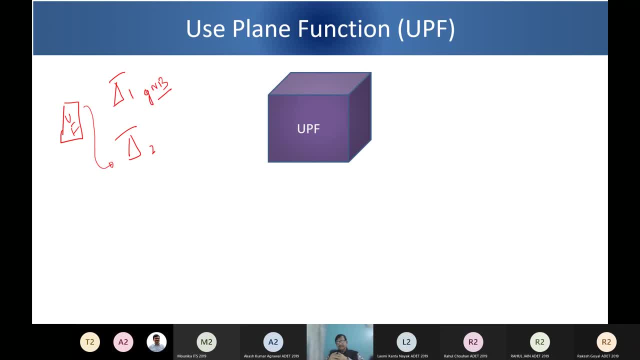 is still common: upf, yes, upf, yes, yes, yes. so what does it mean? it means that the upf acts as a anchor point during ng ran mobility. when there is a mobility from one g node b to other g node b, your epf remains same and that is called anchor point for ng ran. 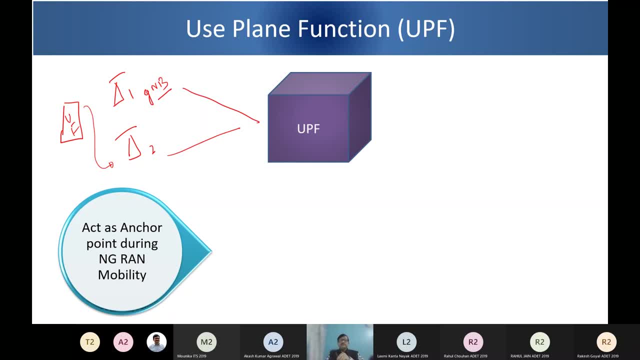 mobility. is this clear? yes, yes, okay, fine now we discussed that, since pdu session is created onto the user plane and epf is sitting in the user plane, so it has to ensure the quality of service which it has got instruction from smf, this is also no issue. 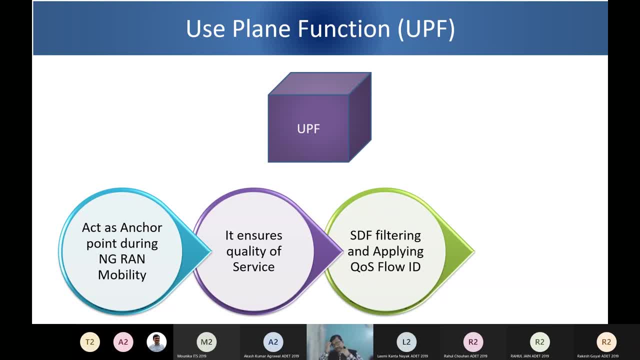 and earlier, while discussing smf, we said that the traffic filtering has to be done. so we call it sdf service: data flow filtering and applying a qs flow id. so when downlink traffic as so this is your data network or any service. so all those ip flows are coming here to the upf. 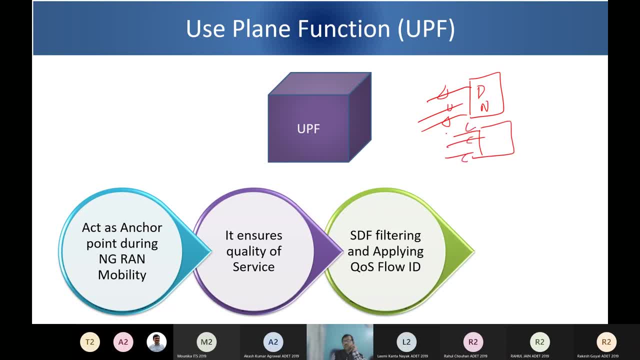 from one data network, it may be from other data network or from another data network or from another data network and so on. so how to identify and apply quality of service. because upf has got filters from smf, it applies those filters and segregate these ips flows into different qs flow id, qfi: it applies a qfi id. 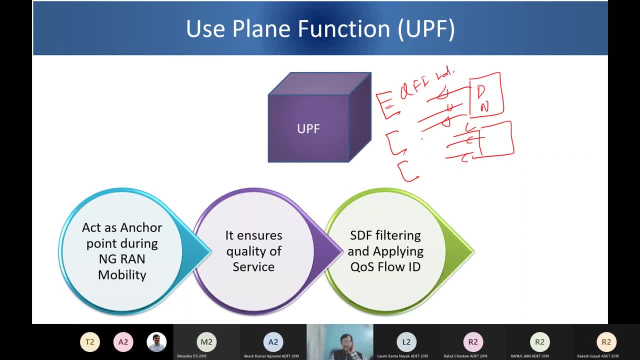 right and and pass on the traffic to that particular qs flow. so sdf filtering and applying qs flow. the next function is, of course, packet routing and forwarding, because it is connected to the data network on one side and g node b to other side. so all those packet forwarding and routing is done. 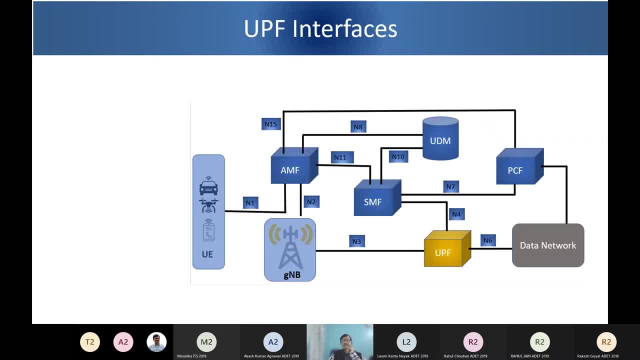 here at upf. what are the interfaces of upf? so: n3 interface with g node b, that here the tunnel is created. n3 interface with g node b, that here the tunnel is created. n3 interface with g node b. n6 interface with data network. n4 interface with smf. so three interfaces. there is one more. 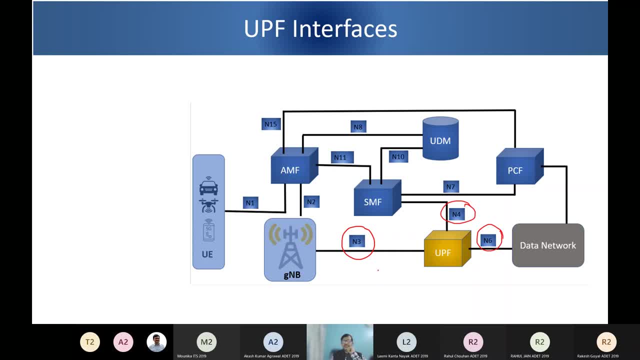 interface which is not written here is like: suppose there are more than one upf, as i said, there can be even intermediate upf. suppose traffic is coming here and then it is, it is going. so basically the interface between two upf is called n9. please remember this, it is n9. 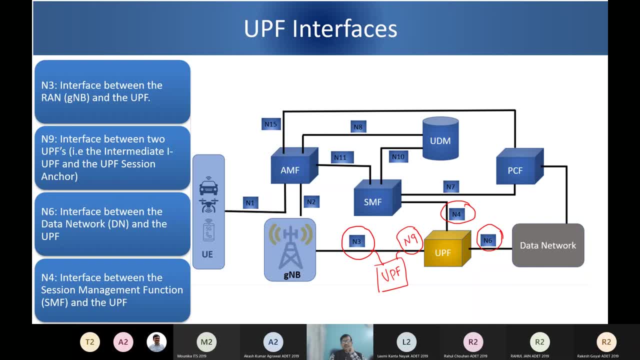 okay, okay now, uh, let us, yeah, please go ahead. so why no interface is shown between u and g node v, ue? this is an air interface, okay, okay, actually n1 is also going through this, although it is shown here transparent. g node b is kind of transparent. so actual connection of the ue. 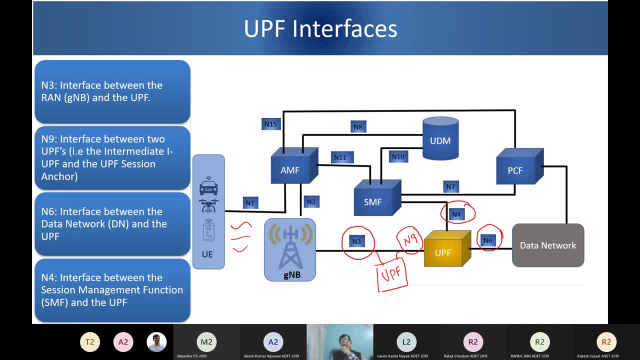 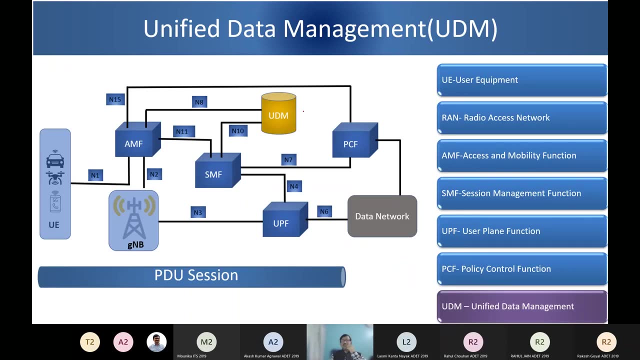 transparent. So actual connection of the UV is through gene node B wherever it goes, whether it is a user plane or control plane, but the I mean the connection is directly to the MFR core part, Now the UDM, Unified Data Management. So let us look at what it is. 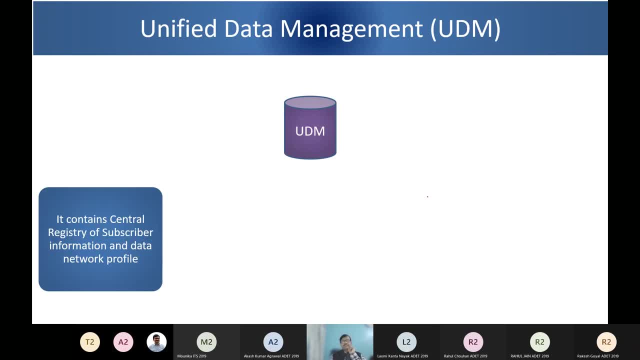 First, it contains registry of subscriber information and data network profile. So just like your HLR or HSS earlier, right. So why data network profile? Because multiple data network will be connected for different services and which user can access to which data network profile. that table would be there in the UDM. Next is the UDM is involved in the. 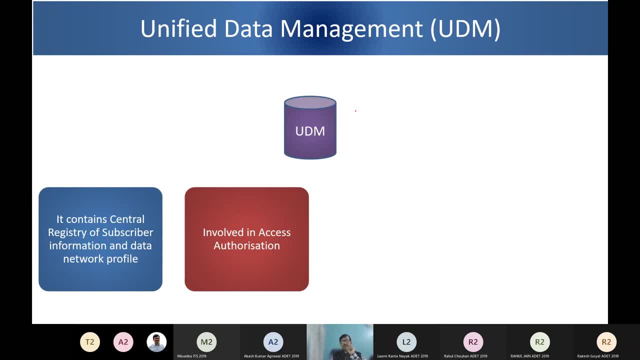 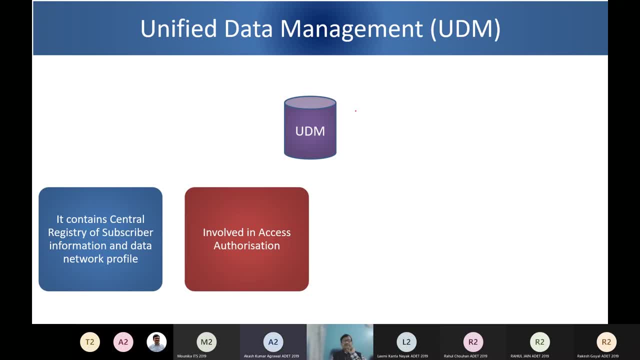 Akash, Whether the particular subscriber is authorized to access the network or not. Yeah, so subscriber profile it has, which it gives to AMF or SMF, as the case may be right. So basically, two things I want to explain here. One is that 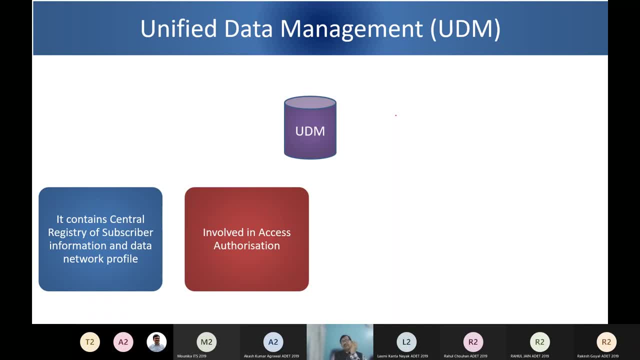 Akash talked about various keys which a SIM is having and the same key will be there with the UDM. So all those keys for authentication, Security keys or whatever keys for authentication purpose. number one: Secondly, when user equipment is sending its concealed ID, it can be decrypted. 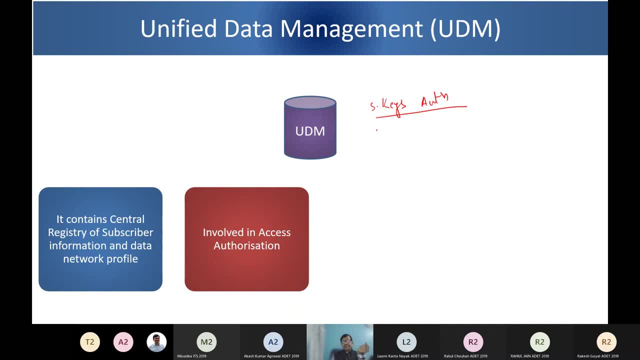 by the UDM itself. So the corresponding private key is also with the UDM. So all those security key, you can say So, all those security key, you can say So, all those security key, you can say Key is also with UDM right BLACK Number. 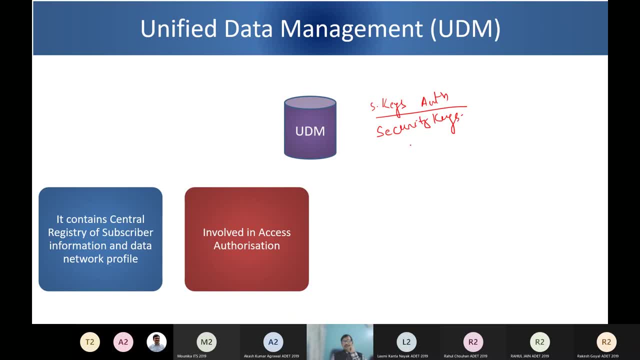 hunter owns is not included in number one�. In fact, UDM knows that which AMF is actually handling a particular UE because AMF has to contact UDM at the time of authentication. So UDM knows that which AMF is actually handling a particular UE at that point of time. 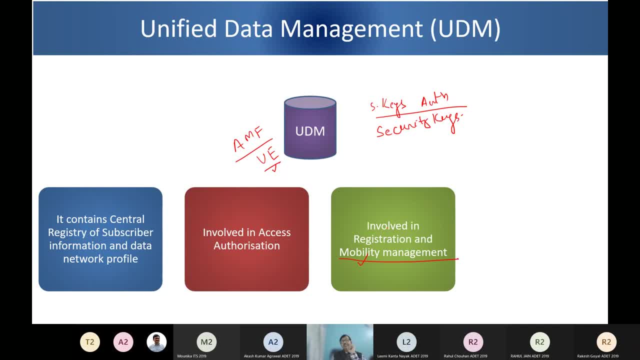 So that's why it plays a role in mobility management, inter-AMF mobility management. it plays a role And then of course it tells AMF and SMS that what is allowed or not allowed, which QoS profile or data network a UE can connect or not connect, because it has got all the profile. 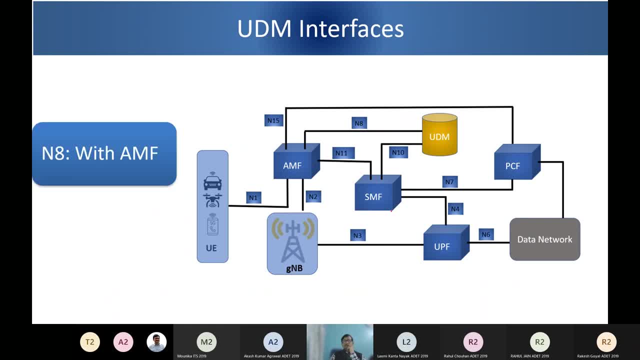 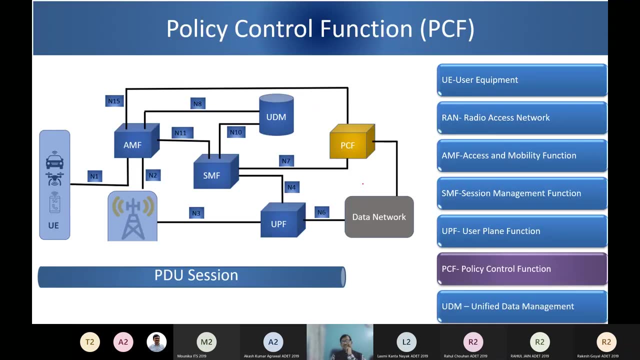 What are the interfaces? Very simple: ANET with AMF, ANTEN with SMF, because these are the network function which uses the UDM services. This is the last network function, which is which we are doing in part, one which is the 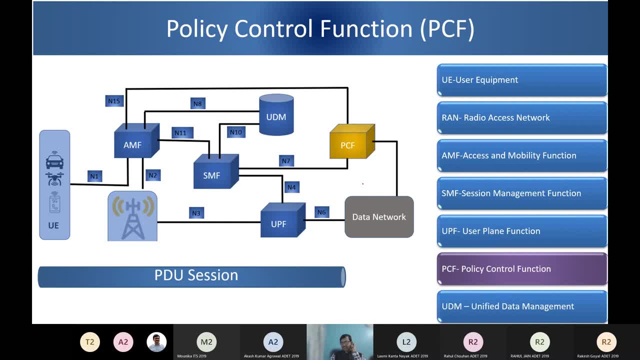 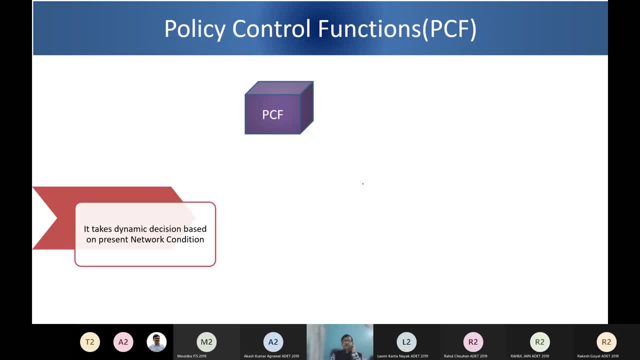 policy control function. So we have discussed a bit about it that all policy related decisions are taken by PCF. So one of the function is that it takes dynamic decision based on present network conditions. That means if a particular time, if a subscriber is in area where, say, no cell is there or or 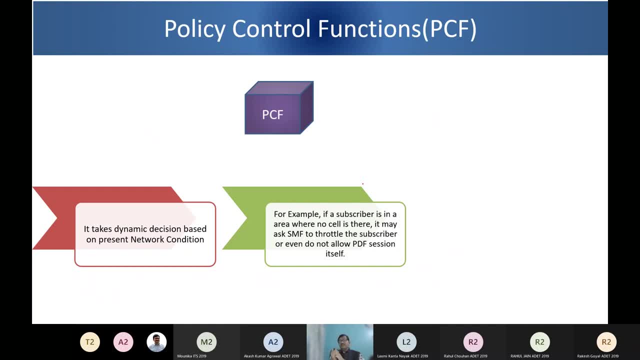 poor coverage is there, it may ask SMF to throttle the customer. that means reduce the data rate or even do not allow the PDU session itself right. So it takes a dynamic decision. also, in addition to the we talked about, it provides PCC rule. 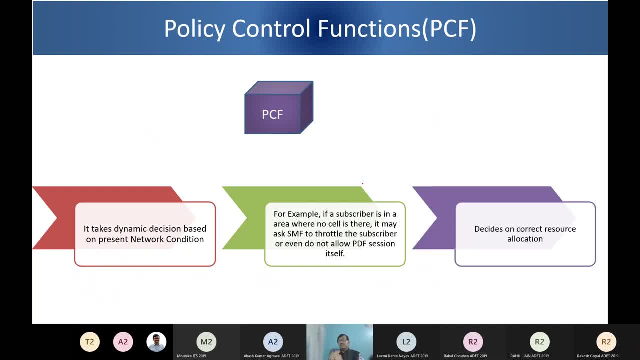 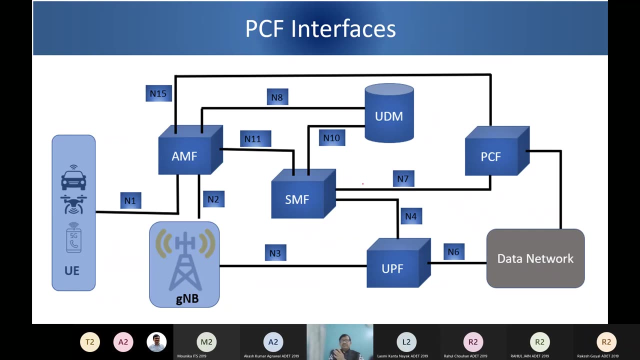 to SMF. It also takes dynamic decision and also decides on the correct resource allocation, because all those policy related decisions are taken by PCF in the network. What are the PCF interfaces? That is, N7 with SMF and N15 with AMF. 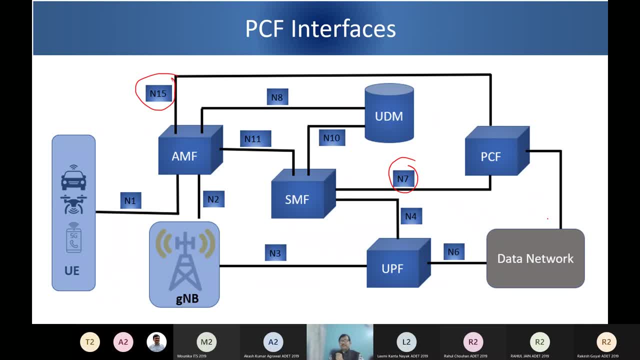 So SMF and AMF. I also see a connection with data network. Can somebody guess what it is for? Can you guess why this is connected to data network? PCF To Sir, To Sir Sir, because as soon as his data limited out we can start to use this. 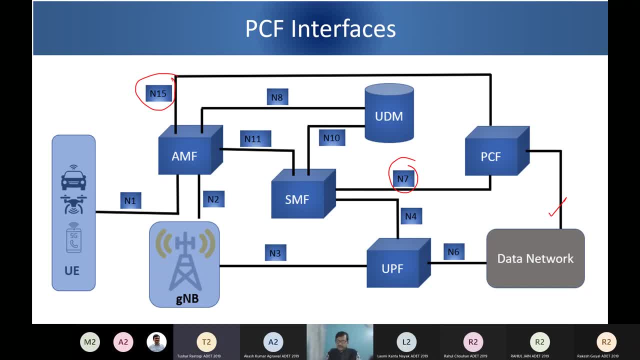 So so stop that pda session, whether he has. yeah. so basically, as i said, this data network is is not a single data network, but it can be various service, maybe ar vr service or gaming service or any kind of service, right? so what happens? let me explain a bit that. whenever suppose, 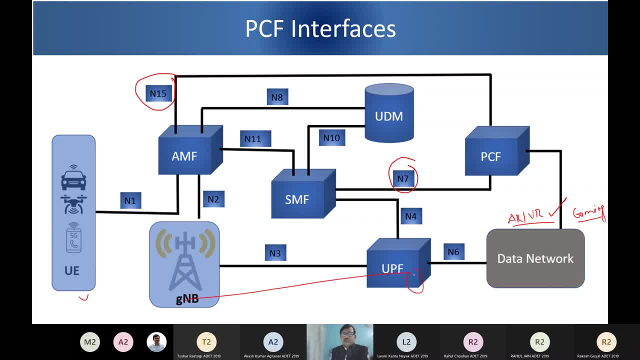 user is on to the network and you have created a pdu session right and within the pdu session you have a default qs flow created right. so using this default qs flow, the user equipment suppose is trying to access ar vr right and then ar vr knows that this, this particular server knows that.